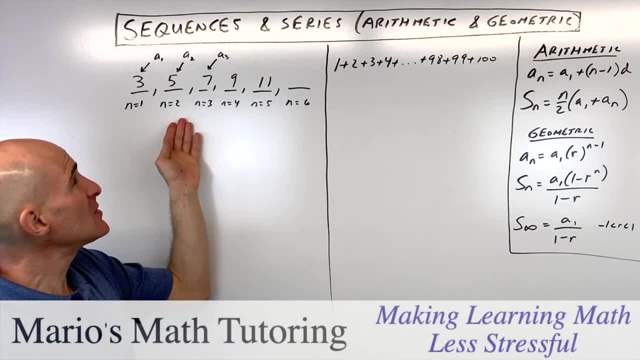 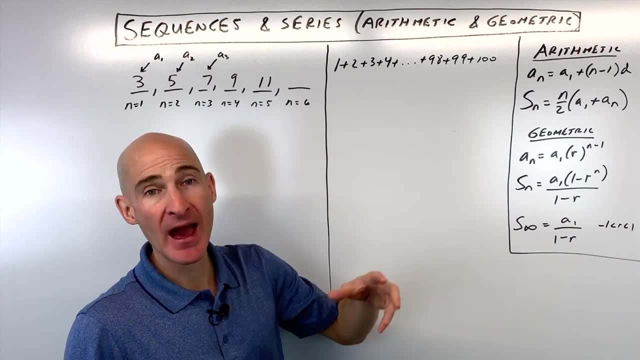 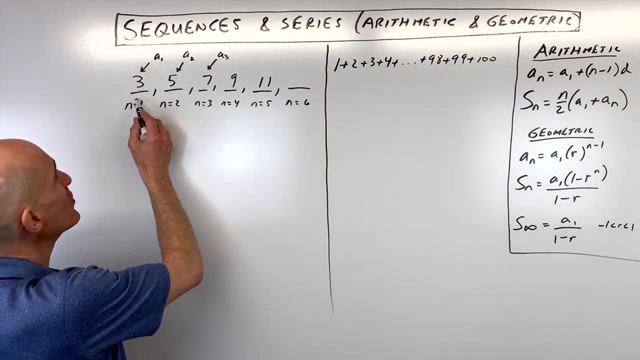 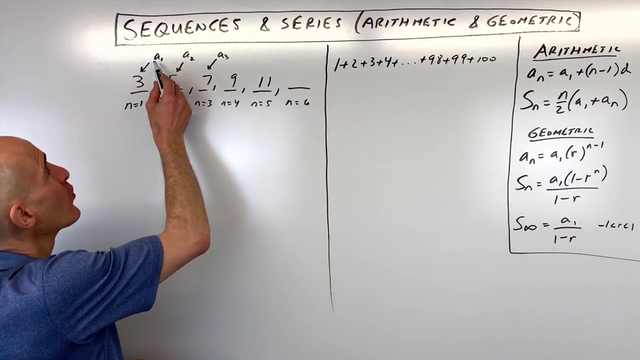 What's the difference between a sequence and a series? Well, a sequence is a list, and a list is separated by commas, Whereas a series is a sum. You're adding up all the terms in that series, That's, you're adding them, So sum. But first let's talk about the notation. So each one of these terms you could call n equals one, n equals two, n equals three, n equals four, etc. That tells you what term that you're on, Whereas a sub one, sub, means, like subscript, a sub two, a sub three. that tells you the. 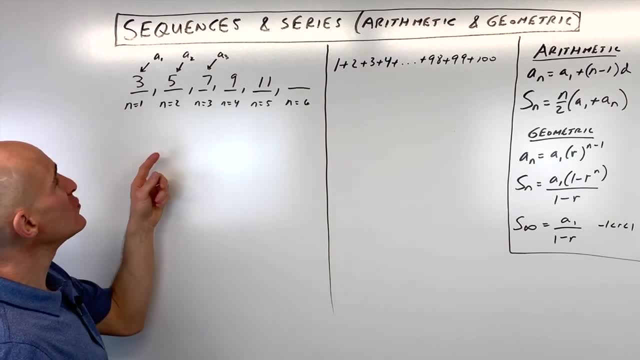 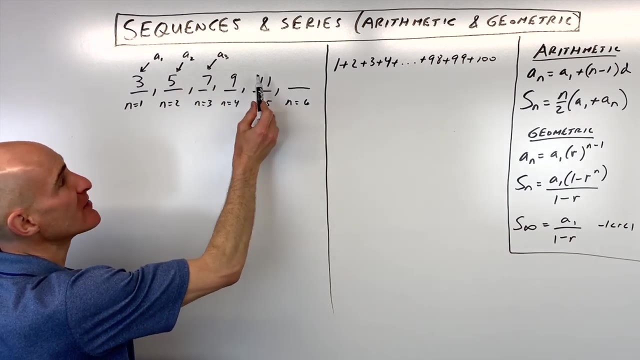 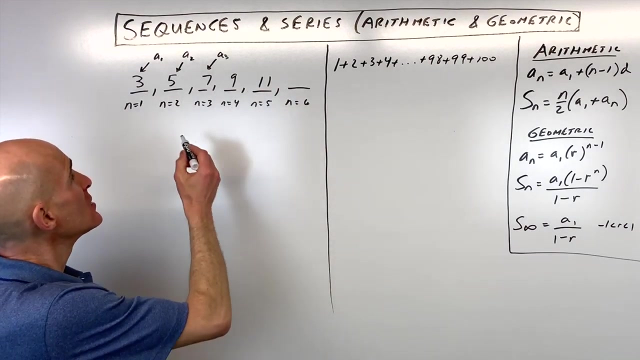 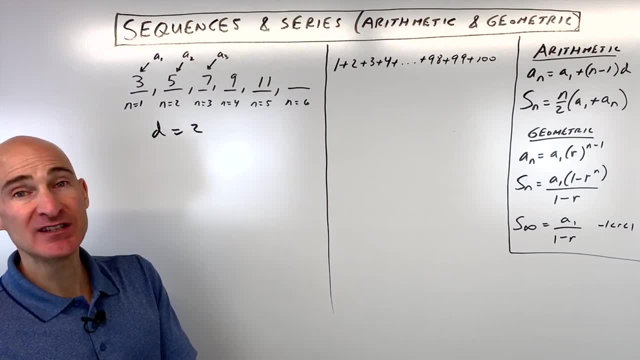 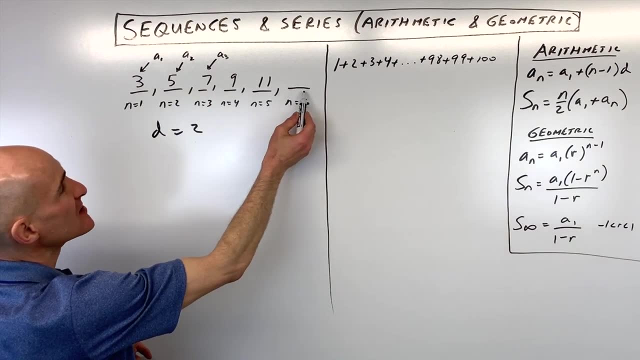 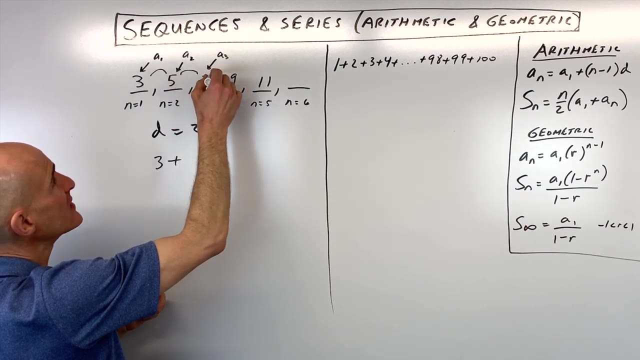 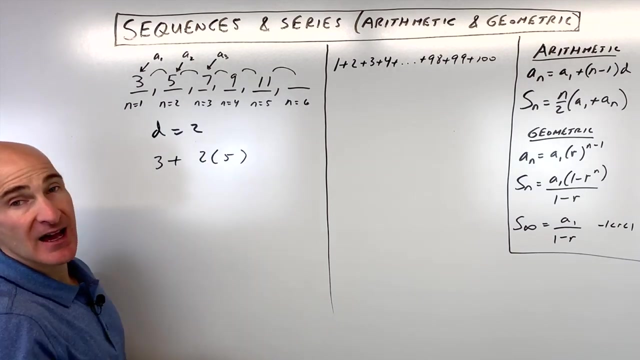 call that d equals two. That's the common difference. So d for difference, like if you subtract five minus three, you get two. seven minus five, you get two. But say we wanted to find out what this sixth term is. What we would do is we would start at three and we would add two once, twice, three times, four times, five times. So why do we add two, five times? How come not six? Well, because we were already at the first term three. 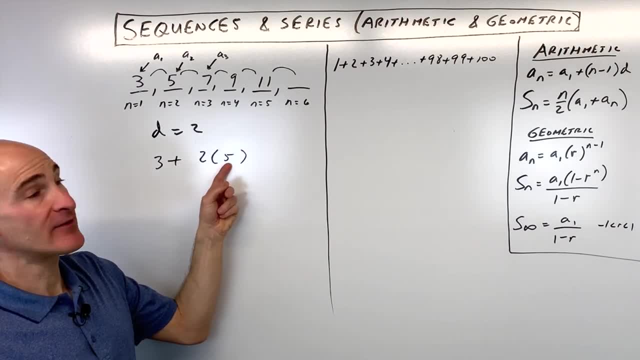 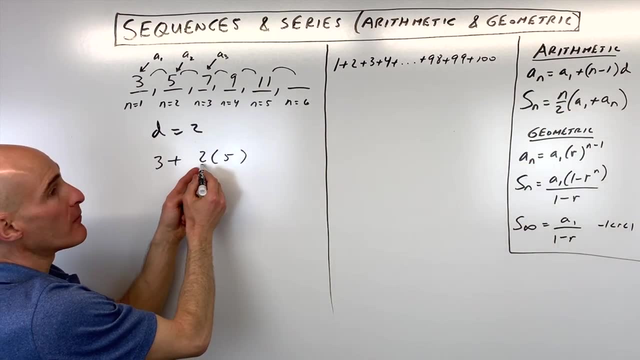 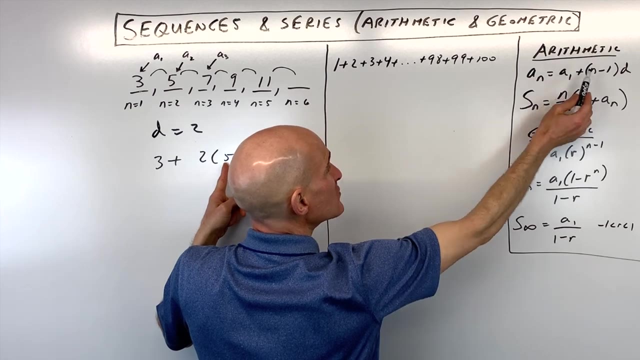 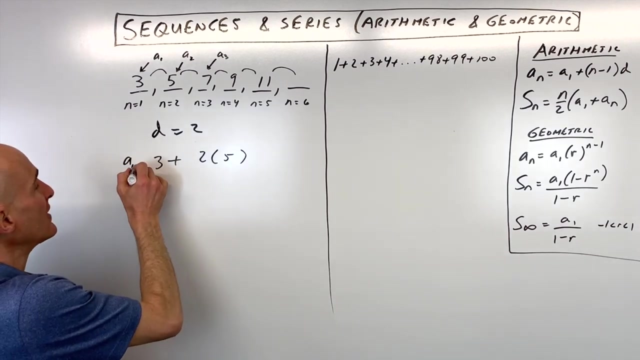 okay, so we only had to add that difference not six times but five times, And that's where our formula comes from here for arithmetic sequences You take the first term, a sub one, plus the common difference- okay here d, which is two times n minus one, and is whatever term you want. So in this case we want to term six, that's six minus one, which is five, And you got it. So this would be a sub six equals 10 plus three, which is 13,. which we? we knew that, but say you wanted to find like a term that was maybe a. 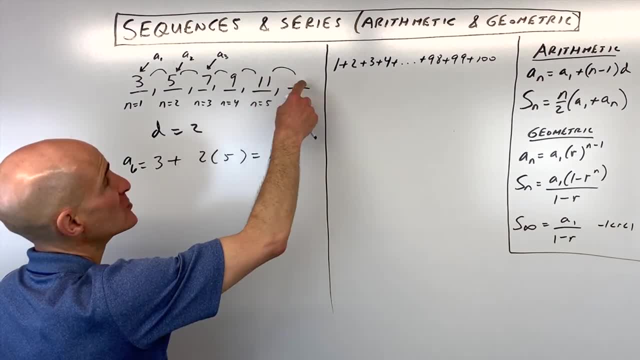 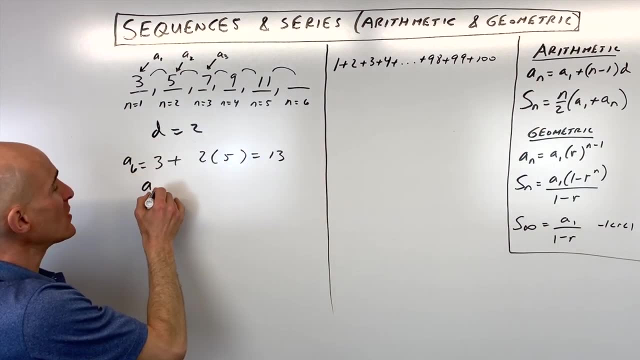 like the 20th term. Well, instead of having to add two, add two, add two until you got to the 20th term, we could write a formula or a rule to find that. So let's go ahead and do that. So a sub n. 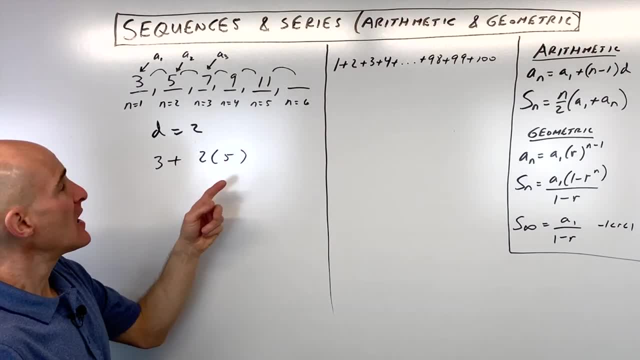 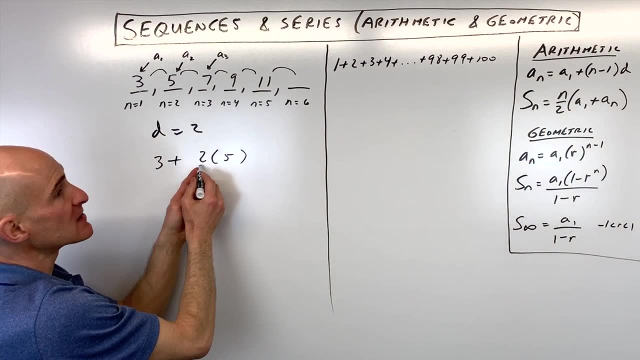 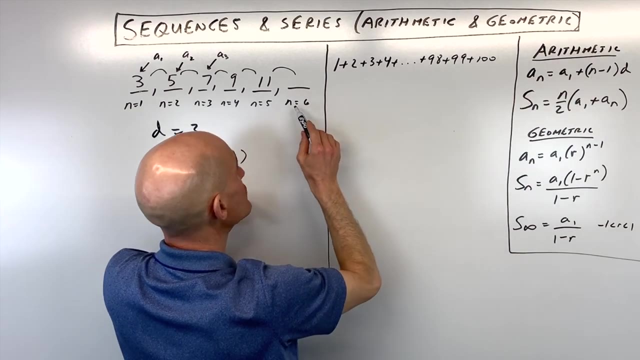 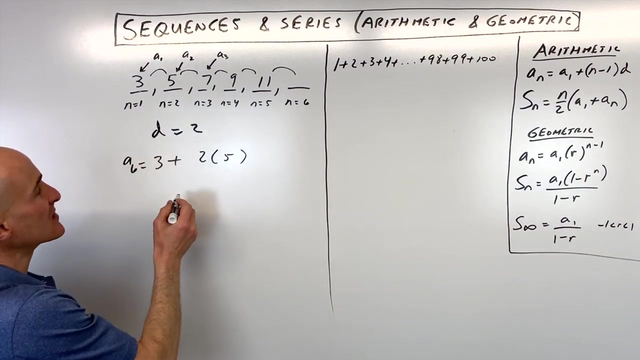 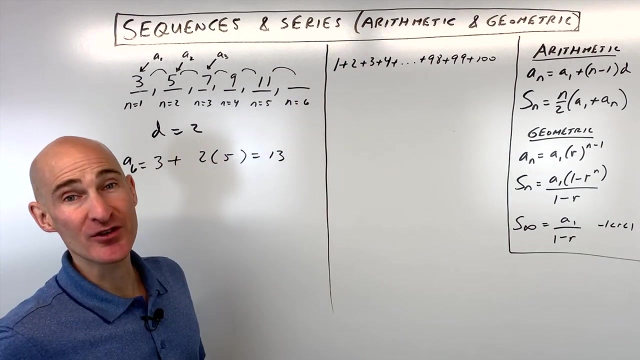 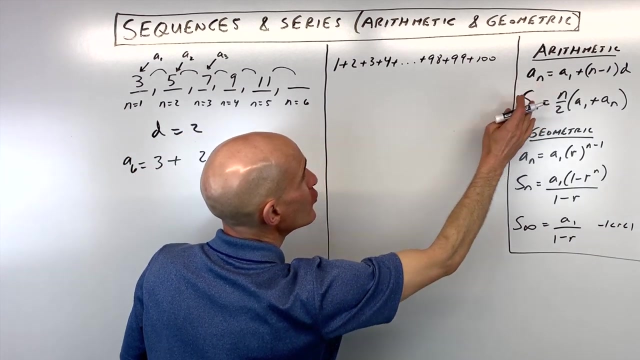 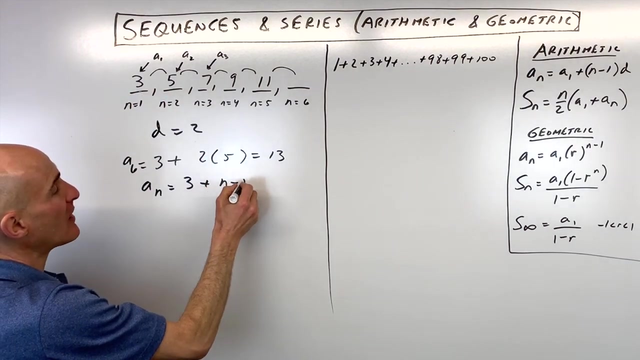 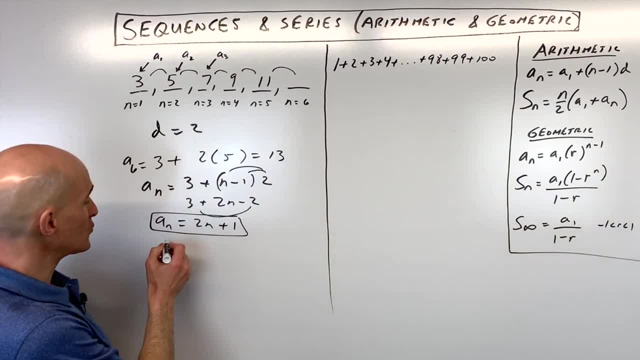 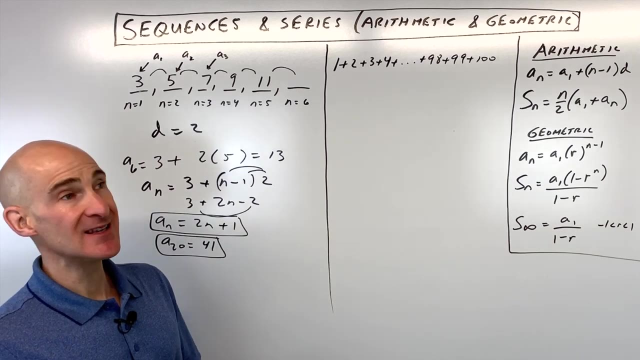 formula or a rule for finding any term. If we want to find that 20th term, we're just going to put in 20. Two times 20 is 40, plus one is 41, and it takes you right to that term. Now another way to write these rules is instead of writing an explicit formula, a formula that takes you right to that particular term, you can write what's called a recursive formula. 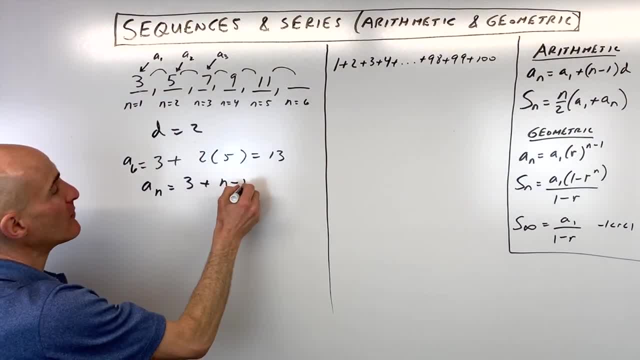 equals a sub one, which is three plus n minus one times d. D is our common difference. Let's go ahead and simplify this by distributing the two, So we get 2n minus two plus three, and let's combine like terms, So 2n plus one, because negative two plus three, and so now we have a. 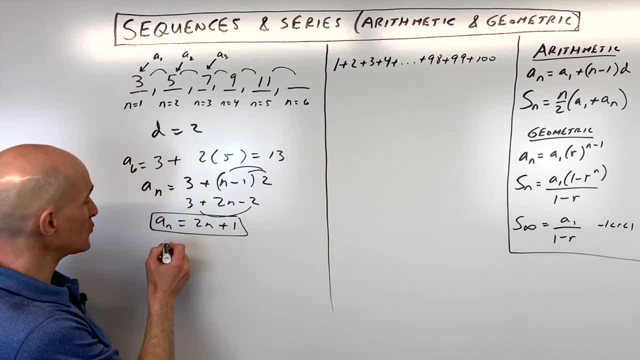 formula or a rule for finding any term. If we want to find that 20th term, we're just going to put in 20.. Two times 20 is 40, plus one is 41, and it takes you right to that term. Now another way to. 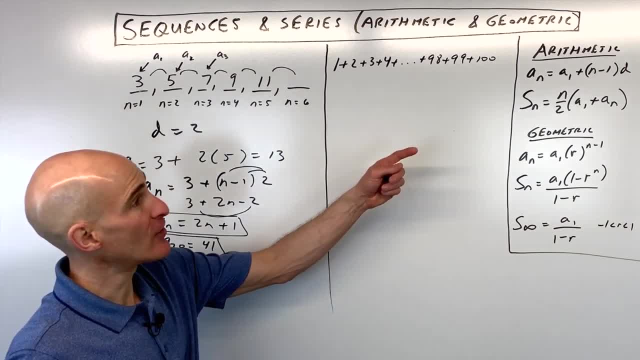 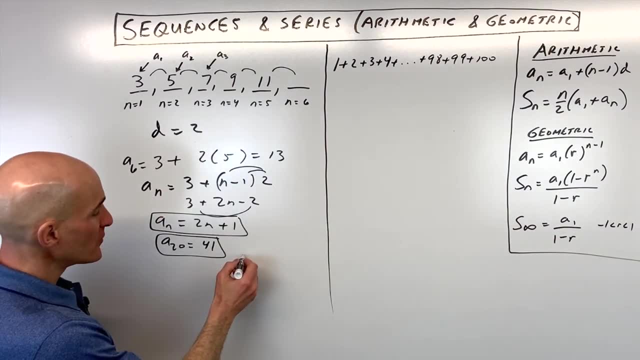 write these rules is, instead of writing an explicit formula, a formula that takes you right to that particular term, you can write what's called a recursive formula, And the recursive formula looks something like this. Let me see if I can show you. You start off with: 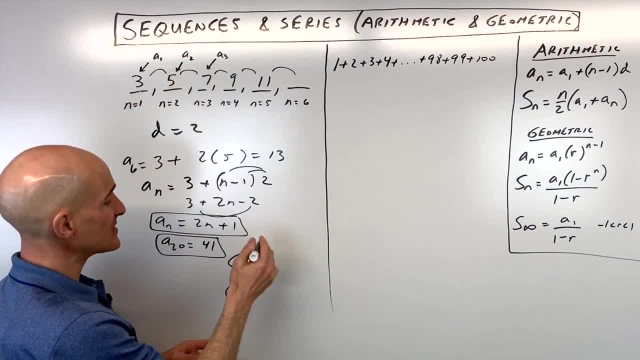 telling the person what's the first term in the sequence. In this case it's three, So a sub one, meaning the value of the first term is three- And then you give them a rule or a formula for finding the next term. Now, there's a couple different ways to do this. One way to do it is to refer to the 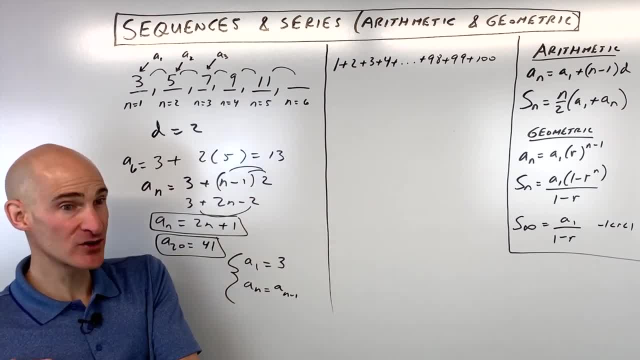 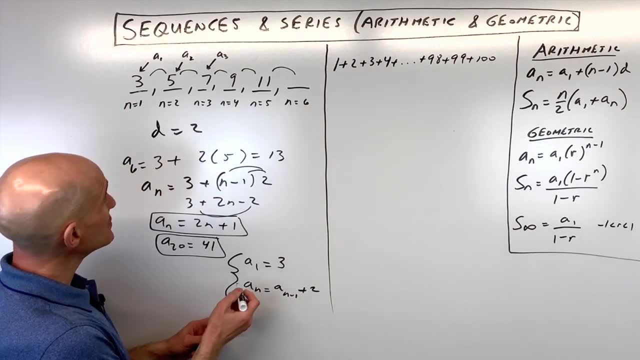 previous term. So a sub n minus one. that means one term before the term that you're on that term that you want to find, And then we're just going to add the rule: So a sub n minus one, which is a 2.. So, for example, if we want to find the sixth term, a sub 6, we would go to the 6 minus 1, which 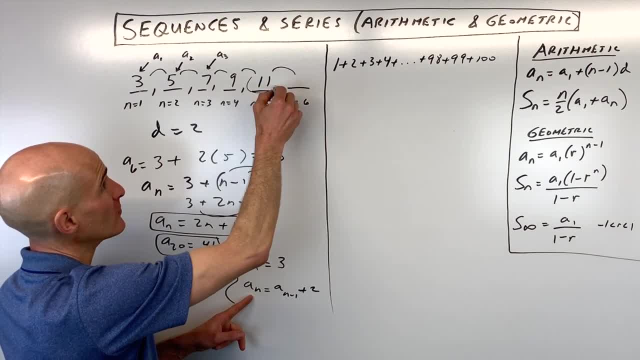 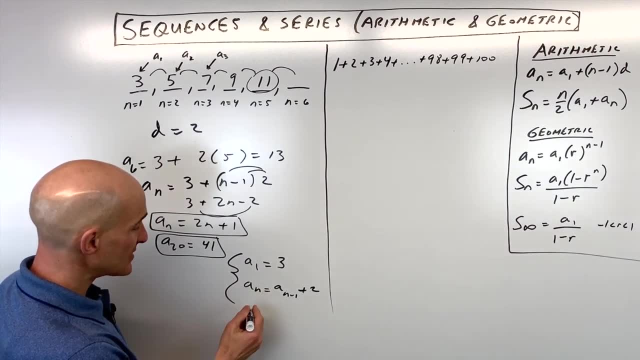 is the a sub 5 term here, the value of the fifth term, and we would just add 2 and we got it. Now, the other way I was telling you that you could write this is, instead of saying a sub n, you could say a sub n plus 1. so that means you want to go to the, the next term, the one after the nth term. 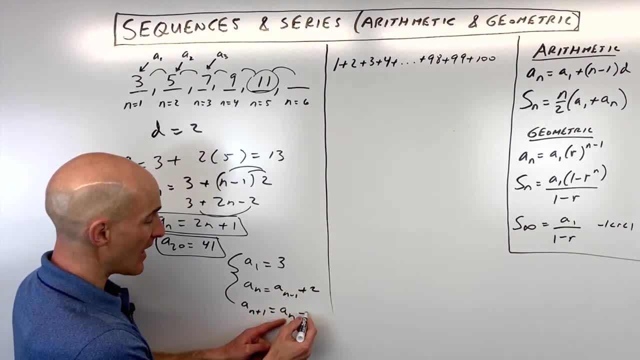 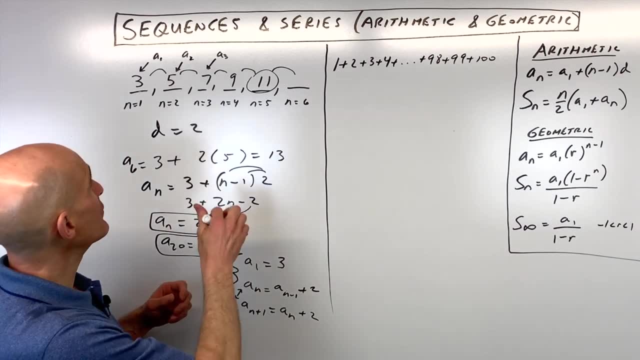 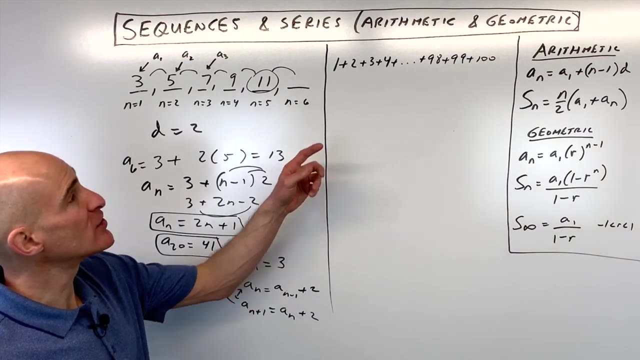 and so then you would take a sub n- that's the value of the term that you're on- and you would add 2.. Either one of these is a fine, whichever one you prefer. Now say, for example, you wanted to add up all these terms, let's say up to the 20th term. how would you do that? Well, let me illustrate. 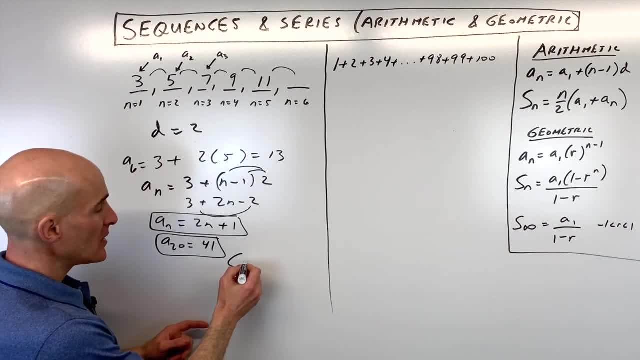 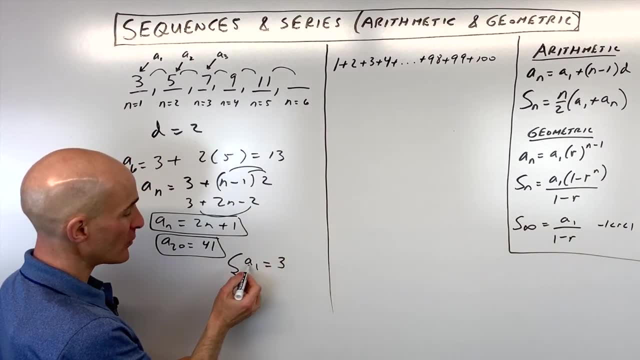 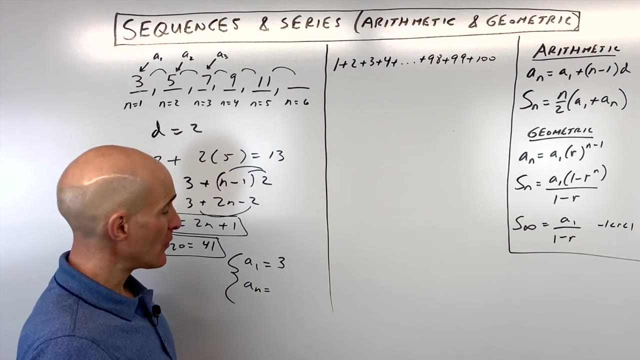 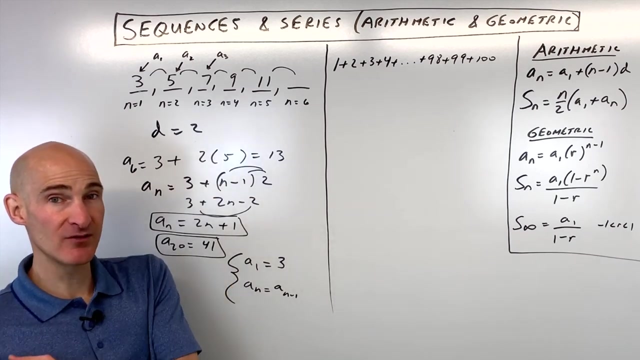 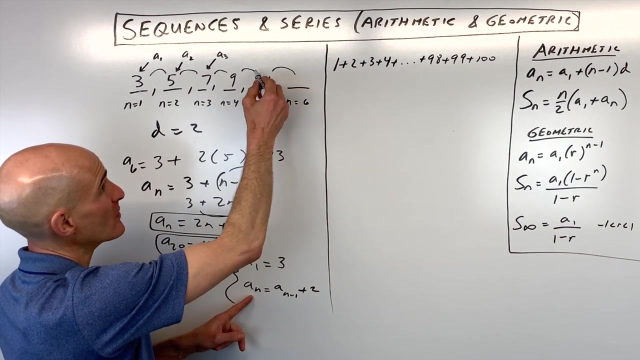 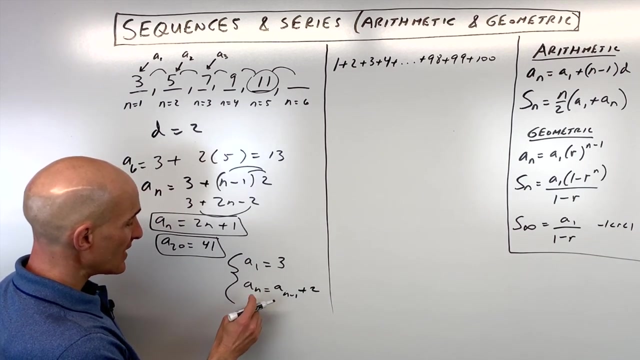 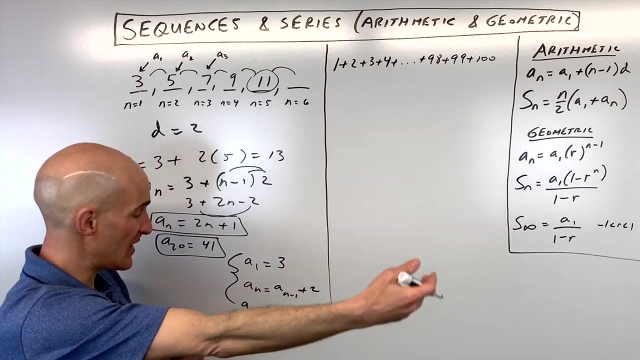 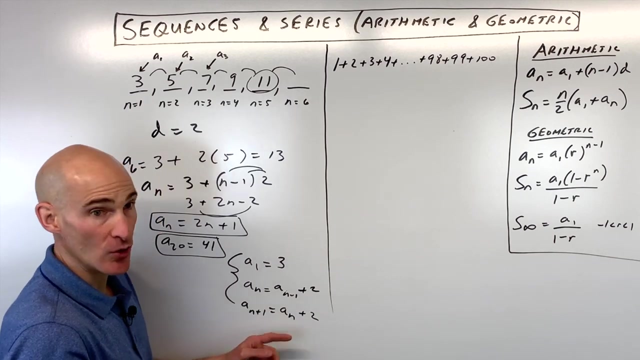 And the recursive formula looks something like this. Let me see if I can show you. You start off with telling the person what's the first term in the sequence. In this case it's three, so a sub one, meaning the value of the first term is three, and then you give them a rule or a formula for finding the next term. Now there's a couple different ways to do this. One way to do it is to refer to the previous term, so a sub n minus one. That means one term before the term that you're on, that term that you want to find. And then we're just going to add two. So for example, if we want to find the sixth term, a sub six, we would go to the six minus one, which is the a sub five term here, the value of the fifth term, and we would just add two, and we got it. Now the other way I was telling you that you could write this is instead of saying a sub n, you could say a sub n plus one. So that means you want to go to the next term, the one after the nth term. And so then you would take a sub n, that's the value of the term that you're on, and you would add two. 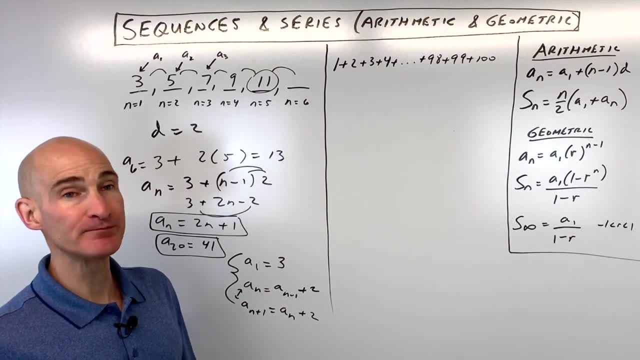 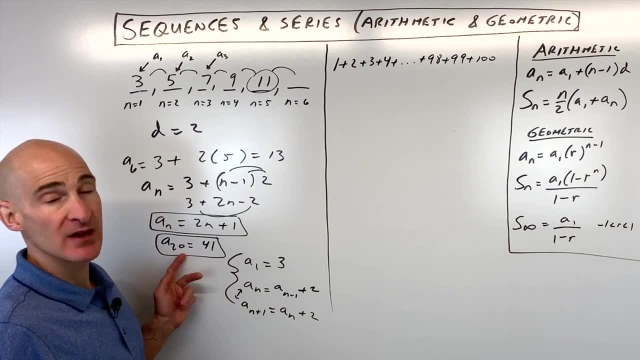 Either one of these is fine, whichever one you prefer. Now say, for example, you wanted to add up all these terms, let's say up to the 20th term. How would you do that? Well, let me illustrate here. 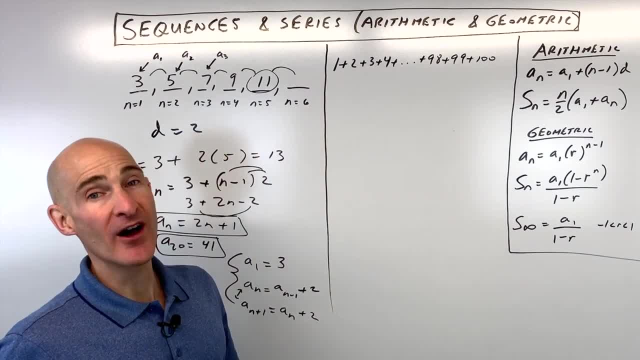 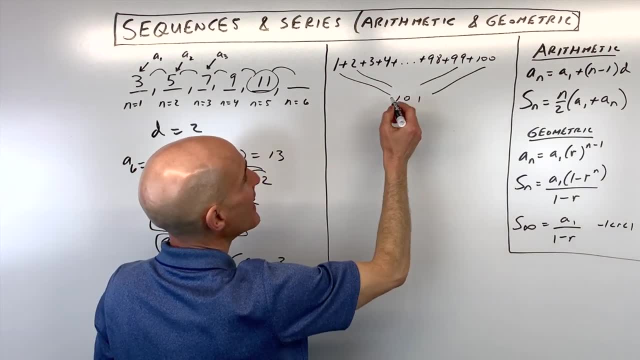 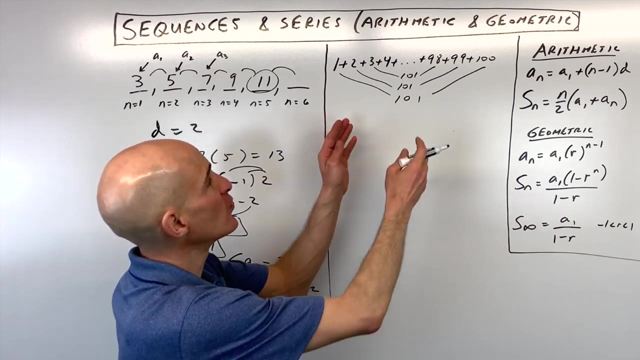 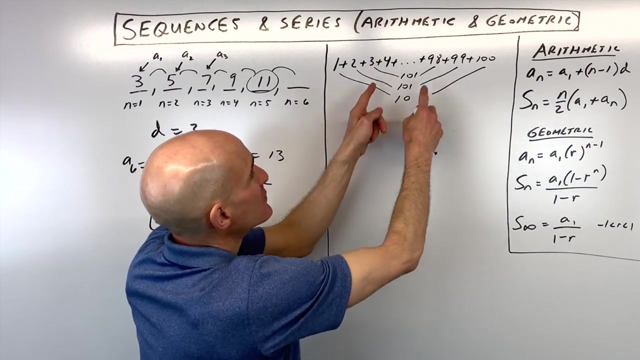 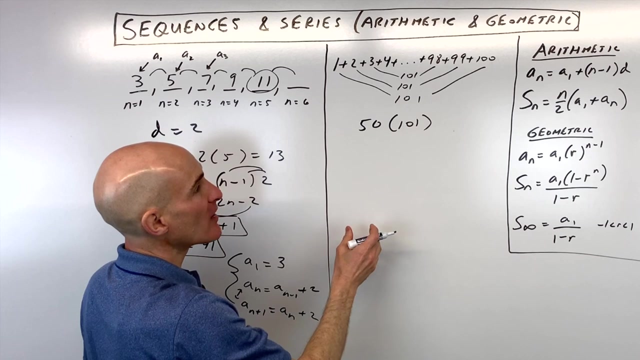 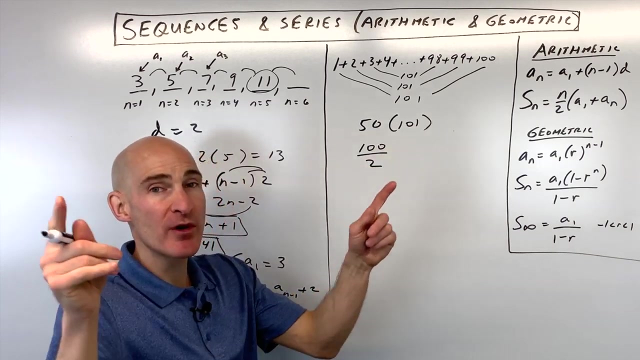 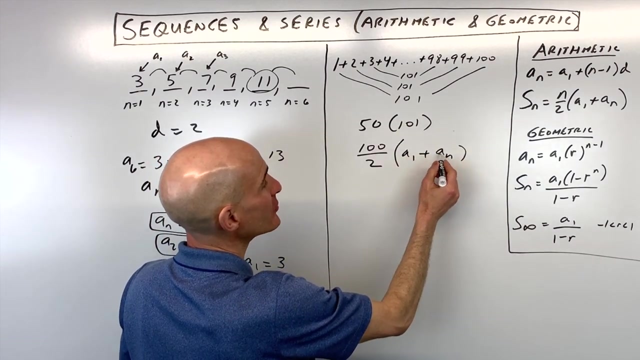 Say you wanted to add all the numbers from one to a hundred. Well, that would take you a while, right? But look at this pattern. So if you take one plus a hundred, you get a hundred and one. Two plus ninety-nine, you get a hundred and one. Three plus ninety-eight, you get a hundred and one. How many hundred and one do you get? You get a hundred and one. How many hundred and ones do you think that we could make, you know, by adding the numbers from one to a hundred? Well, if you said fifty, you're right, because you're pairing them up two at a time, right? So what we have here is we have, there's fifty one hundred and ones. So if we generalize now and write this as a formula, what we did is we took the number of terms, which was one hundred, divided by two, because we're pairing them up two at a time, and then what we did is we took the first term, a sub one, which is one, plus the nth term, okay? 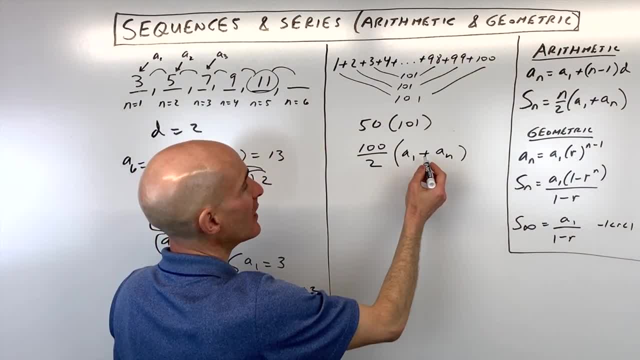 The last term, which is a hundred, and that's how we got our hundred and one. So that's where this formula is coming from right here. It's the number of terms divided by two, times the sum of the 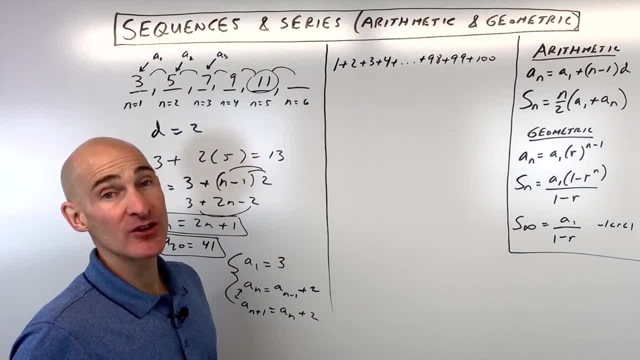 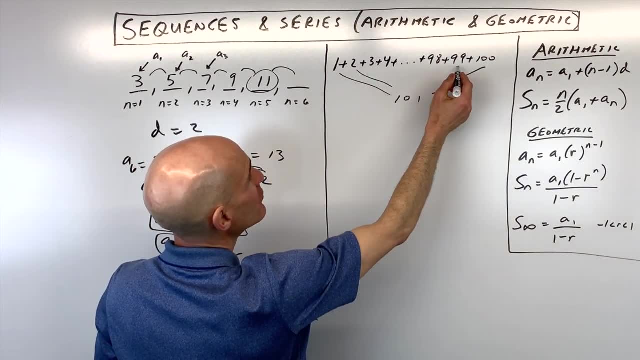 here. say, you wanted to add all the numbers from 1 to 100. well, that would take you a while, right. but look at this pattern. so if you take 1 plus 100, you get 101,. 2 plus 99, you get 101, 3 plus 98. 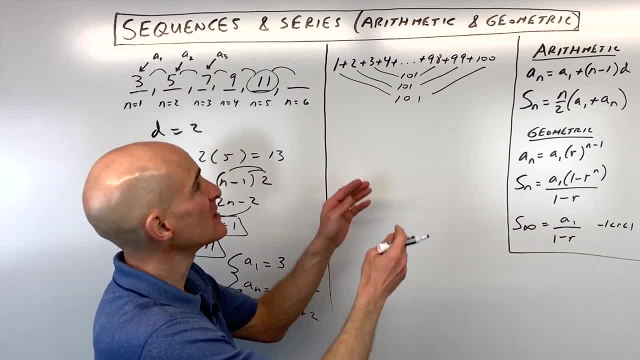 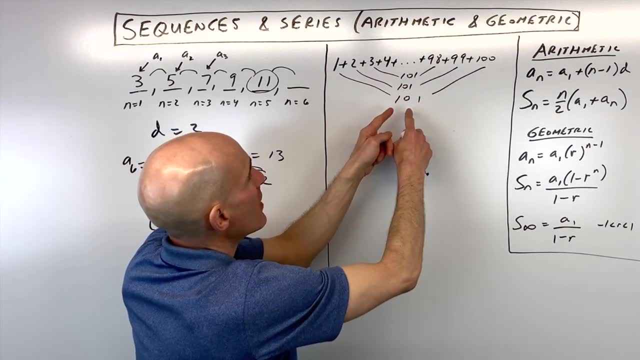 you get 101.. How, How many hundred and ones do you think that we could make you know by adding the numbers from 1 to 100?? Well, if you said 50, you're right, because you're pairing them up two at a time, right? so what? 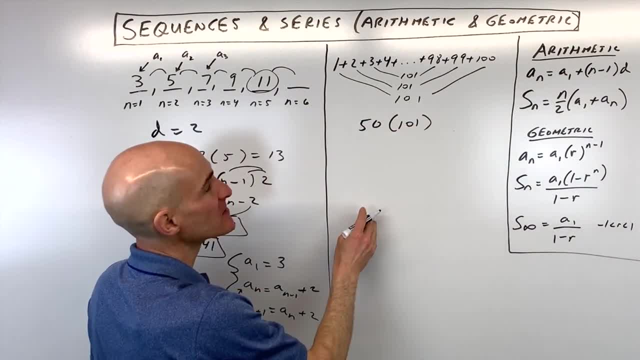 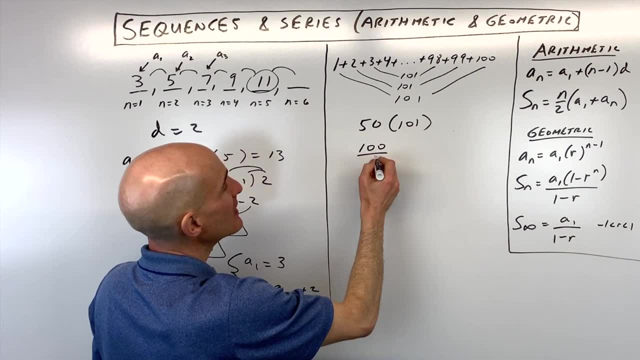 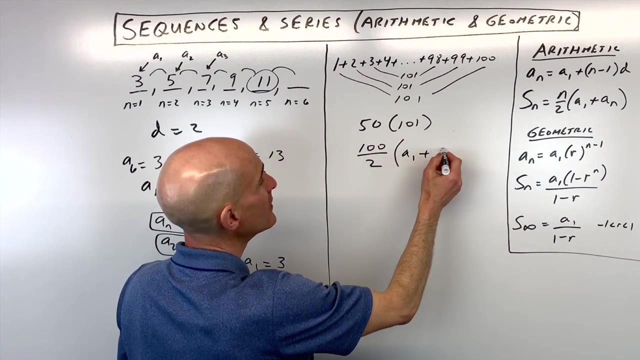 we have here is we have there's 50 101s. so if we generalize now and write this as a formula, what we did is we took the number of terms, which was 100, divided by 2, because we're pairing them up two at a time. and then what we did is we took the first term, a sub 1, which is 1 plus the nth term. 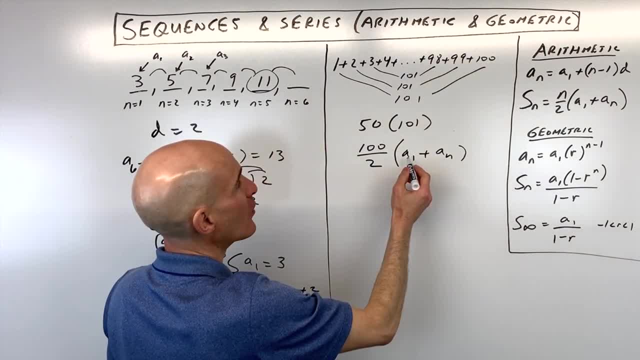 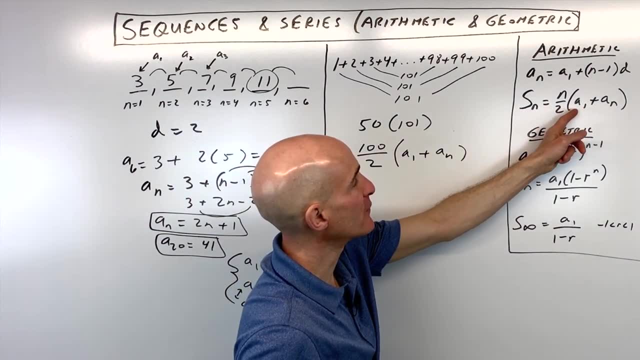 okay, which is the last term, which is 100, and that's how we got our 101. so that's where this formula is coming from. right here, it's the number of terms divided by 2 times the sum of the first term in the last term. okay, a sub n just means the the nth term of the last term. so, going back to 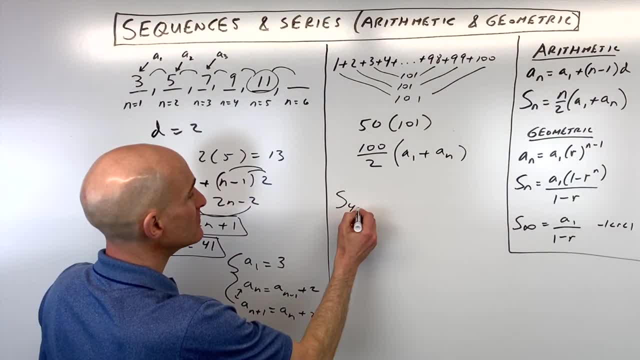 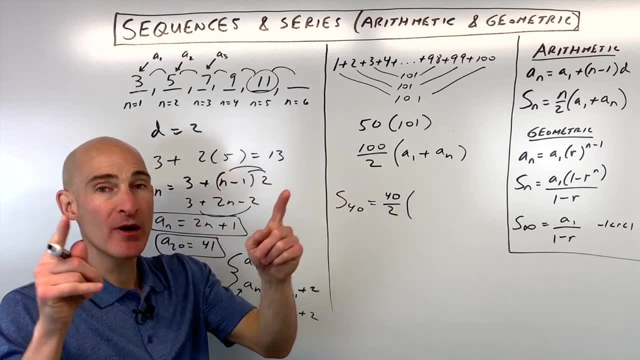 this problem over here. if we wanted to add up the sum of the first 40 terms, okay s sub 40. we know that there's 40 terms. okay, we're dividing that by 2 because we're going to pair them up two at a time. 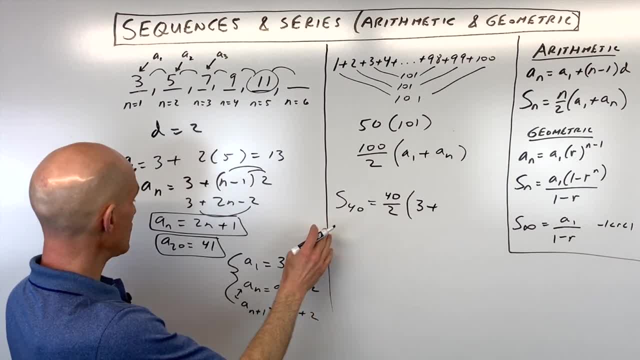 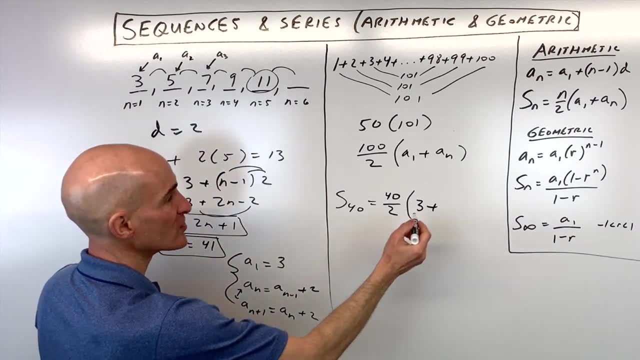 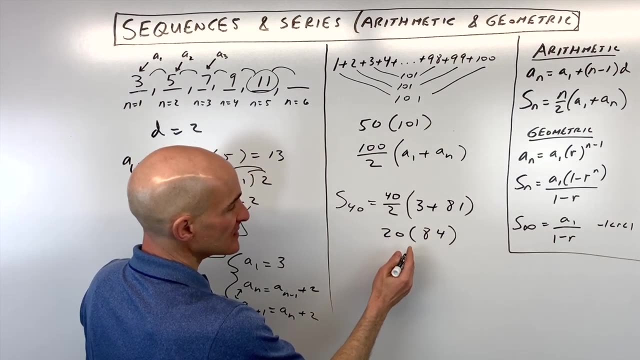 and the first term we said was 3.. And the 40th term. let's see what the 40th term is. We're going to put 40 in for here, So that's 2 times 40, which is 80, plus 1,, which is 81. And so now we have 20 times 84. Let's see. 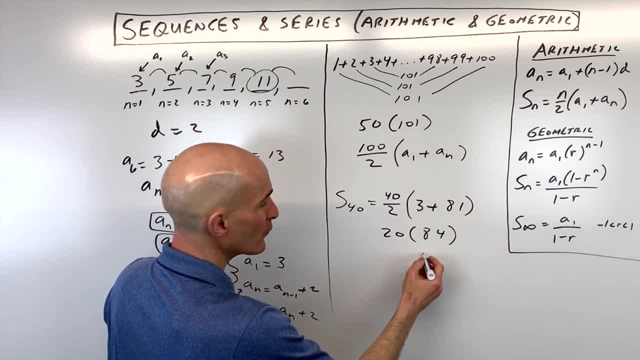 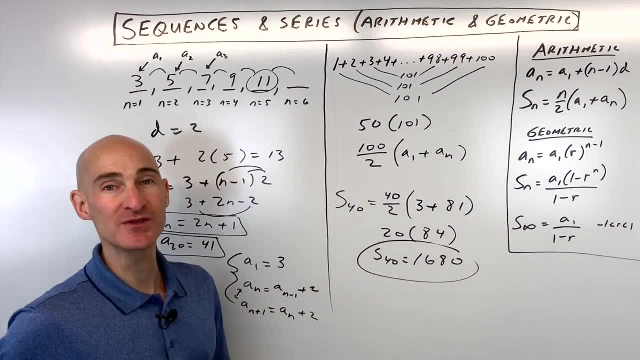 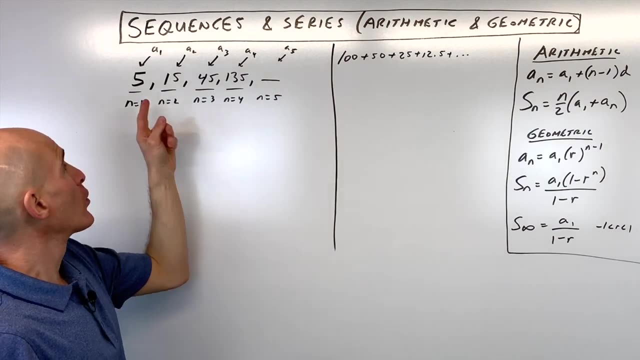 10 times 84 is 840.. So it's 840 doubled, That's 1,680.. And that's the sum of the first 40 terms. Let's take a look at this sequence now. We've got 5,, 15,, 45,, 135,, dot, dot, dot. What are we doing? 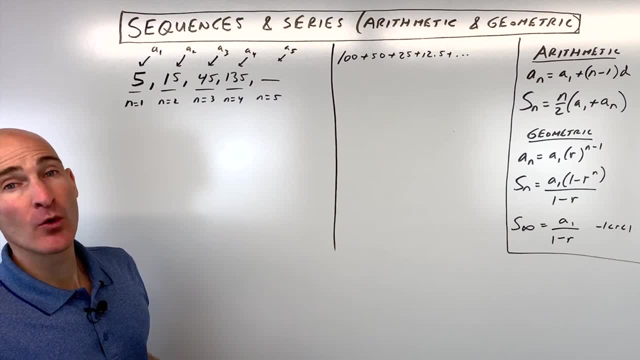 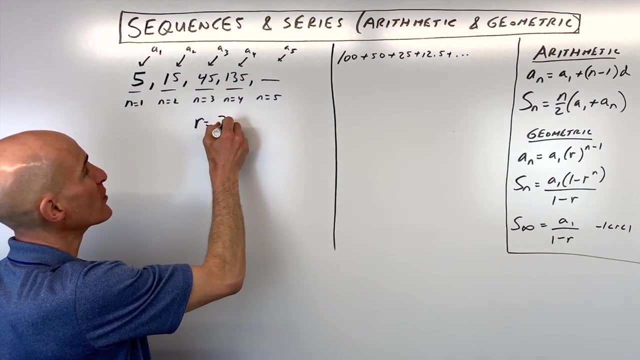 to get from this term to this next term, to the next term, to the next term. Well, here you can see, we're actually multiplying by 3.. And this thing that we're multiplying by each time, this is called the ratio. so r for ratio, And if you're having trouble finding out what that ratio is, 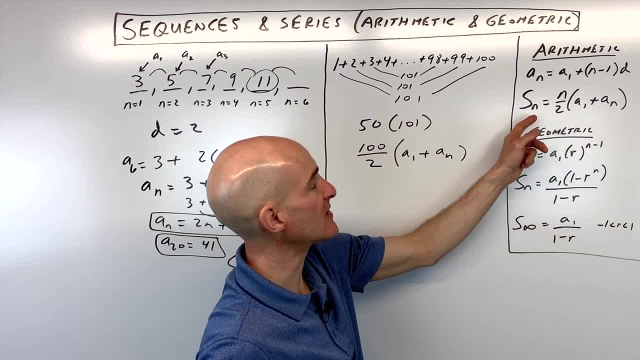 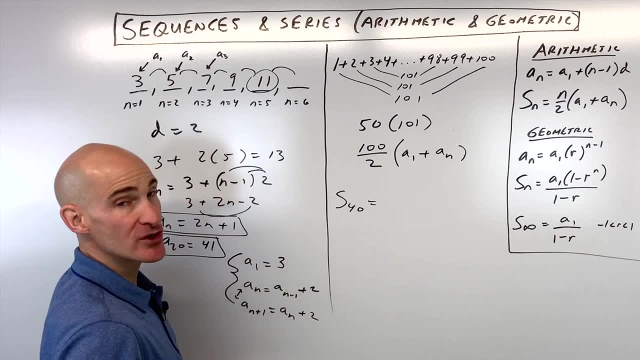 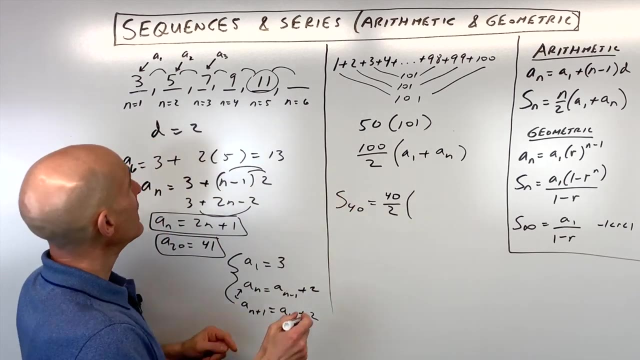 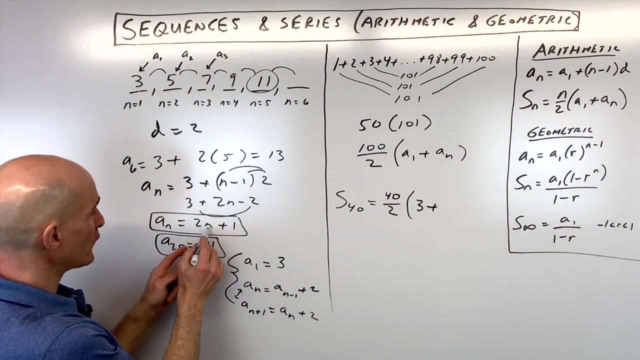 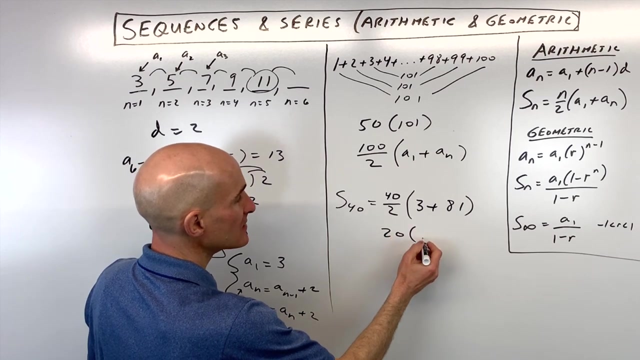 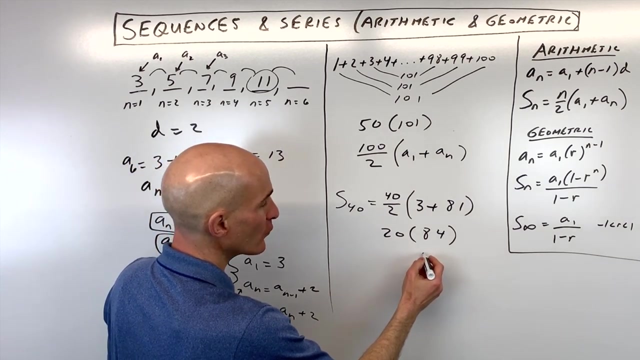 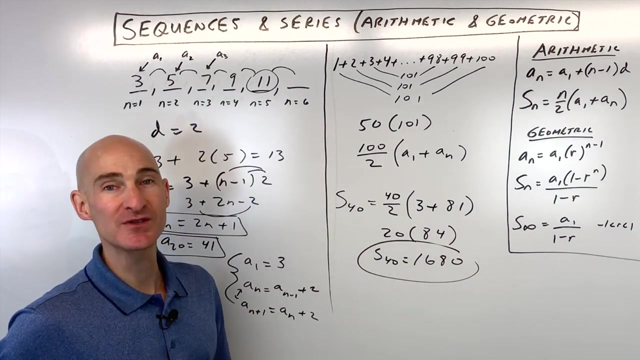 first term and the last term, okay? A sub n just means the nth term or the last term. So going back to this problem over here, if we wanted to add up the sum of the first forty terms, okay, s sub forty, we know that there's forty terms, okay? We're dividing that by two, because we're going to pair them up two at a time, and the first term we said was three. And the fortieth term, let's see what the fortieth term is. We're going to put forty in for here, so that's two times forty, which is eighty plus one, which is eighty one. And so now we have twenty times eighty-four. Let's see, ten times eighty-four is eight hundred and forty, so it's eight hundred and forty doubled, that's one thousand six hundred and eighty, and that's the sum of the first forty terms. 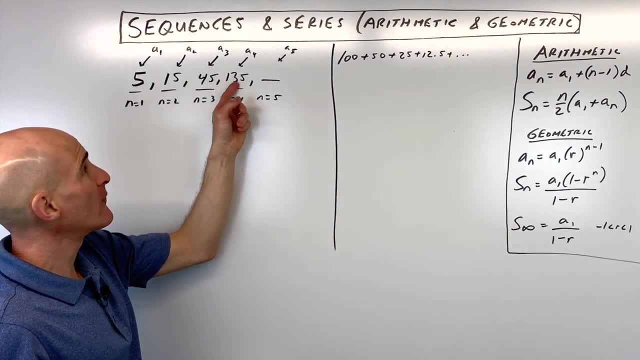 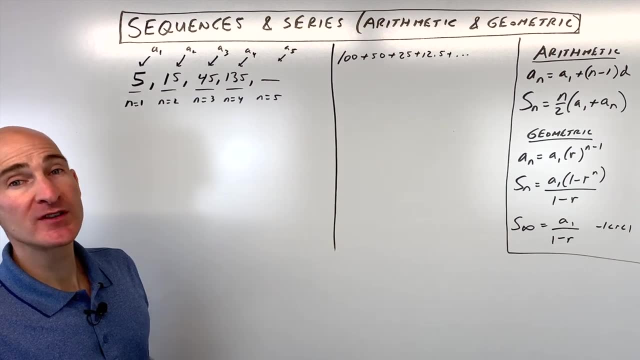 Let's take a look at this sequence now. We've got five, fifteen, forty-five, one What are we doing to get from this term to this next term to the next term to the next term? 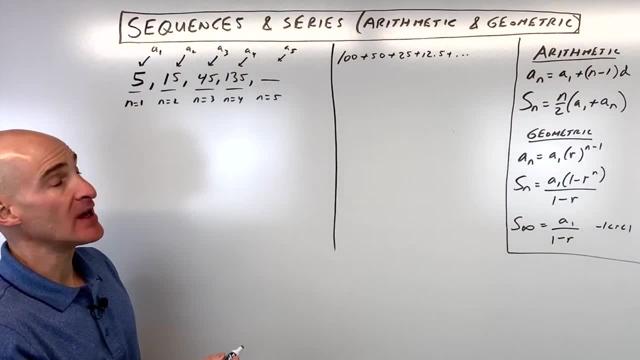 Well here you can see we're actually multiplying by 3. 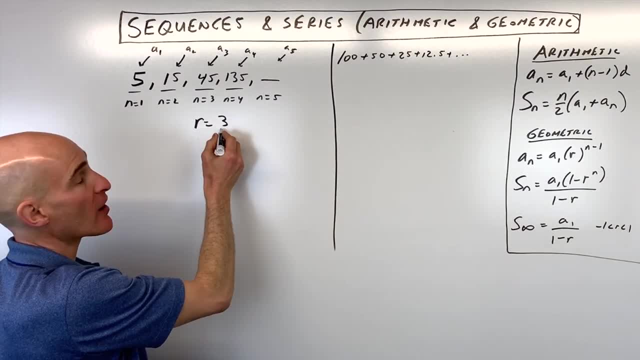 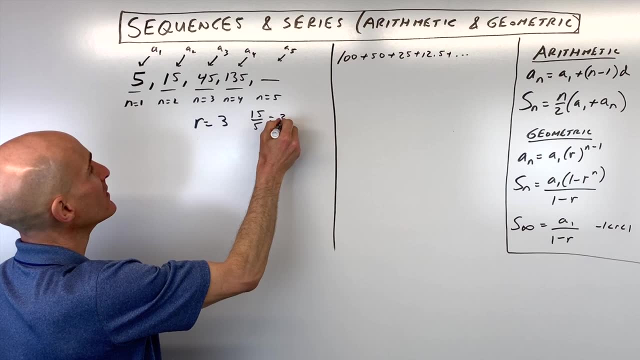 And this thing that we're multiplying by each time, this is called the ratio, so R for ratio. And if you're having trouble finding out what that ratio is, just take the number divided by the one before it. 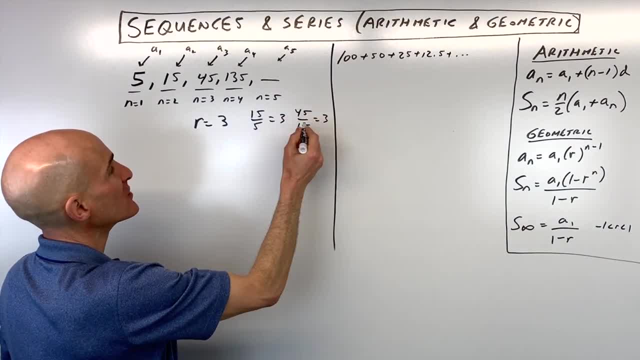 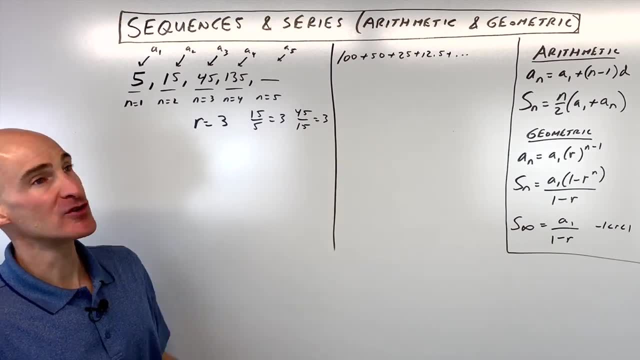 Same thing here, 45 divided by the number before it, and you can see we're getting 3333. Now if it looks like you're dividing, remember division is really like multiplying by the reciprocal, so if it looks like you were dividing by 2, that's like multiplying by a half. 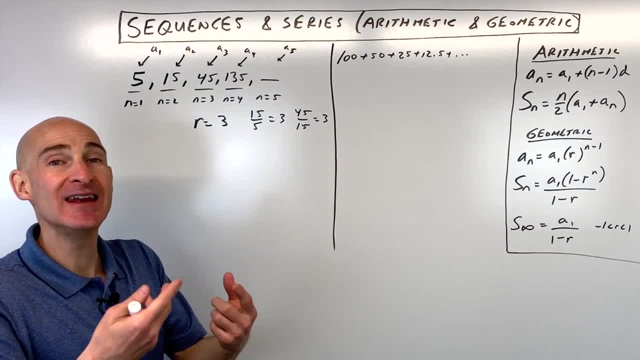 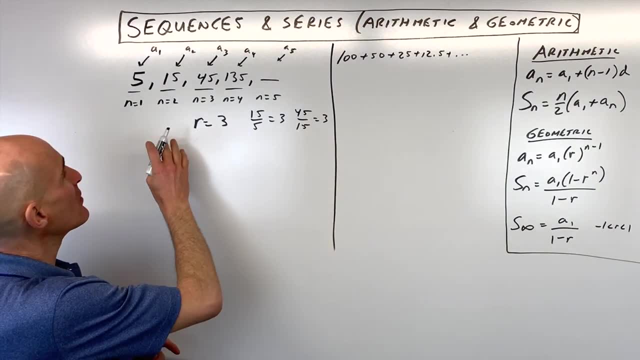 Same thing with the arithmetic ones, if it looks like you're subtracting, it's really like adding a negative number, so that's important to keep in mind. So arithmetic, you're adding the same thing, geometric, you're multiplying by the same quantity. 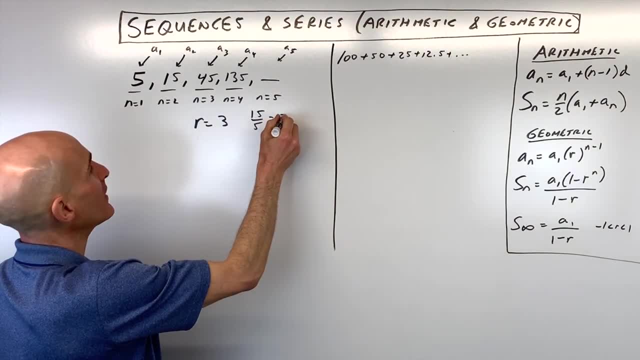 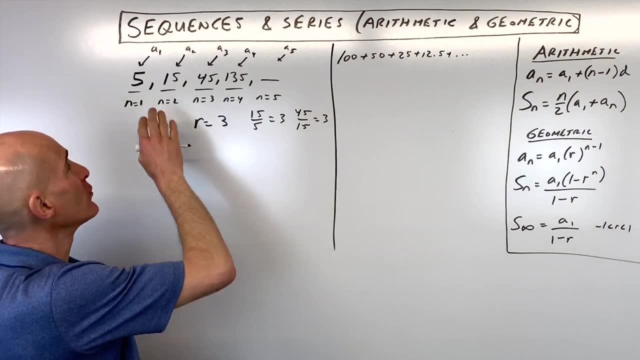 just take the number divided by the one before it. Same thing here: 45 divided by the number before it, And you can see we're getting 3, 3,, 3, 3.. Now, if it looks like you're dividing, remember. 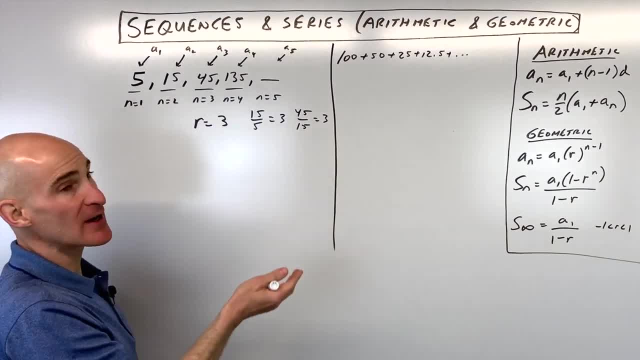 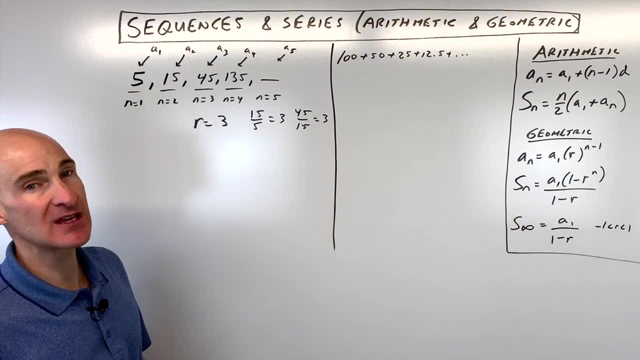 division is really like multiplying by the reciprocal. So if it looks like you were dividing by 2, that's like multiplying by a half. Same thing with the arithmetic ones. If it looks like you're subtracting, it's really like adding a negative number, So that's important to keep in. 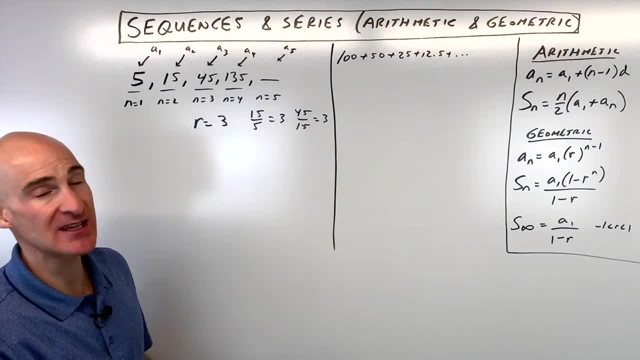 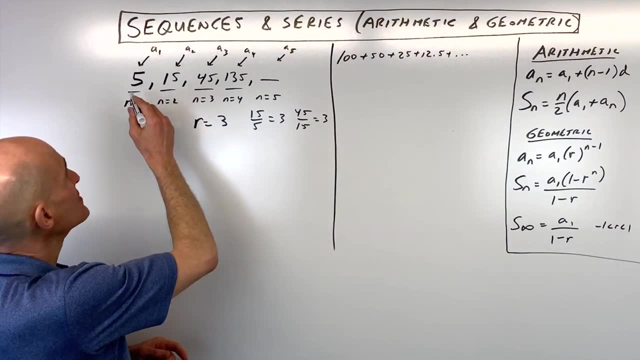 mind. So, arithmetic, you're adding the same thing. Geometric, you're multiplying by the same quantity. But now let's say we wanted to get an idea about how to find the value of this fifth term here. Well, you can see, we're starting at 5. And we're multiplying by. 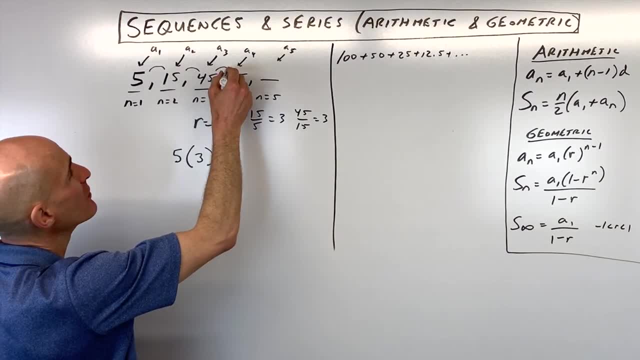 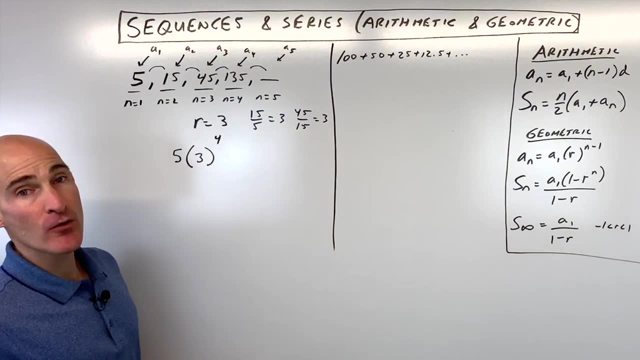 3, how many times? 1,, 2,, 3, 4.. Now notice that we're on the fifth term, but we only multiply by 3, 4 times. So that's where our formula comes from. What you do is you start at the first term. 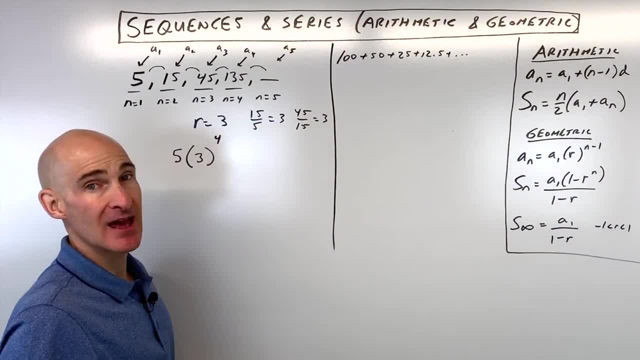 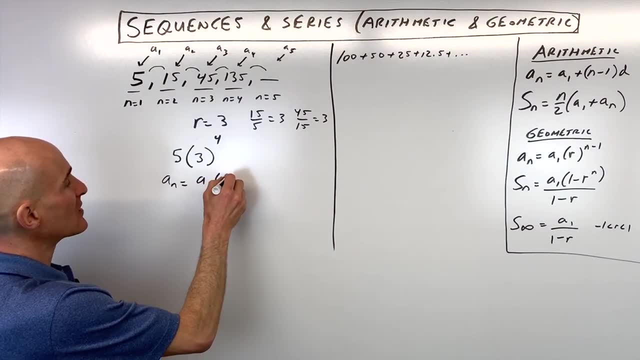 you multiply by the ratio n minus 1 times, So that's the n minus 1 power. So if we were to write this as a rule or a formula, it would be a sub n equals a sub 1 times r to the n minus 1.. Our 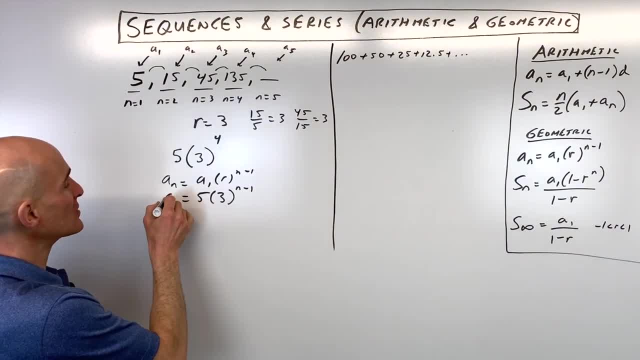 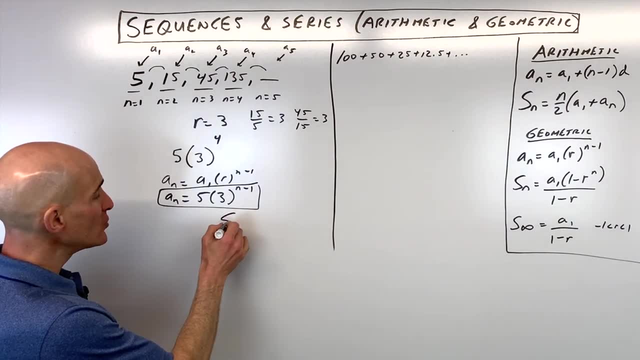 first term we said was 5.. Our ratio is 3 to the n minus 1.. So that's the n minus 1 power. So if we wanted to write it in a recursive manner, you would do the same thing. You would let the person 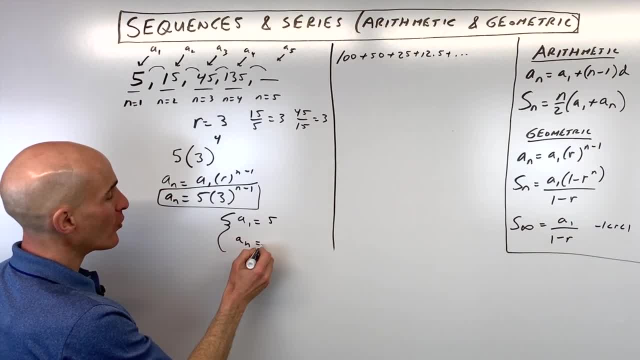 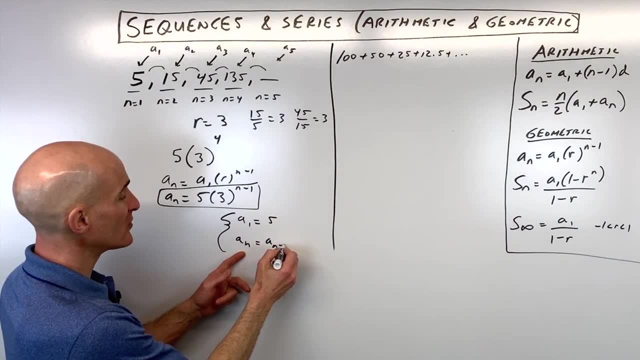 know what term you're starting at, which is 5. And then you'd give them a rule for finding that next term, next term, next term Now. recursive formulas are good for computers. A computer can do all these calculations quite quickly And you can write it like this: where you're taking the 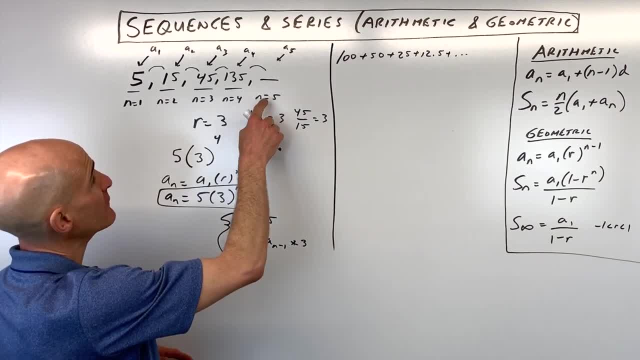 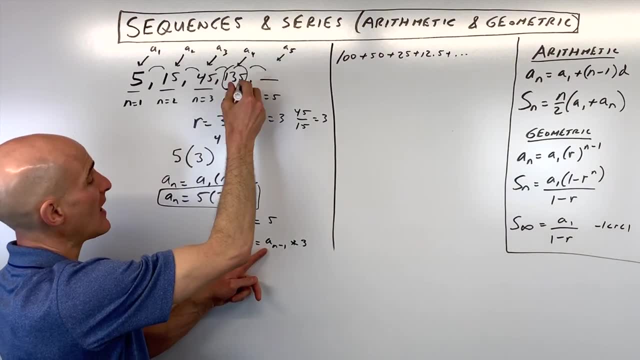 n minus 1th term, and you're multiplying by 3.. So if we wanted to find the fifth term a sub 5, we're taking the a sub 5 minus 1, which is the a sub 4th term. okay, which is this 135.. And then 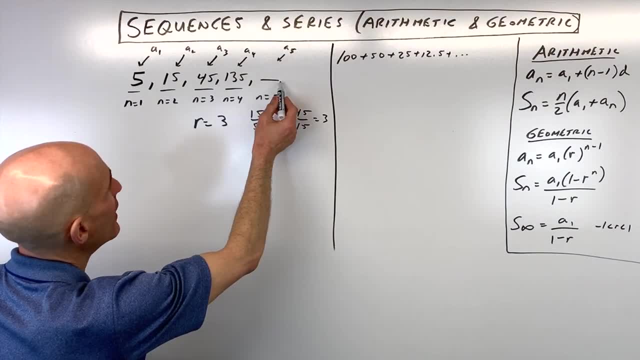 But now let's say we wanted to get an idea about how to find the value of this fifth 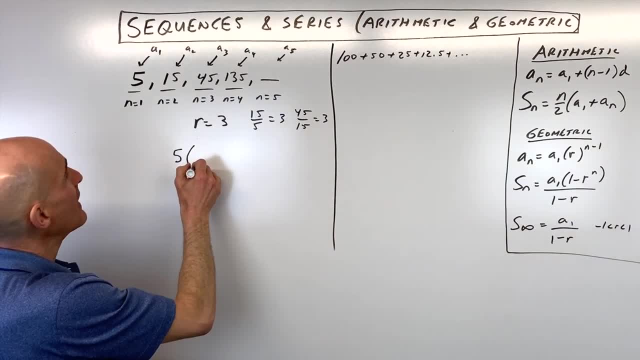 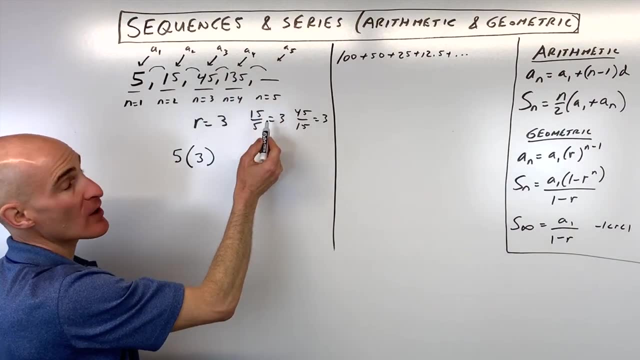 term here. Well you can see we're starting at 5, and we're multiplying by 3 how many times? 1? 2? 3? 4? Now notice that we're on the fifth term, but we only multiply by 3 four times. So that's where our formula comes from. 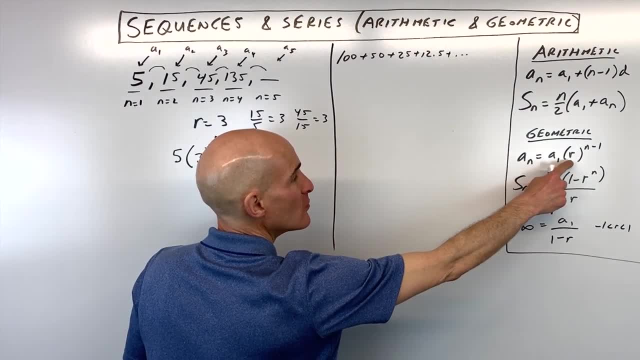 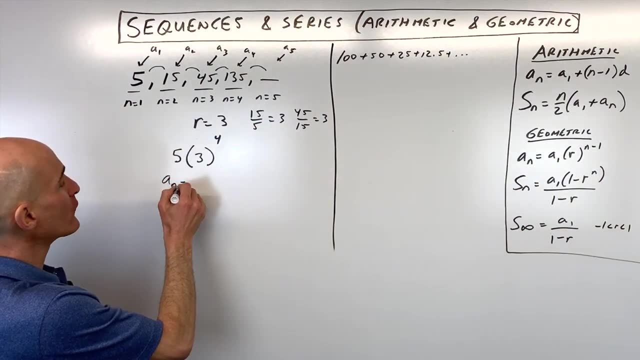 What you do is you start at the first term, you multiply by the ratio, n-1 times, so that's the n-1 power. So if we were to write this as a rule or a formula, it would be a sub n equals a sub 1 times R to the n-1, our first term we said was 5, our ratio is 3 to the n-1 power, and that's your rule or your formula. 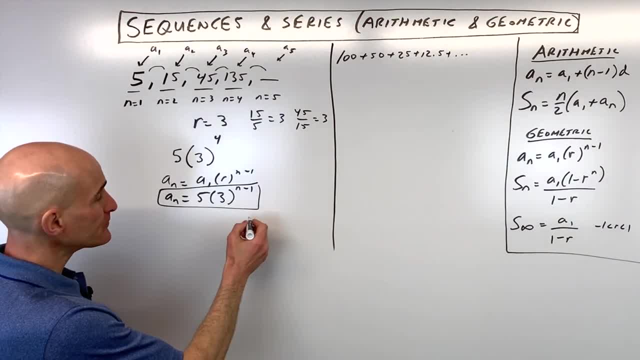 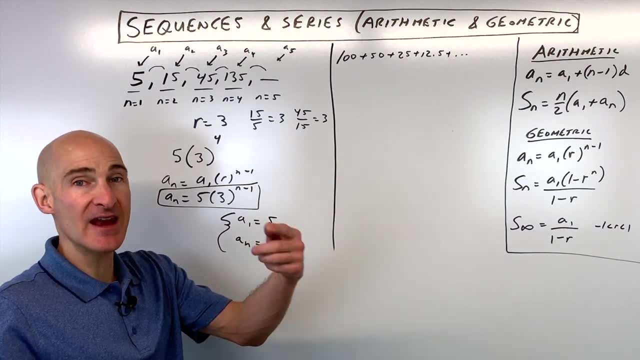 Now if you wanted to write it in a recursive manner, you would do the same thing. You would let the person know what term you're starting at, which is 5, and then you'd give them a rule for finding that next term, next term, next term. Now recursive formulas are good for computers, you know. 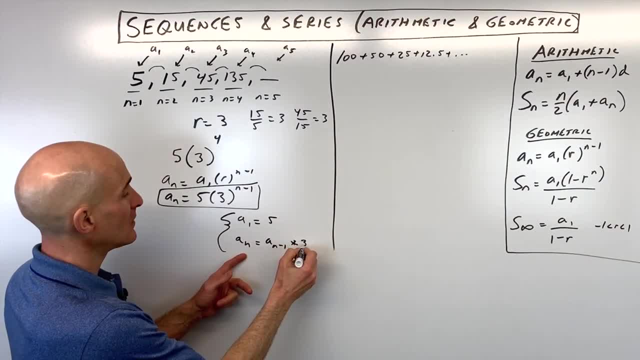 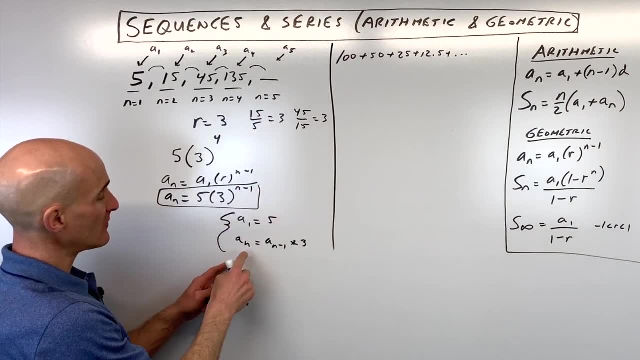 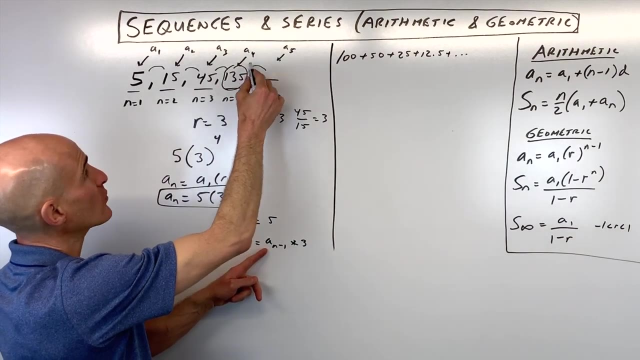 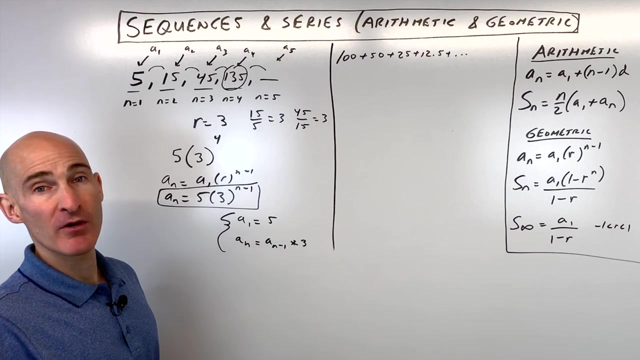 Computer can do all these calculations quite quickly, and you can write it like this, where you're taking the n-1th term and you're multiplying by 3. So if we wanted to find the fifth term, a sub 5, we're taking the a sub 5 minus 1, which is the a sub 4th term, which is this 135, and then we're multiplying by 3. Now if you wanted to find the 10th term, you might not want to keep multiplying by 3 a 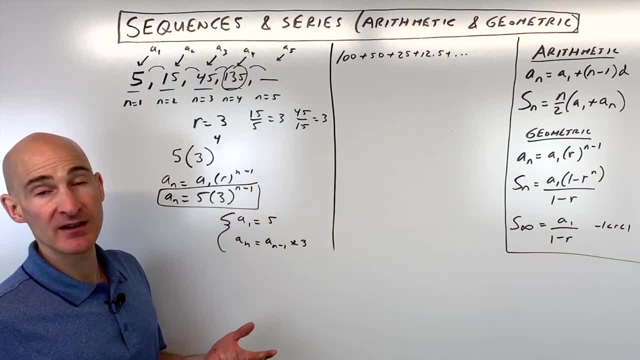 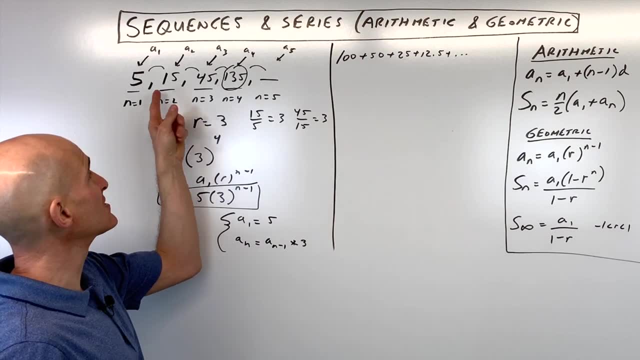 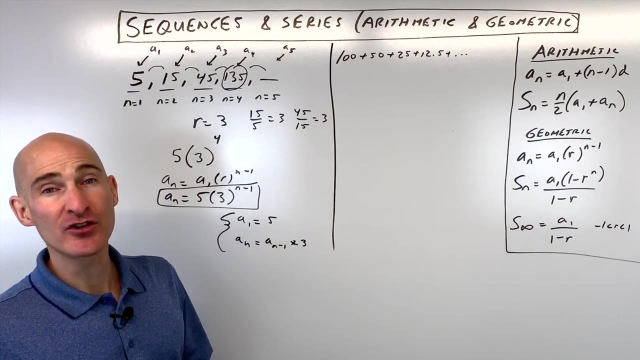 bunch of times, so you could just put in 10 for n and find the value of that 10th term. Now let's talk about how do we find the sum, we're switching from sequences to series now, how do we find the sum of let's just say the first 10 terms. Well of course we could write them all out and then add them up, but if it was like 20 terms or 100 terms, that would take too long. 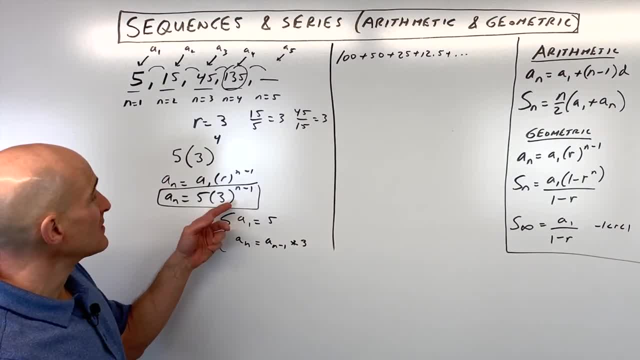 we're multiplying by 3.. Now if you wanted to find the 10th term, you might not want to keep multiplying by 3, you know a bunch of times. So you could just put in 10 for n and find the value. 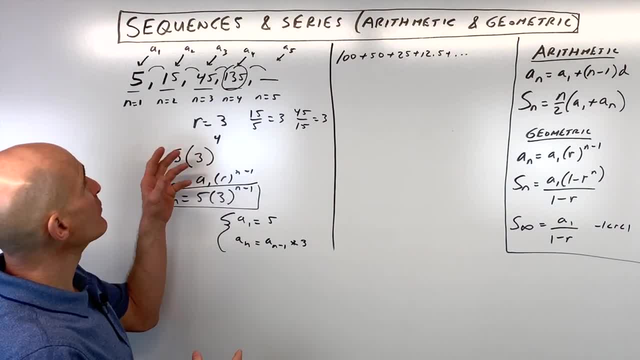 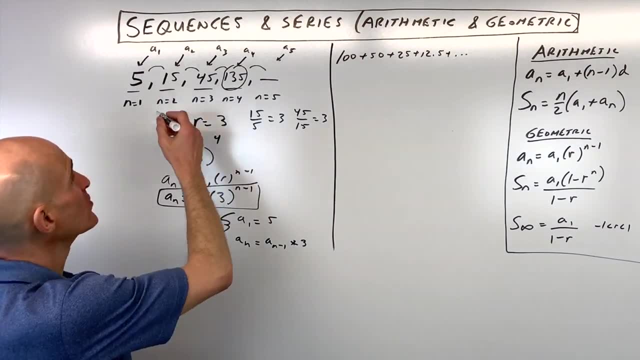 of that 10th term. Now let's talk about how do we find the sum. We're switching from sequences to series, now How do we find the sum of, let's just say, the first 10 terms? Well, of course, 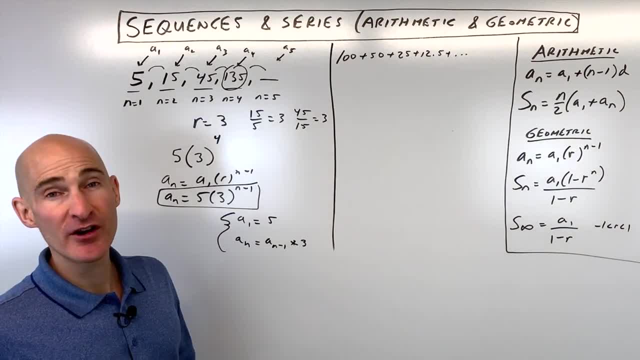 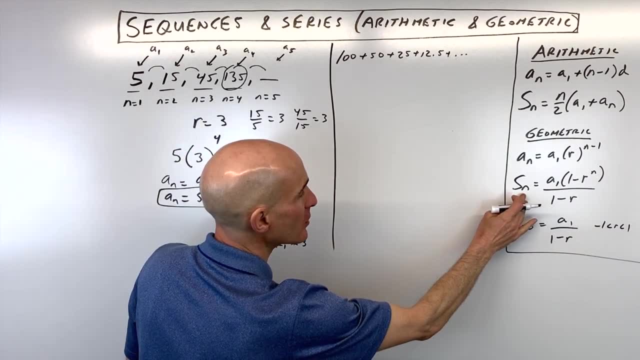 we could write them all out and then add them up, But if it was like 20 terms or 100 terms, that would take too long. So let's go ahead and figure out the sum of the first 10 terms. We're going to be using this formula right here, And the first term we know is 5.. So that's. 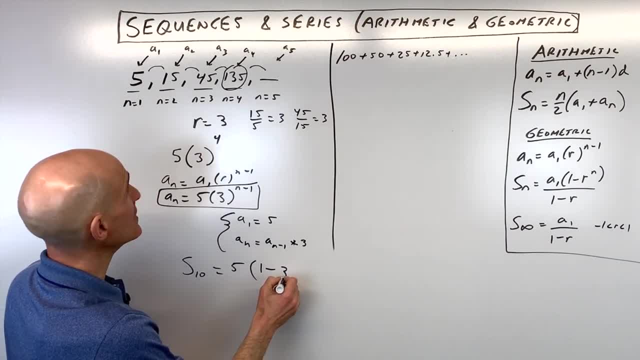 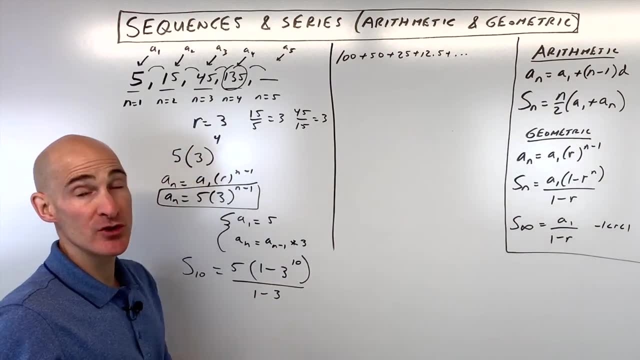 a sub 1.. We have 1 minus the ratio, which is 3, to the 10th power, because we have 10 terms all divided by 1 minus the ratio, 1 minus 3.. Now, when you work with this formula, you want to be: 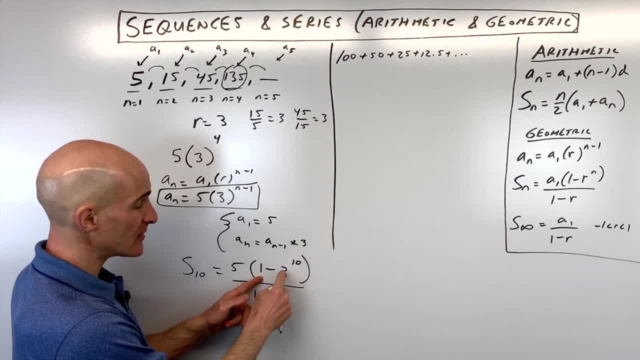 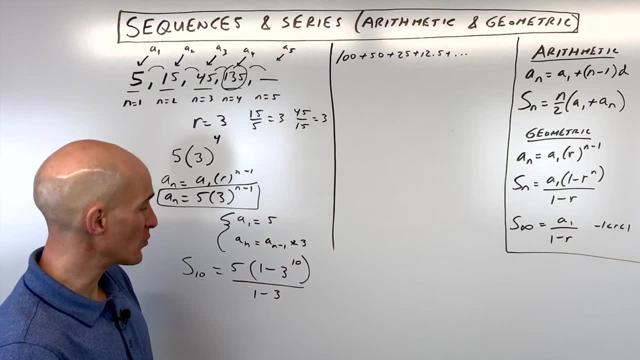 careful. Some students mistakenly will write 1 minus 3, oh, that's negative 2 to the 10th power. But you want to follow the order of operations. You want to do the exponents first and then the subtraction. Okay, so you're with me. So let me go to the 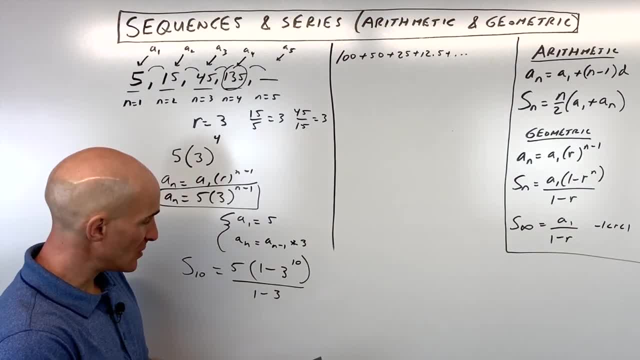 calculator on this one And I'm just going to do it here. You can do it in steps if you want. So I'm going to do 3 to the 10th. first I'm going to do 1 minus that answer. I'm going to multiply by. 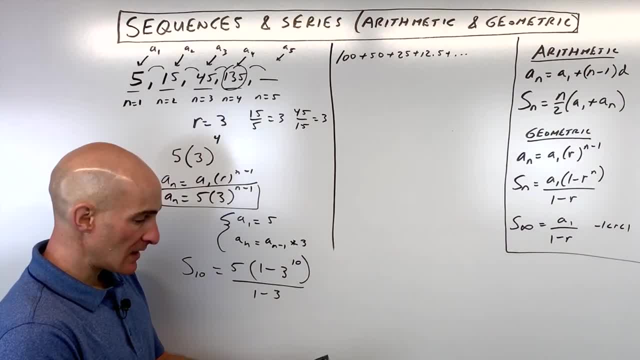 5,, and then I'm going to divide by negative 2.. And that comes out to 147,620.. And that's the sum of the first 10 terms. Now notice how this is such a large number. And it's because every time you 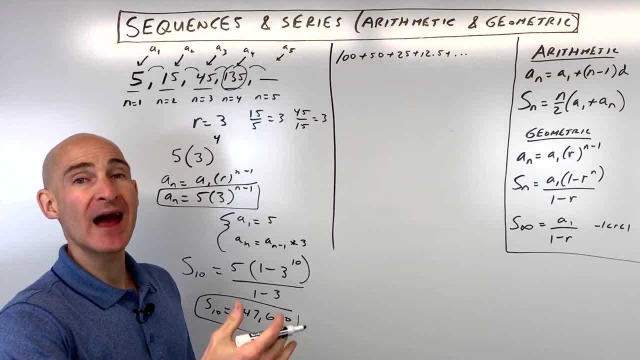 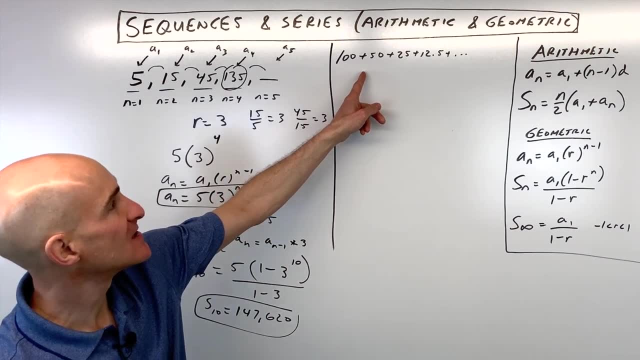 multiply by 3, you know you're tripling, tripling, tripling. It's growing exponentially, So that's why we're getting into quite a large number quite quickly. Now, another type of geometric series we want to look at are these ones here where you have an infinite number of terms. See the dot. 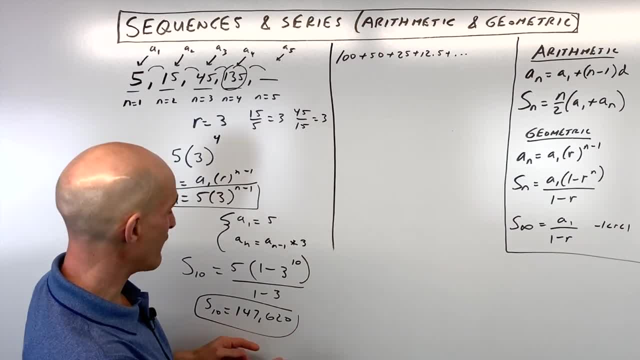 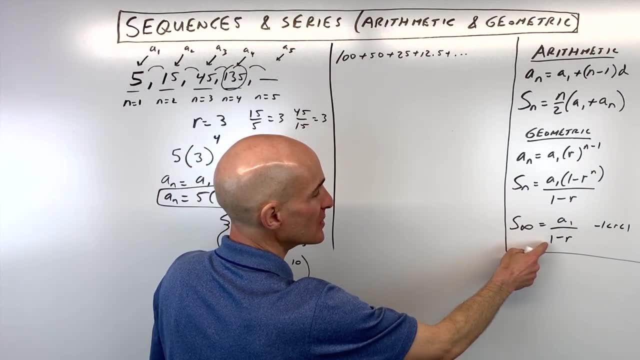 dot, dot, So it continues on and on and on, as opposed to a finite set of terms. So this is the form we're going to use for finite. This is the form we're going to use for infinite geometric series. But the important thing here is that 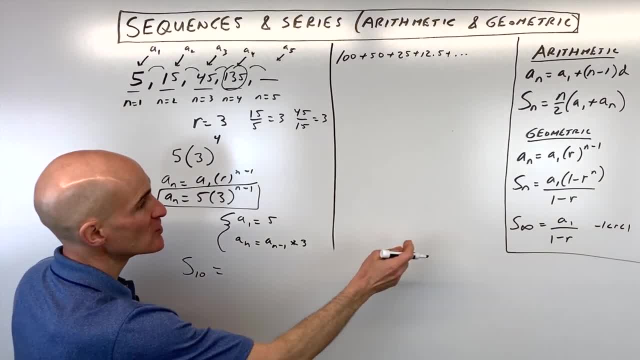 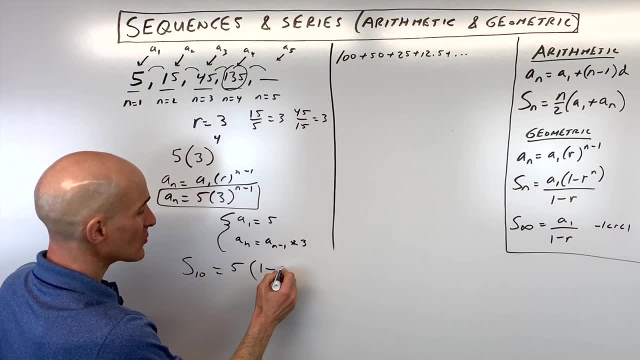 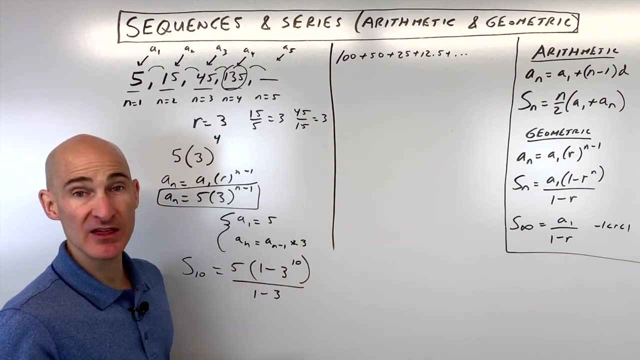 So let's go ahead and figure out the sum of the first 10 terms, we're going to be using this formula right here, and the first term we know is 5, so that's a sub 1. We have 1 minus the ratio, which is 3, to the 10th power, because we have 10 terms, all divided by 1 minus the ratio, 1 minus 3. Now when you work with this formula, you want to be careful, some students mistakenly will write 1 minus 3, oh that's negative 2 to the 10th power, but you want to follow the order of operations, you want to do the exponents first, and then the subtraction. Okay, so are you with me? So let me go to the calculator on this one, and I'm just going to do it here, you can do it in steps if you want, so I'm going to do 3 to the 10th first, I'm going to do 1 minus that answer, I'm going to multiply by 5, and then I'm going to divide by negative 2, and that comes out to 147,620, and that's the sum of the first 10 terms. 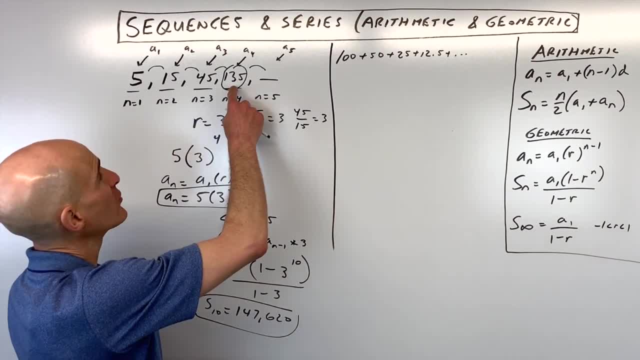 Now notice how this is such a large number, and it's because every time you multiply by 3, you know, you're tripling, tripling, tripling. 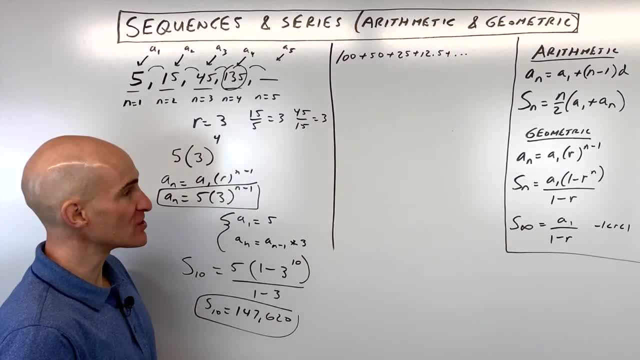 It's growing exponentially, so that's why we're getting into quite a large number quite quickly. 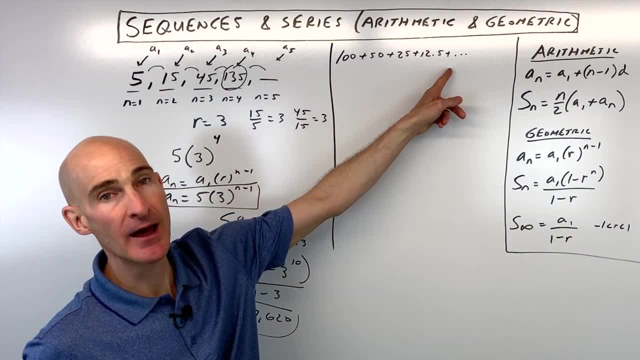 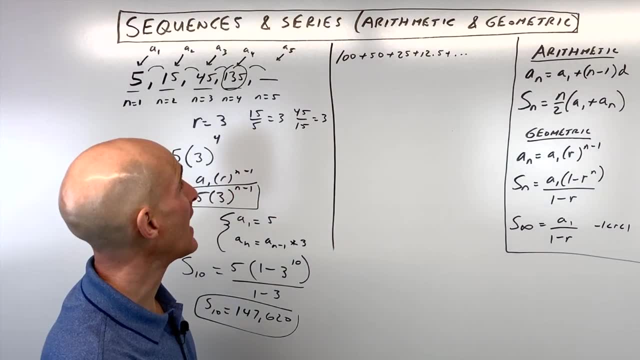 Now another type of geometric series we want to look at are these ones here where you have an infinite number of terms, see the dot, dot, dot, so it continues on and on and on, as opposed to a finite set of terms. 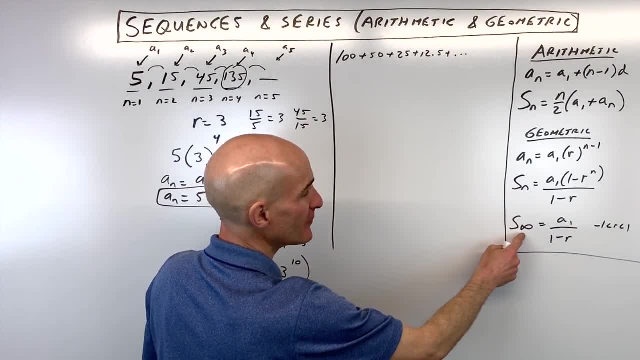 So this is the formula we're going to use for finite, this is the formula we're going to use for infinite geometric series, but the important thing here is that when you multiply by that ratio. 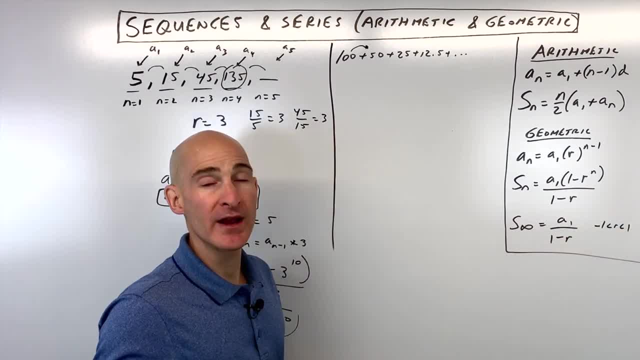 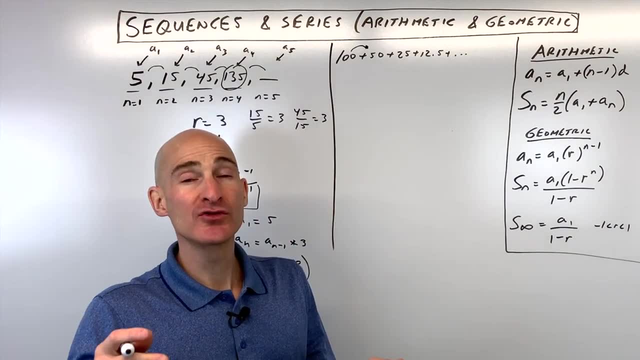 That ratio has to be in between negative 1 and 1, so what happens, you can see I'm multiplying by a half, that's 50, a half, that's 25, 12.5, what is this number getting closer and closer to? 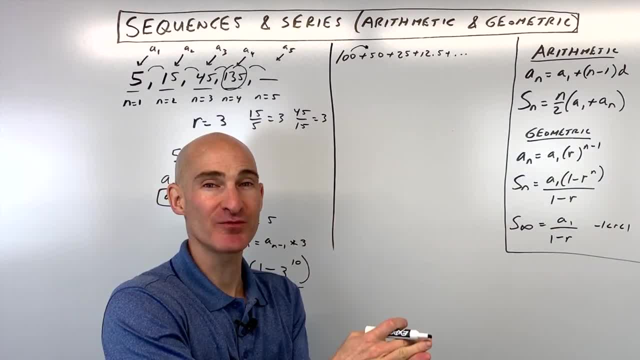 0. So that means that it's converging, ok, so it's approaching 0, and we can sum all those terms up. 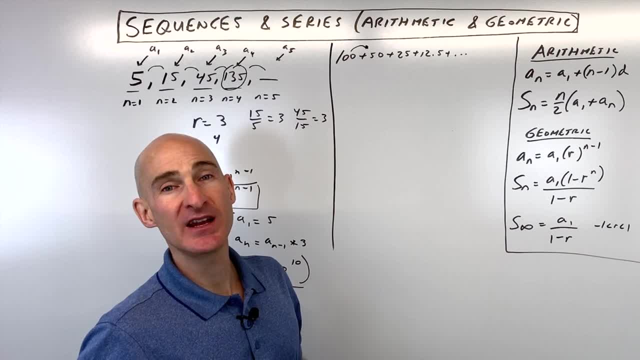 Now if we were multiplying by 2 each time, that would be what we call divergent, and it would be going gradually to infinity if we tried to add all those terms up, of course it would be an infinite sum. 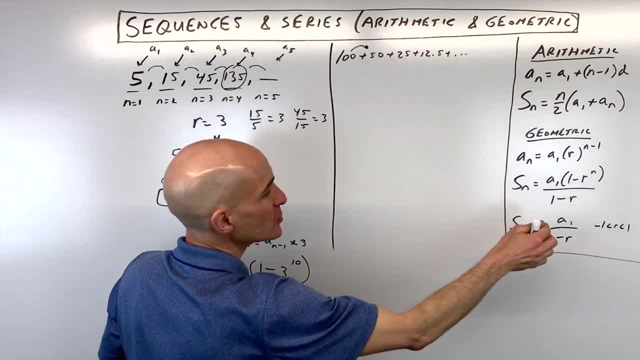 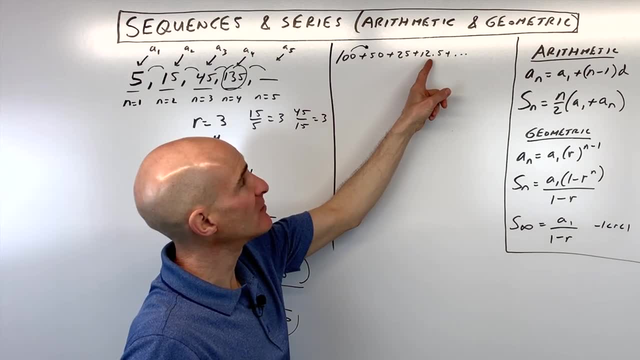 when you multiply by that ratio, that ratio has to be in between negative 1 and 1.. So what happens? you can see. I'm multiplying by a half, That's 50,. a half, that's 25,, 12.5.. What is this number? 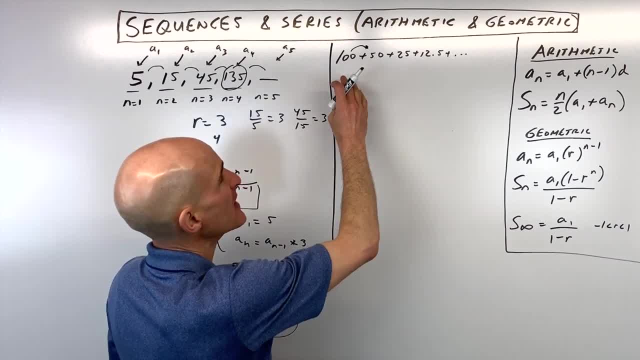 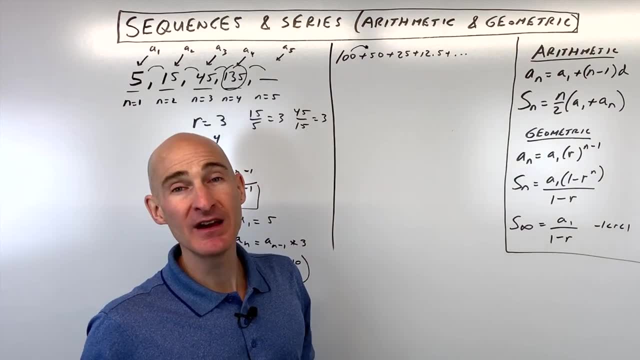 getting closer and closer to Zero. So that means that it's converging, okay, So it's approaching zero. And we can sum all those terms up Now. if we were multiplying by 2 each time, that would be what we call divergent, and it would be going to gradually to infinity. If we tried to add all. 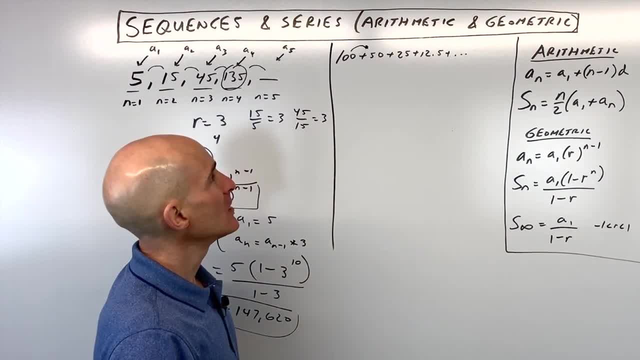 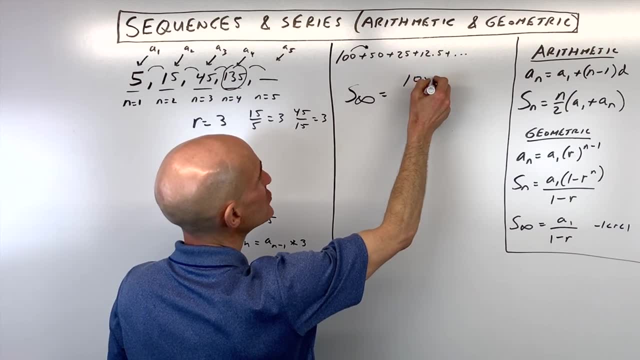 of these together we would get zero, So we wouldn't be able to actually get an exact value for that sum. So here, what we're going to do now is we're going to use our formula, We're going to say the sum of an infinite geometric series. it's the first term, which is 100, over 1, minus the ratio. 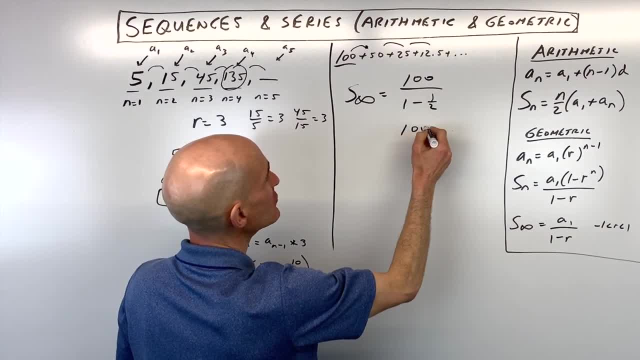 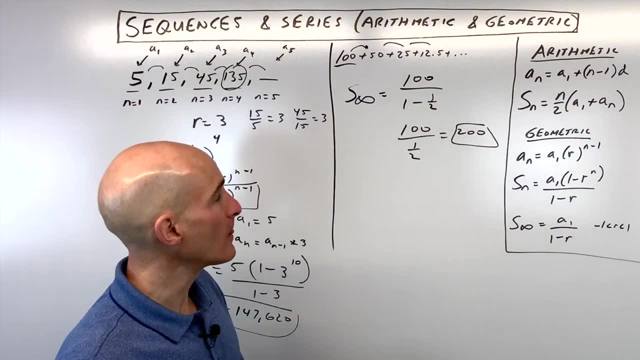 we're multiplying by a half each time to get to the next term. So this comes out to 100 divided by a half, which equals 200.. Remember, when you divide by a fraction, it's like multiplying by the reciprocal. Again, sometimes, you know, you may have a problem where it looks like. 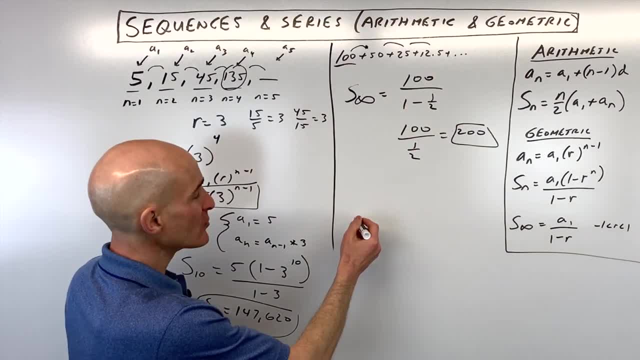 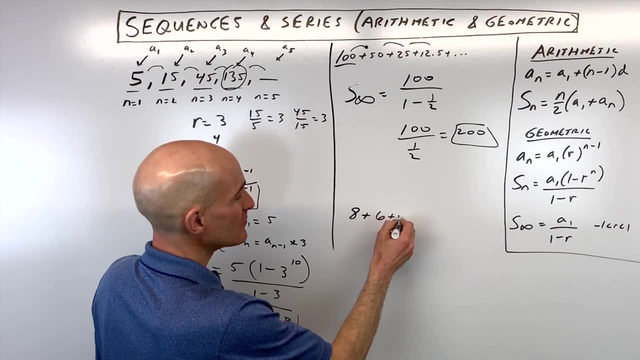 it's getting smaller, right, but it might actually be divergent, like, for example: here's a little trick sometimes that teachers might put on your test. it might be something like this: like eight plus six plus four plus two, and you might say, oh, it's getting closer to zero, but what happens? 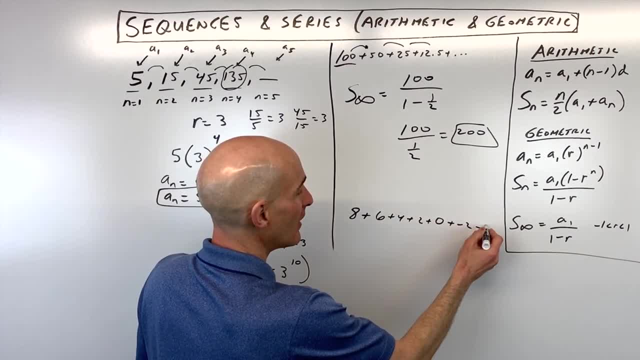 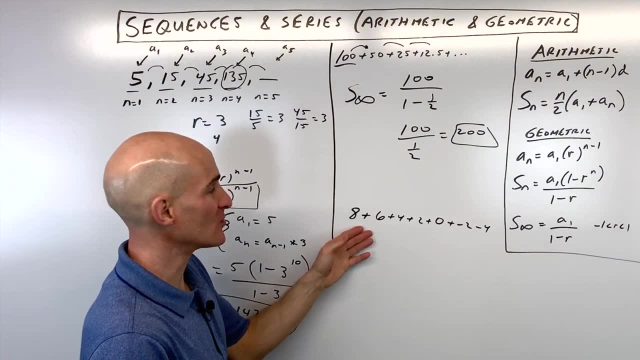 because this is arithmetic. you actually just flew right by zero, right? so you keep subtracting two and eventually this is going to go to negative infinity. you can't actually find that sum. it's going to go to negative infinity, right? so it has to be geometric and the ratio has to be between: 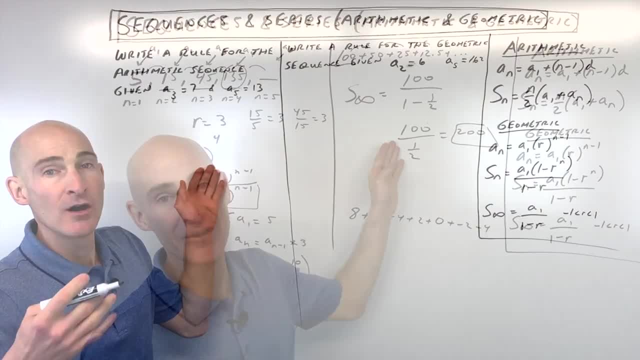 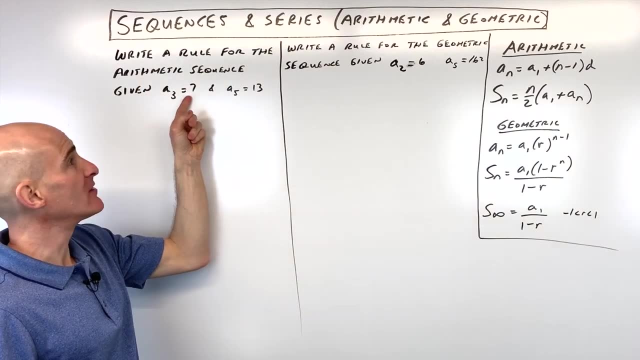 be between negative one and one, for it to converge and for you to find the sum. let's look at a couple more challenging problems. so write a rule for the arithmetic sequence: when you're given, the third term is seven and the fifth term is 13. so how do we do something like that? well, let's go over here. 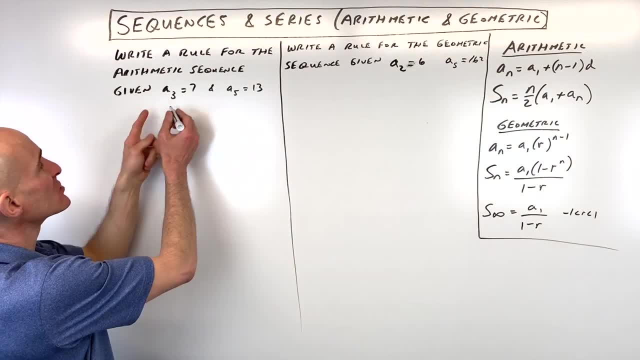 to our arithmetic explicit formula, and let's take this term here. we know that the value of the third term is seven, so we're going to call this seven the first term. we don't actually know the value of the third term is seven, so we're going to call this seven the first term. we don't 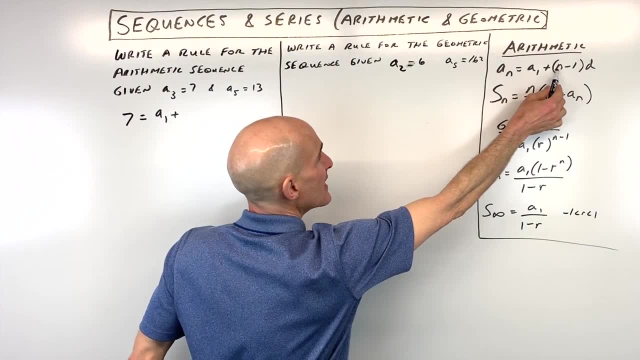 know, the value of the third term is seven, so we're going to call this seven. the first term, we don't know, and the third term, okay. that's: n equals 3,, 3 minus 1 is 2, and the difference we also. 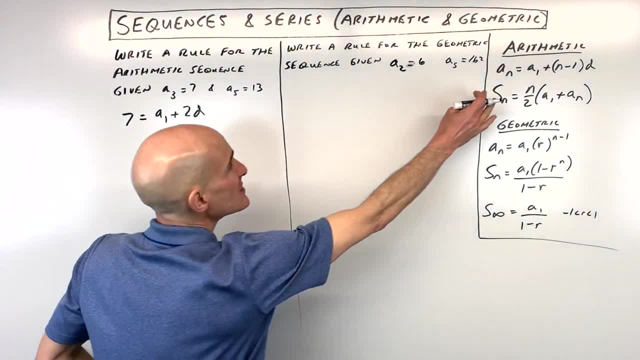 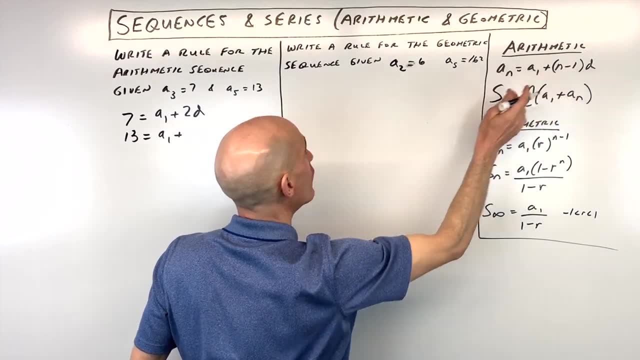 don't know. Let's take this term here: the fifth term is 13,. so, same thing, the value of that term is 13,. the first term we don't know but 5, which is the term that we're on. 5 minus 1 is 4, times the difference, which we don't know. So what we have is a system. 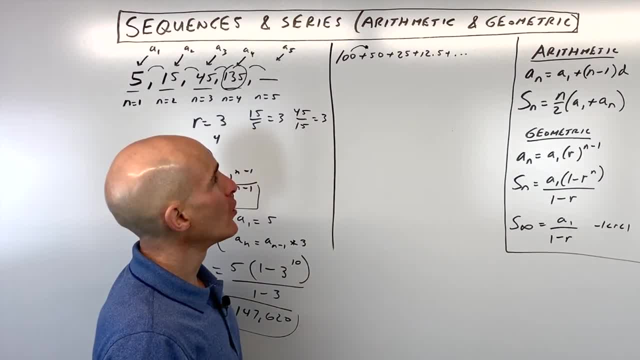 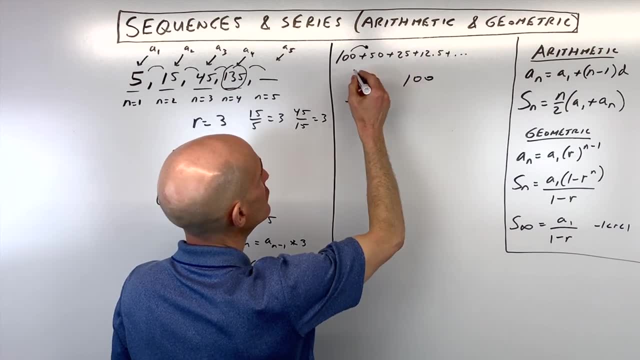 So we wouldn't be able to actually get an exact number. We wouldn't be able to get an exact, you know, value for that sum. So here what we're going to do now is we're going to use our formula, we're going to say the sum of an infinite geometric series, it's the first term, which is 100, over 1 minus the ratio, we're multiplying by a half each time to get to the next term, so this comes 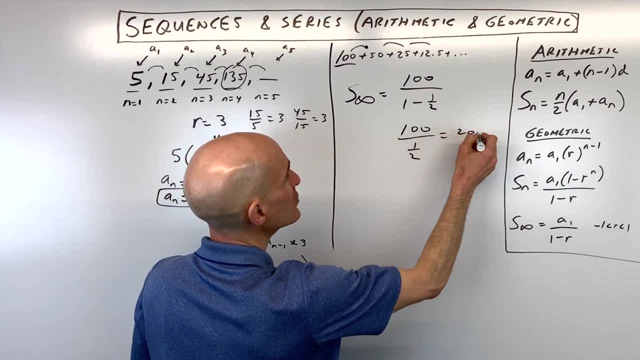 out to 100 divided by a half, which equals 200, remember when you divide by a fraction it's like multiplying by the reciprocal. 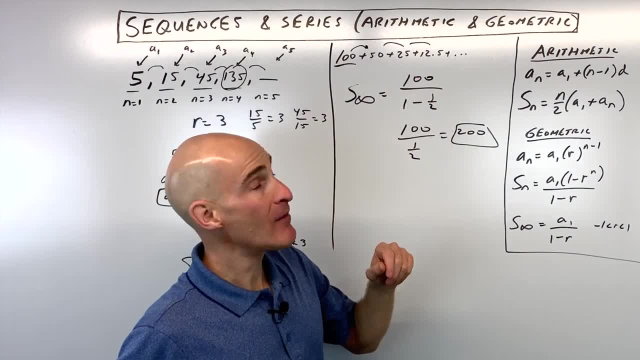 Again, sometimes, you know, you may have a problem where it looks like it's getting smaller, right? 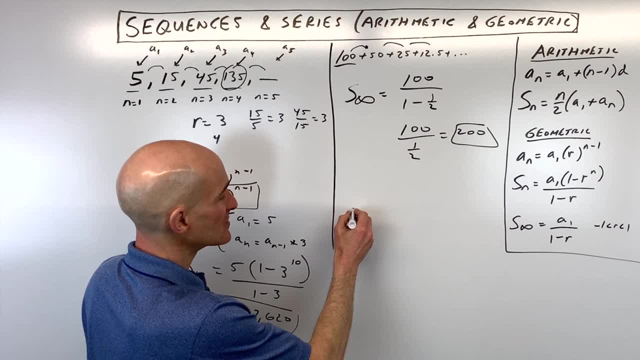 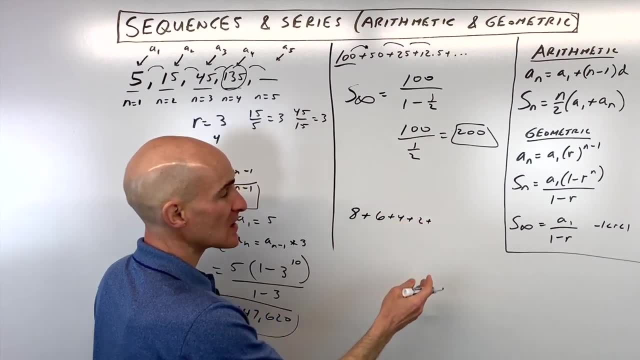 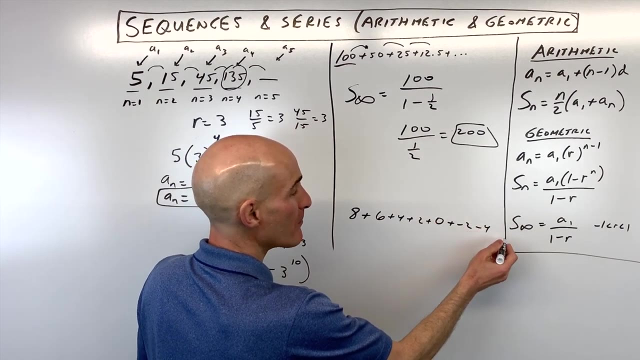 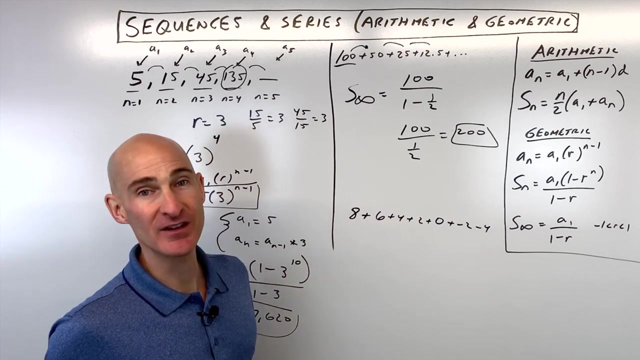 But, it might actually be divergent, like for example, here's a little trick sometimes that teachers might put on your test, it might be something like this, like 8 plus 6 plus 4 plus 2, and you might say, oh, it's getting closer to 0, but what happens, because this is arithmetic, you actually just flew right by 0, right? So you keep subtracting 2, and eventually this is going to go to negative infinity, you can't actually find that sum, it's going to go to negative infinity, right? 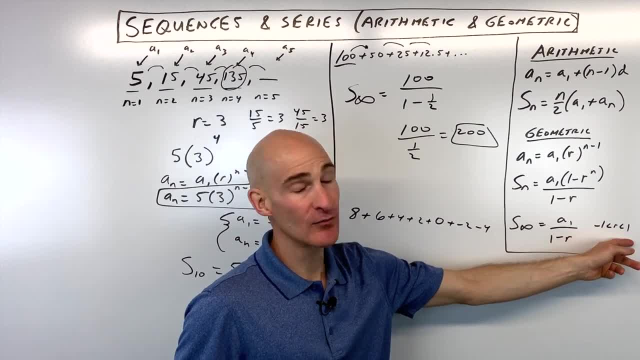 So it has to be geometric, and the ratio has to be between, be between negative 1 and 1 for it to converge, and for you to find the sum. 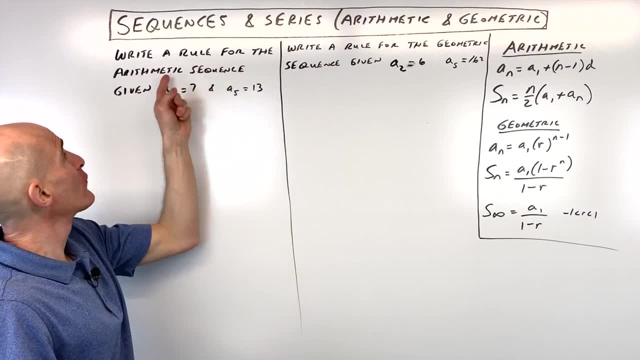 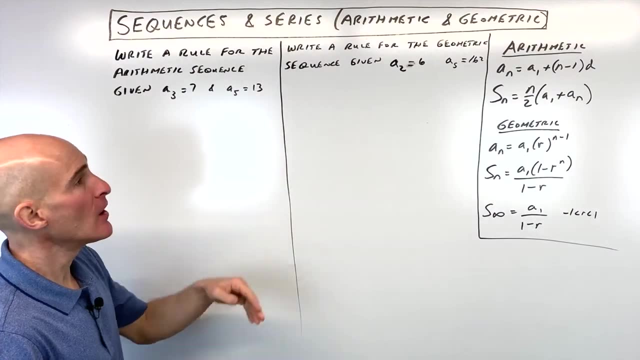 Let's look at a couple more challenging problems, so write a rule for the arithmetic sequence when you're given the third term is 7, and the fifth term is 13, so how do we do something like that? 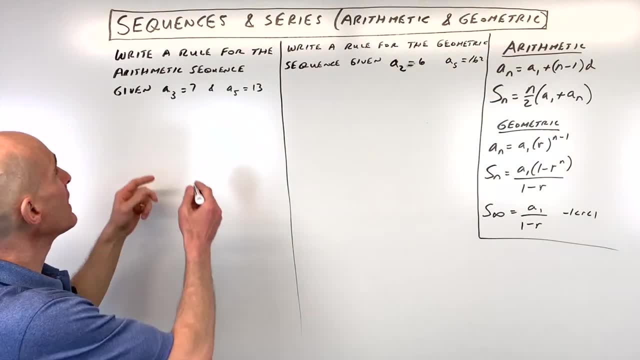 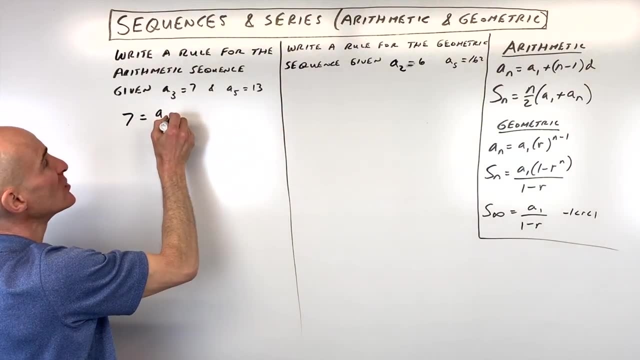 Well, let's go over here to our arithmetic explicit formula, and let's take this term here, we know that the value of the third term is 7, so we're going to call this 7, the first term we don't actually know, and the third term, okay, that's n equals 3, 3 minus 1 is 2. 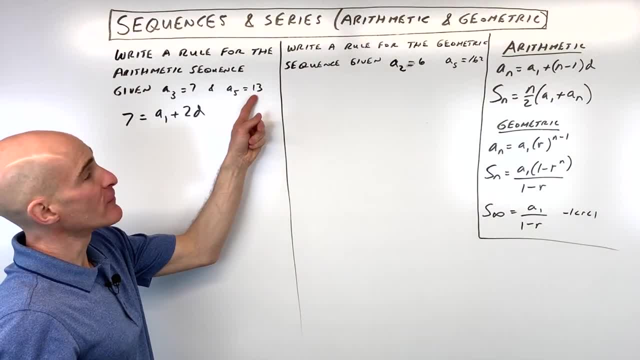 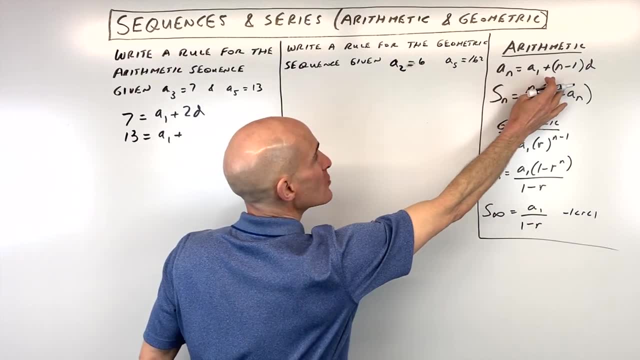 And the difference we also don't know. Let's take this term here, the fifth term is 13, so same thing, the value of that term is 13, the first term we don't know, but 5, which is the term that we're on, 5 minus 1 is 4, times the difference, which we don't know. 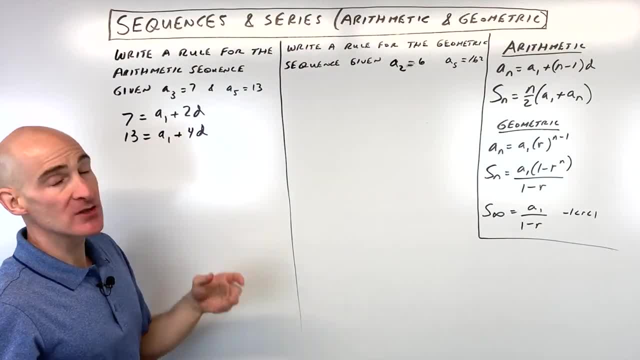 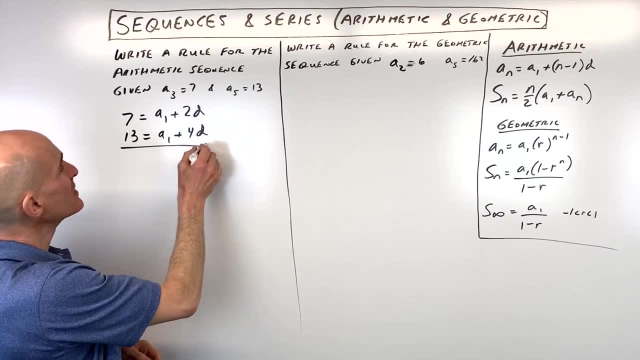 So what we have is a system of equations where we have two variables and two equations, so we can solve for a1 and d. So what we're going to do is, let's go ahead and subtract these equations, we're going to use the elimination method. 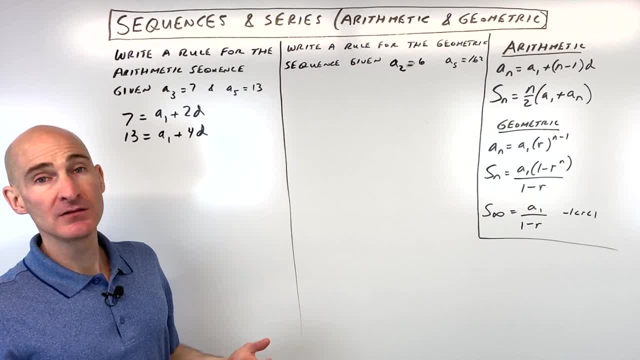 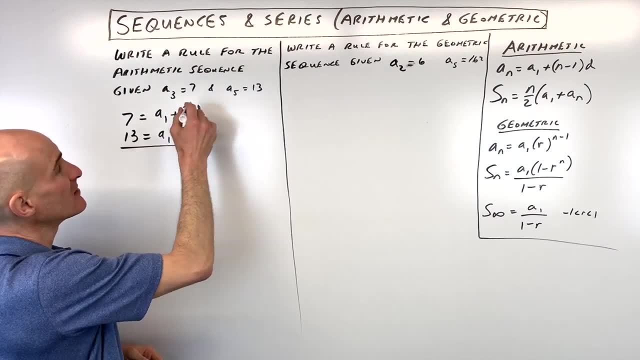 of equations where we have two variables and two equations. so we can solve for a1 and d. So what we're going to do is let's go ahead and subtract these equations. we're going to use the elimination method, So the a1's would cancel out. 7 minus 13 is negative. 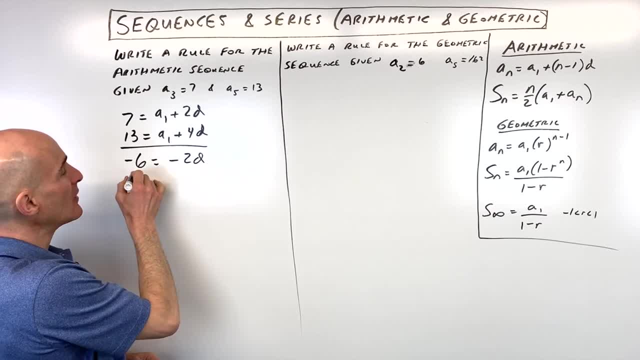 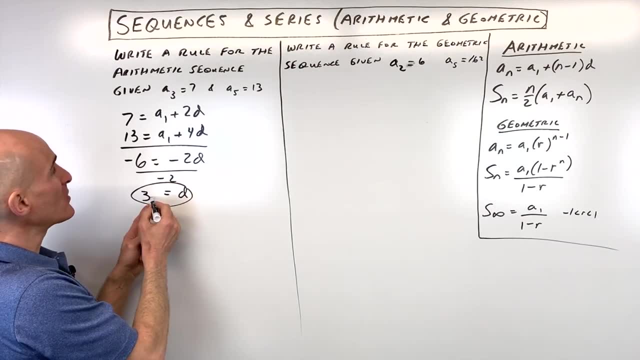 6, 2d minus 4d is negative 2d, and if we divide both sides by negative 2,, you can see that d is equal to positive 3.. Now if we put 3 back into either one of these equations, I'll. 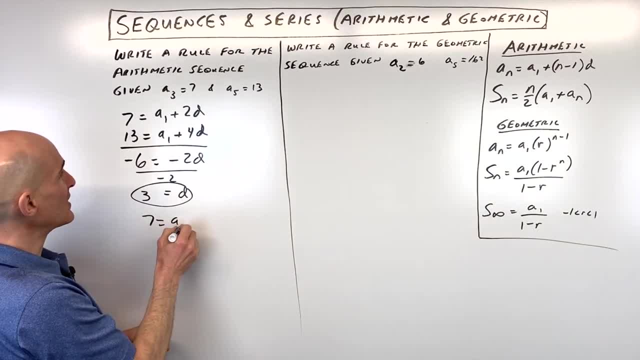 just put it into this top one: here we have 7 equals a1, plus 2 times 3, which is 6, and if we subtract 6 from both sides, you can see that a1 is equal to 1.. So now, if we put it, 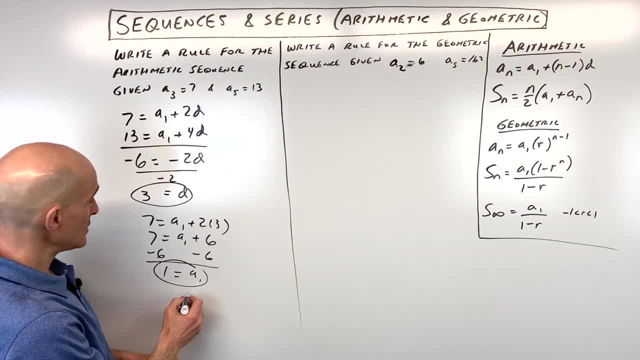 all back together. we can write a rule for this sequence. We have: a sub n equals a sub 1, which is 1,, plus n minus 1 times d, which is 3, and then I like to just kind of simplify. 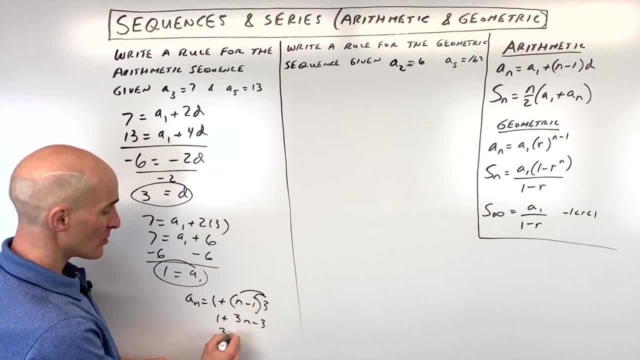 this down a little bit. by distributing and combine like terms, we have: 3n minus 2 equals a sub n. Now you can test it out. if you want, you can put 5 in, for example 15 minus 2, that's. 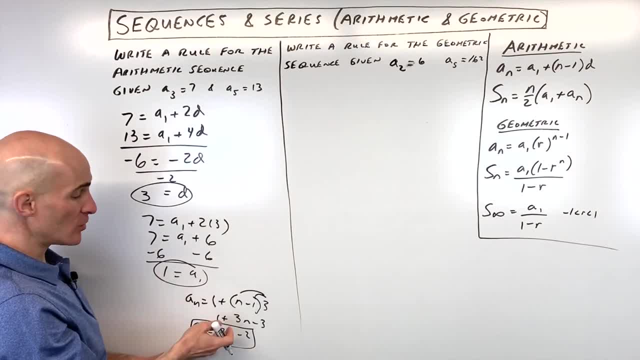 13,. you can put 3 in 3 times 3 is 9, minus 2 is 7,. you know it checks out and that's our formula for our arithmetic sequence. But for this one it says: write a rule for the. 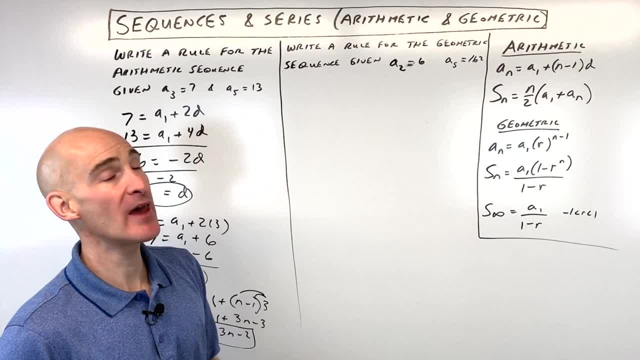 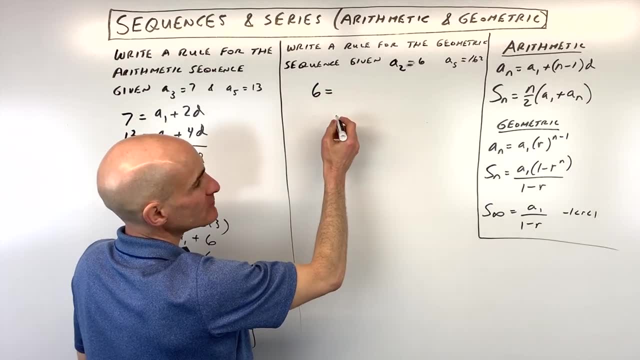 geometric sequence. given two terms, how would you do that one? Well, same thing. we're going to go to our geometric explicit formula. the value of the second term is 6, and we don't know what the first term is and we don't know what the ratio is, but we know that. second, 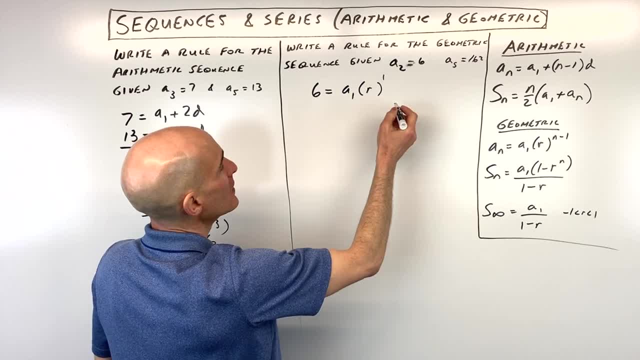 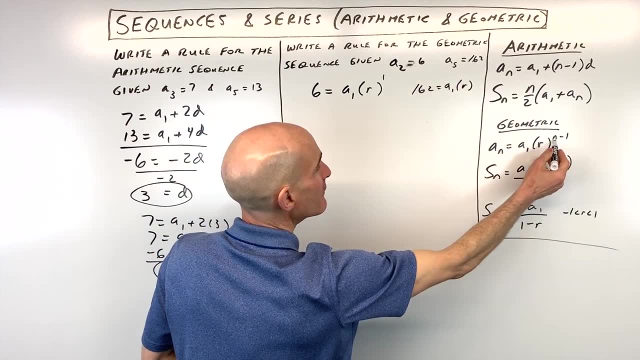 term. so 2 minus 1, n is equal to 2, so this is 1.. Over here we have 162 equals. we don't know the first term, we don't know the ratio, but 5 minus 1 is. 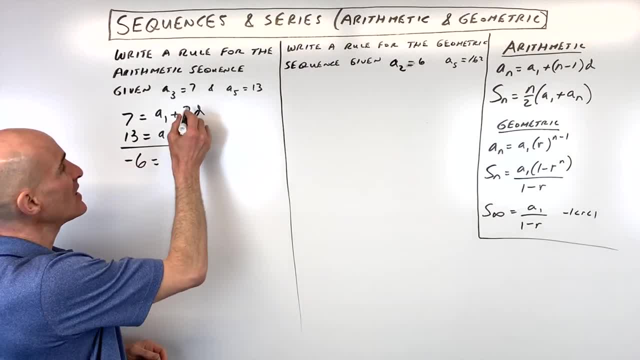 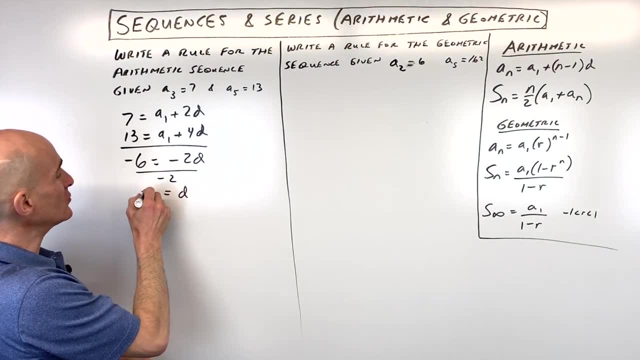 So the a1s would cancel out, 7 minus 13 is negative 6, 2d minus 4d is negative 2d, and if we divide both sides by negative 2, you can see that d is equal to positive 3. 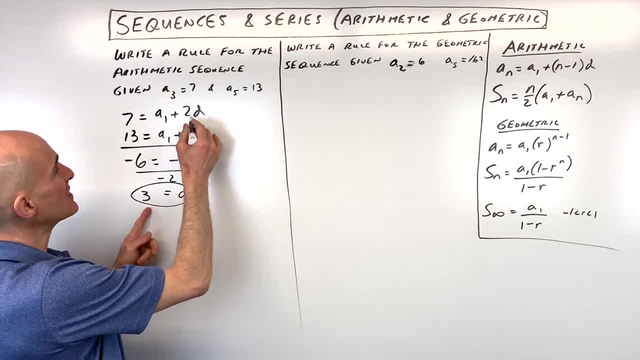 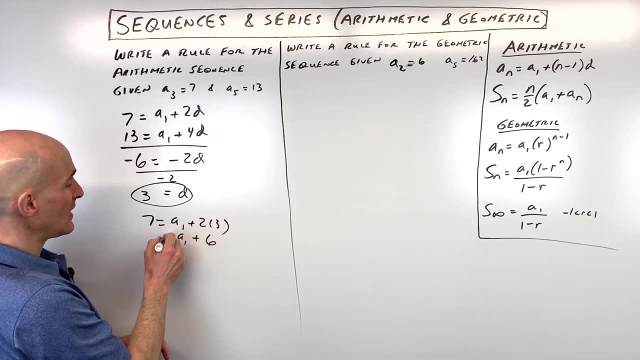 Now if we put 3 back in to either one of these equations, I'll just put it into this top one here, we have 7 equals a1 plus 2 times 3, which is 6, and if we subtract 6 from both sides, you can see that a1 is equal to 1. 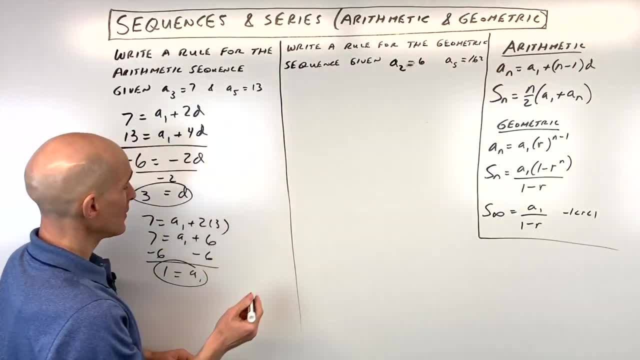 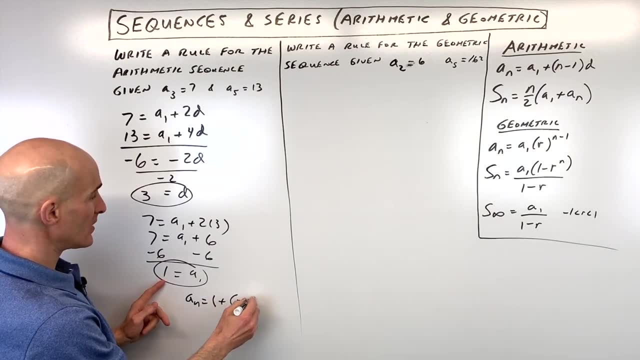 So now if we put it all back together, we can write a rule for this sequence. We have a sub n equals a sub 1, which is 1, plus n minus 1 times d, which is 3, and then I like to just kind of simplify this down a little bit by distributing, and combine like terms, we have 3n minus 2 equals a sub n. 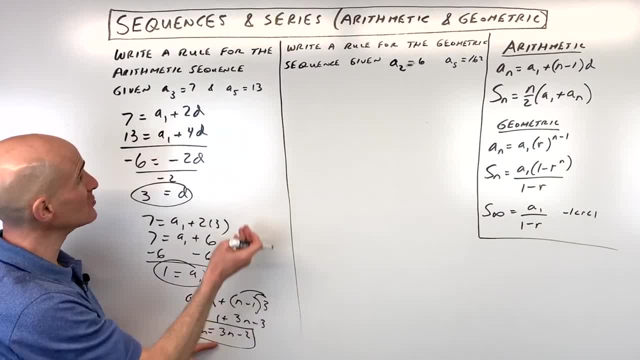 Now you can test it out if you want, you can put 5 in for example, 15 minus 2, that's 13, you can put 3 in, 3 times 3 is 9, minus 2 is 7, you know, it checks out, and that's our formula for our arithmetic sequence. 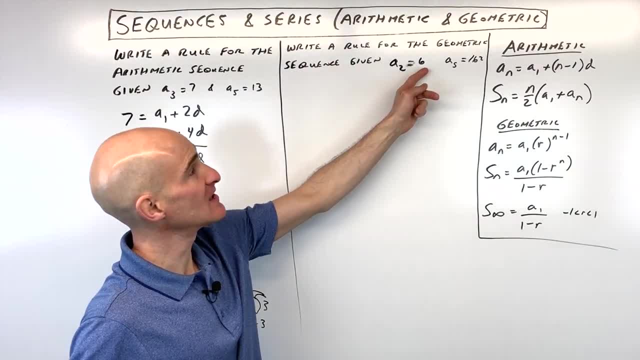 But for this one, it says write a rule for the geometric sequence given two terms. How would you do that one? 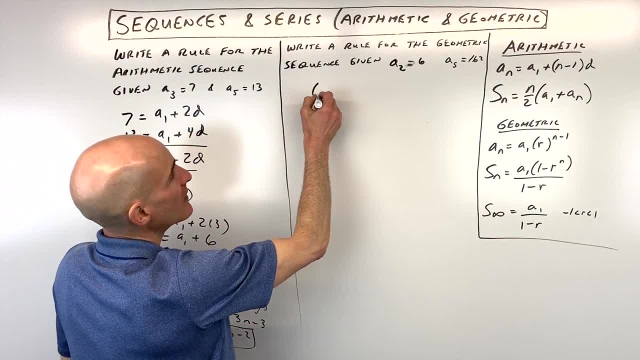 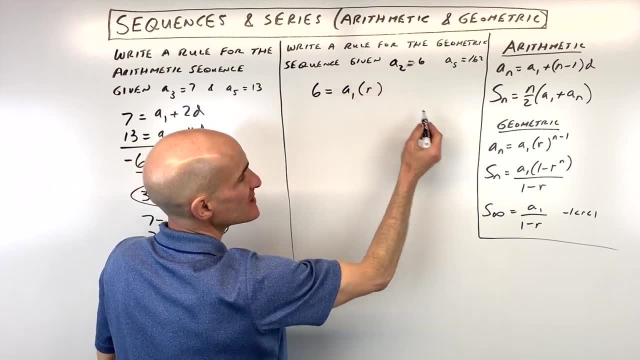 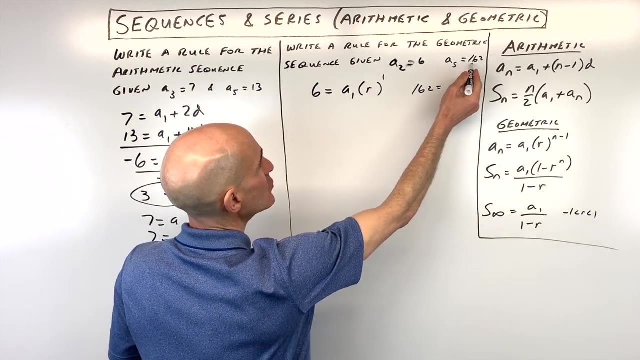 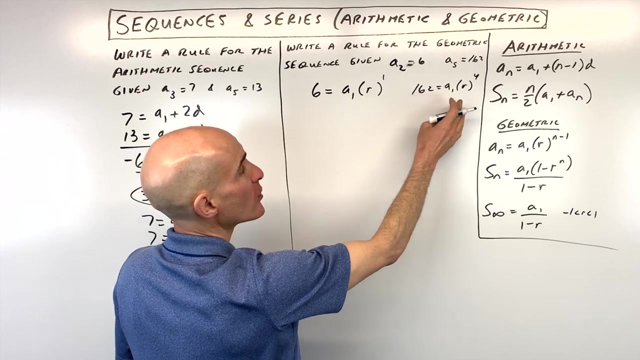 Well same thing, we're going to go to our geometric explicit formula, the value of the second term is 6, and we don't know what the first term is, and we don't know what the ratio is, but we know that second term, so 2 minus 1, n is equal to 2, so this is 1. Over here we have 162 equals, we don't know the first term, we don't know the ratio, but 5 minus 1 is 4. So now we have two variables, the first term and the ratio, and we have two equations, we can solve that system. 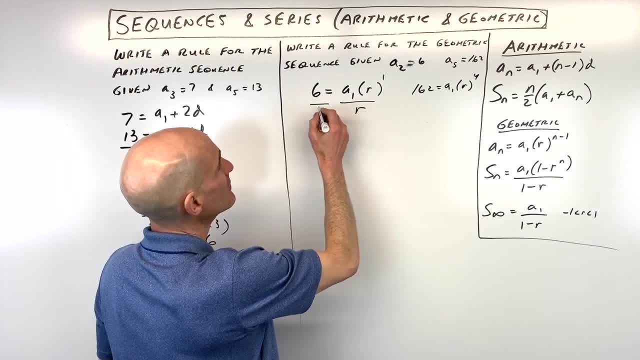 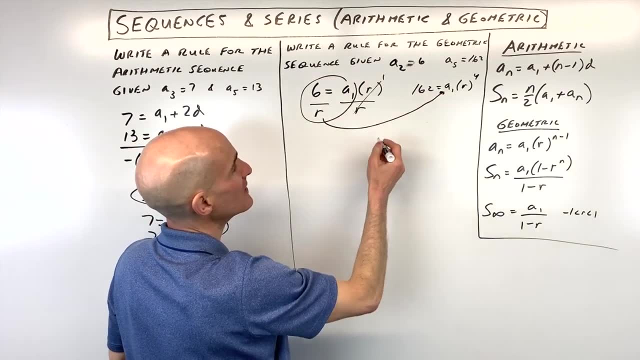 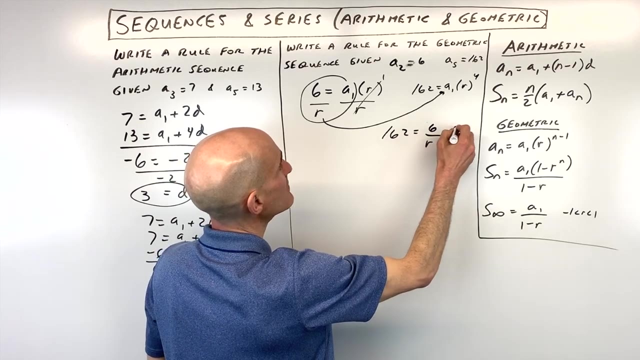 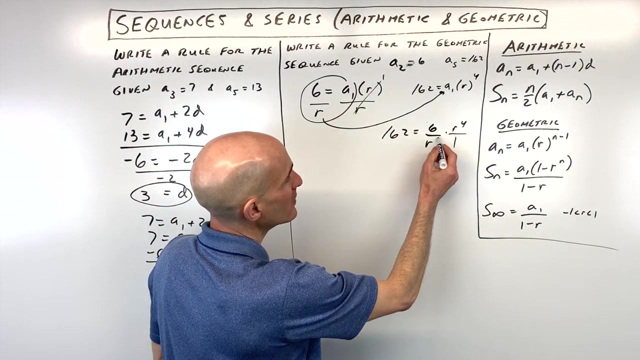 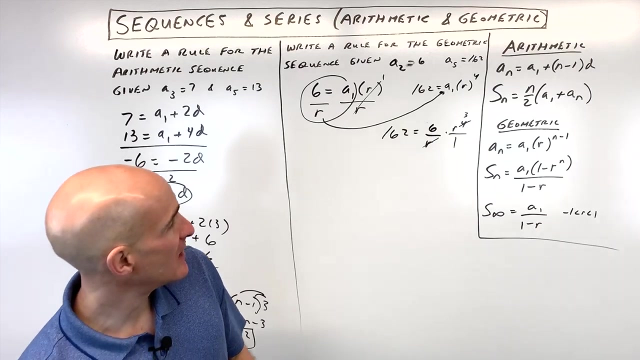 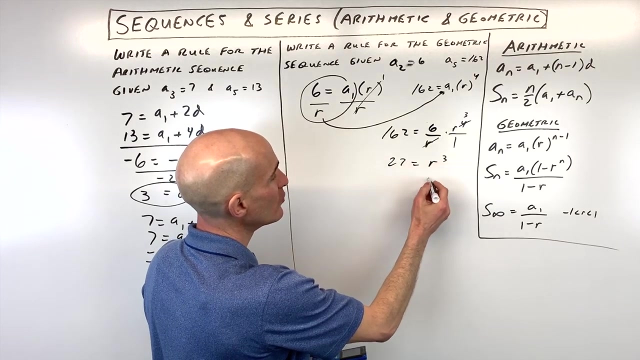 What I'm going to do here is I'm going to divide both sides by r, ok? So now you can see that a1 equals 6 divided by r, we can put that in place of a1 in the second equation, so we have 162 equals 6 divided by r, times r to the 4th. Now this is really like r to the 4th over 1, because anything can be written as a fraction, and we can do some cross reducing. One of these r's cancels with one of these r's, leaving an r cubed. If we divide both sides by 6, let me go to the calculator on that one, that comes out to 27 equals r cubed, take the cube root of both sides, and you can see we're getting r equals 3. 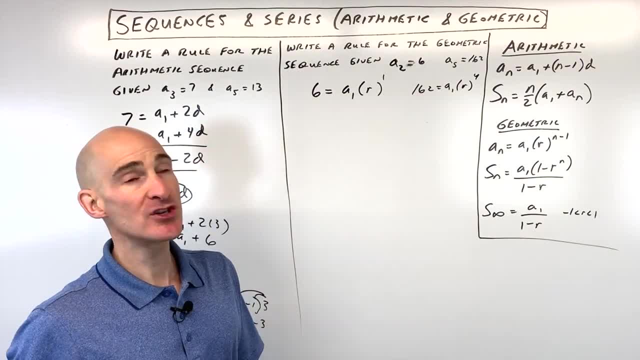 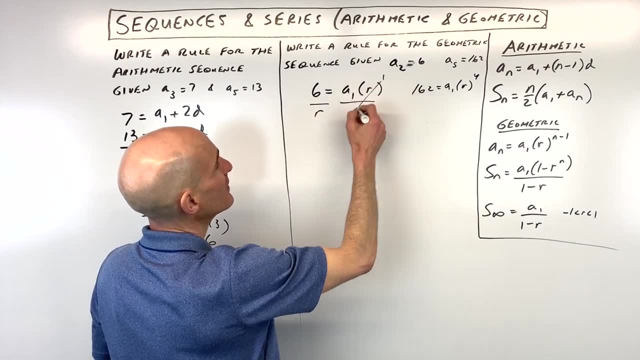 4,. so now we have two variables- the first term and the ratio- and we have two equations. we can solve that system. What I'm going to do here is I'm going to divide both sides by r, ok, So now you can see that a1 equals 6 divided by r. we can put that in place of. 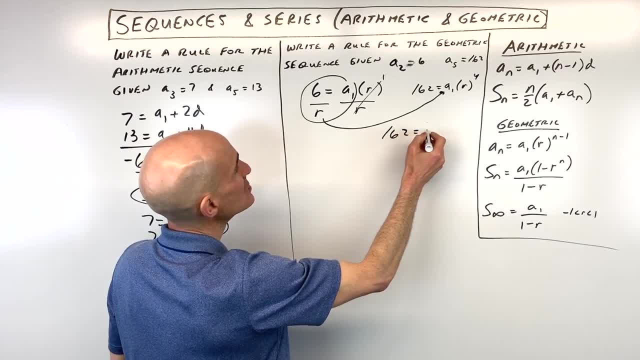 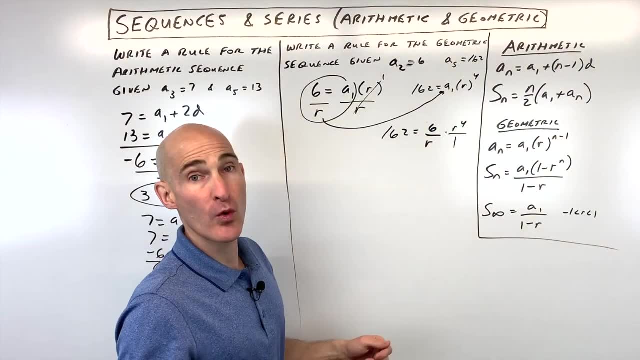 a1 in the second equation. so we have 162 equals 6 divided by r times 162, and that's times r to the fourth. Now this is really like r to the fourth over 1, because anything can be written as a fraction and we can do some cross reducing One of these r's cancels. 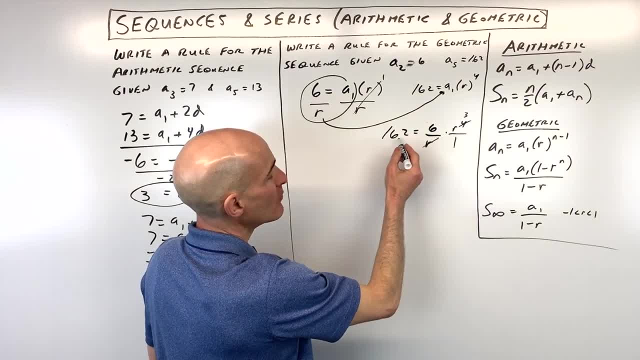 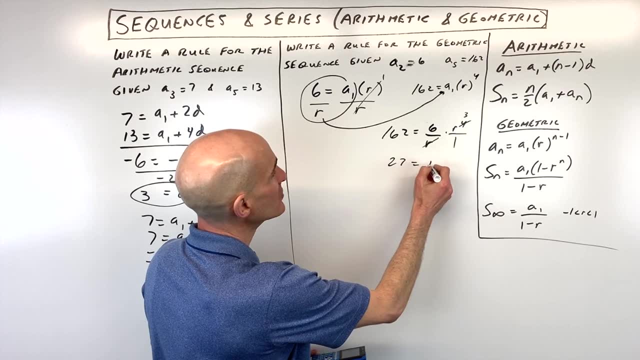 with one of these r's, leaving an r cubed. If we divide both sides by 6, let me go to the calculator on that one that comes out to 27,. equals r cubed. take the cube root of both sides and you can see we're getting r equals 3.. 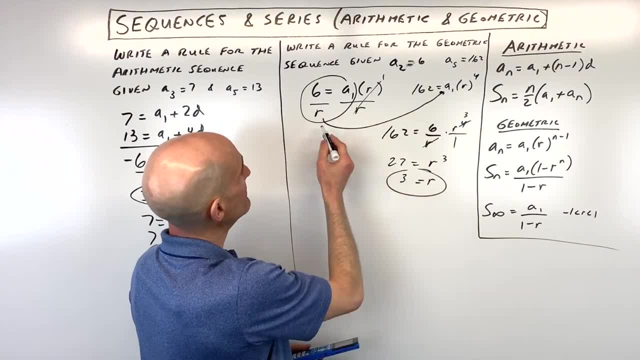 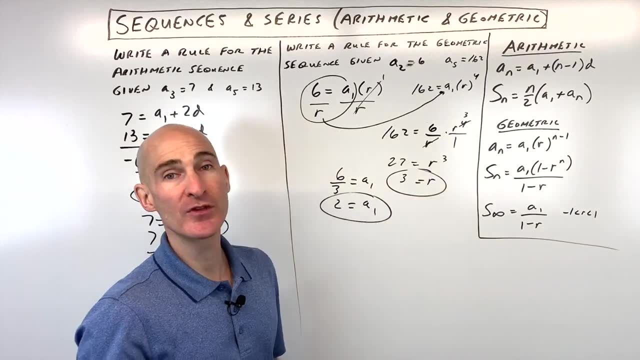 Now, if we put 3 back in to either one of these equations- I'm going to put it over here- we have 6 divided by 6.. 6 divided by 3 equals a1,, a1 equals 2, so we have the first term in the ratio we can. 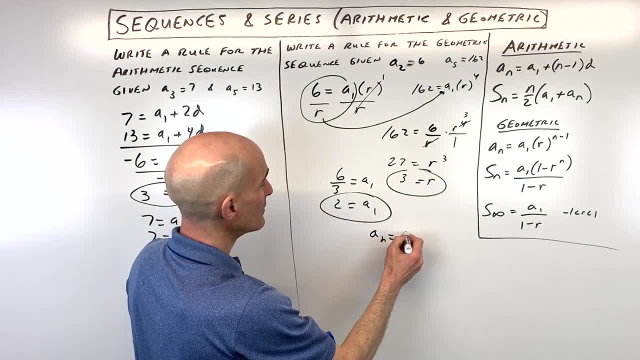 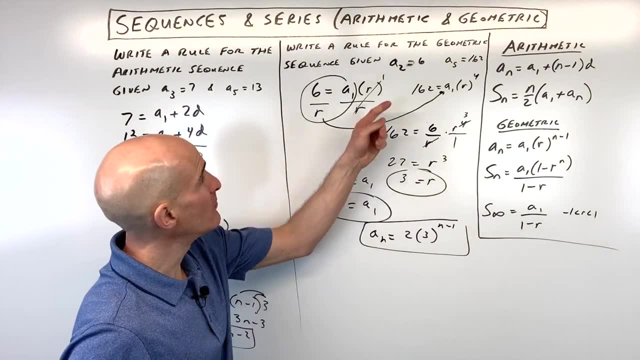 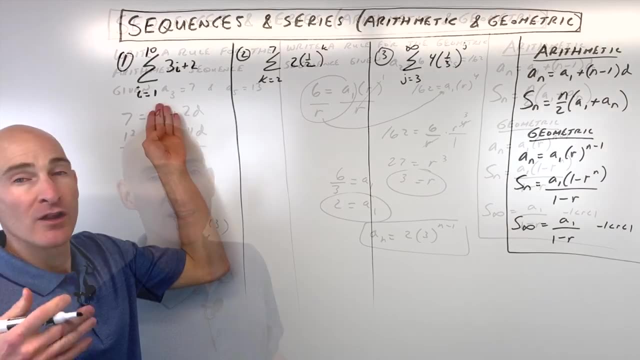 write our rule or our formula for any term in the geometric sequence And if you want to check it out, you can always plug in 2. for example, 2 minus 1 is 1,, 3 to the first is 3, times 2 gives you 6, and same thing with the next term. 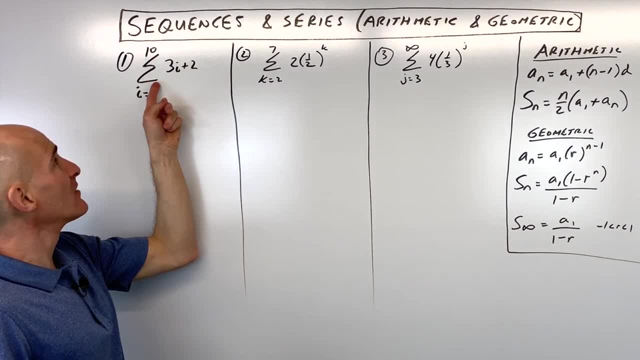 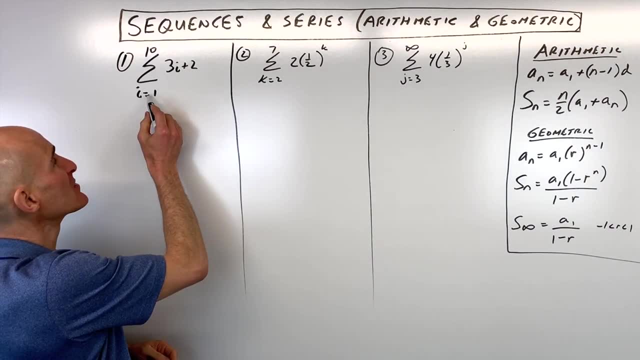 Let's take a look at this summation notation. so see this Greek letter sigma here. it kind of represents the sum and what you do is you take this number here on the bottom- this is called the index- and you would put it in. so if I put 1 in, I get 3 times. 1 is 3,. 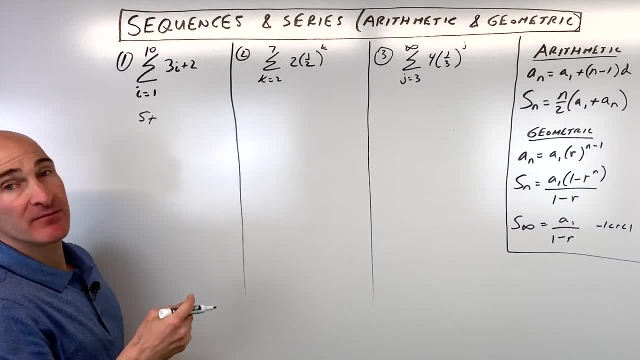 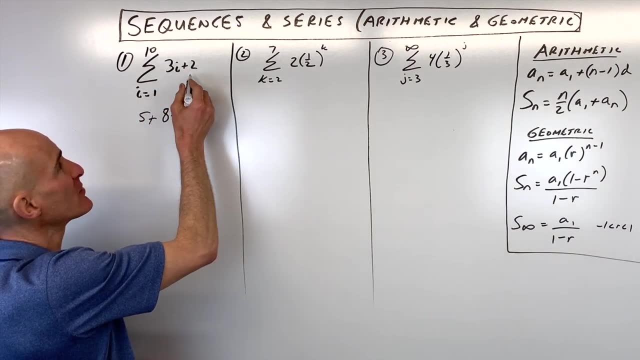 plus 2 is 5,. ok, that's our first term. Now, if I put 2 in 3 times 2, is 6, plus 2 is 8,. if I put 3 in, that's 9 plus 2 is 11,, plus dot, dot dot. you work your way from 1 all. 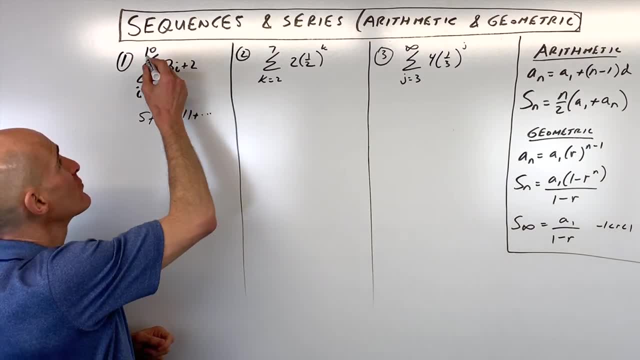 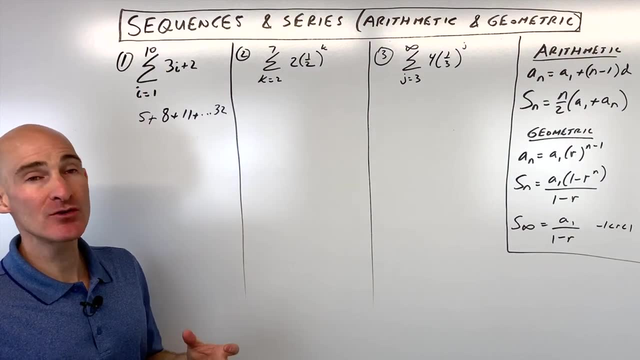 the way up to 10, you know in order, sequentially, like that. So if we put 10 in, we get 30 plus 2, which is 32.. And what the sigma represents again is a sum or a summation, it's a series, and we're adding. 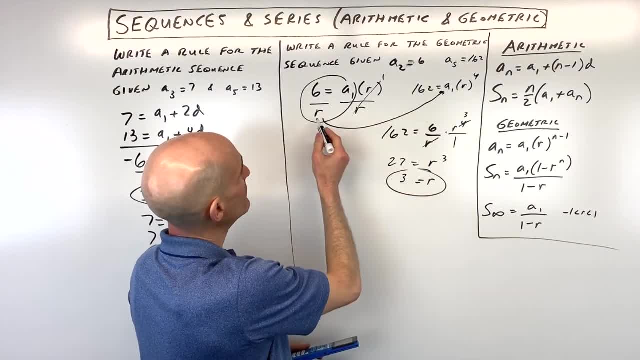 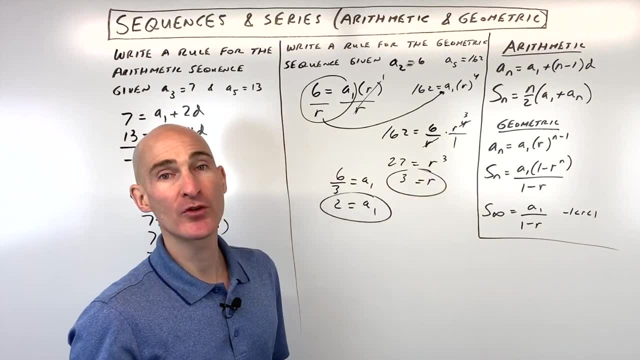 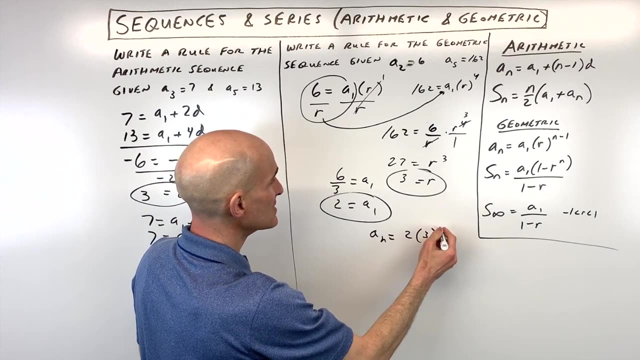 Now if we put 3 back in to either one of these equations, I'm going to put it over here, we have 6 divided by 3 equals a sub 1, a sub 1 equals 2, so we have the first term in the ratio, we can write our rule, or our formula for any term in the geometric sequence. 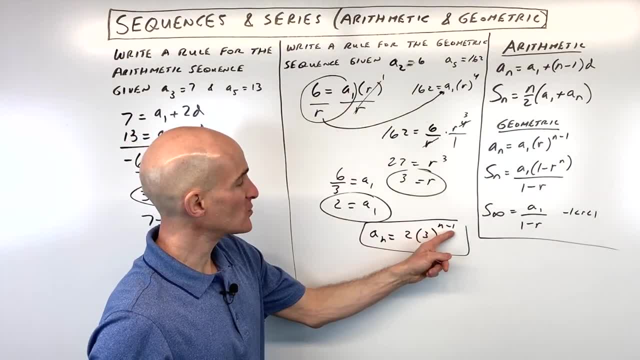 If you want to check it out, you can always plug in 2 for example, 2 minus 1 is 1, 3 to the first is 3, times 2 gives you 6, and same thing with the next term. 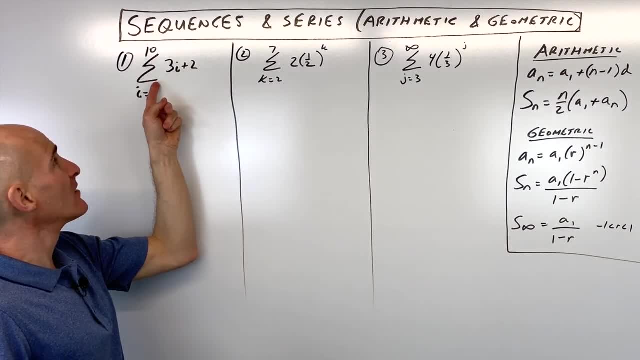 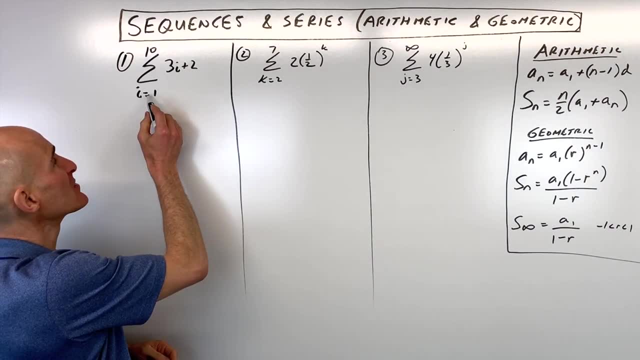 Let's take a look at this summation notation, so see this Greek letter sigma here, kind of looks like an e, that represents the sum, and what you do is you take this number here on the bottom. 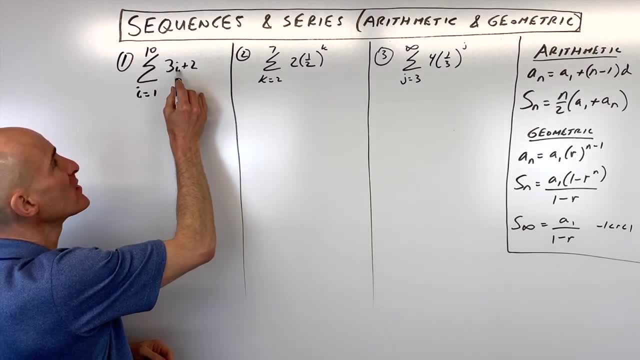 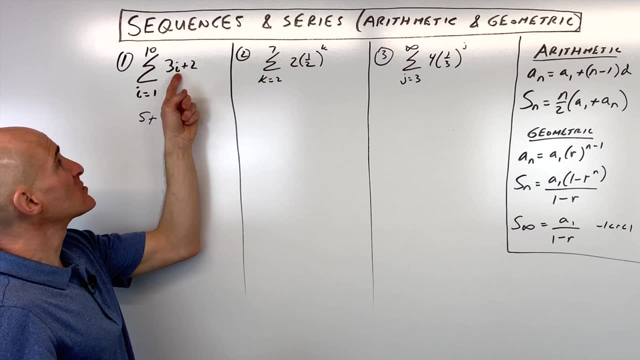 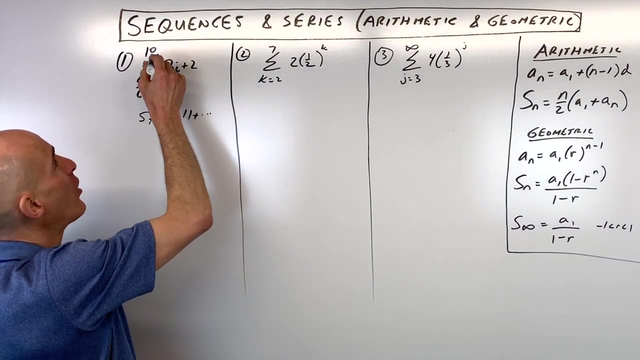 the index, and you would put it in. So if I put 1 in, I get 3 times 1 is 3 plus 2 is 5. Okay, that's our first term. Now if I put 2 in, 3 times 2 is 6 plus 2 is 8. If I put 3 in, that's 9 plus 2 is 11 plus dot dot dot. You work your way from 1 all the way up to 10, you know, in order sequentially 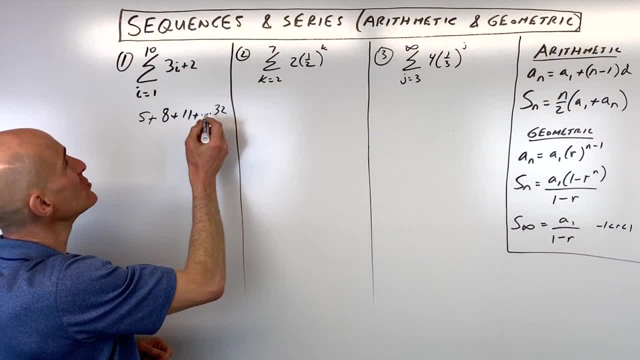 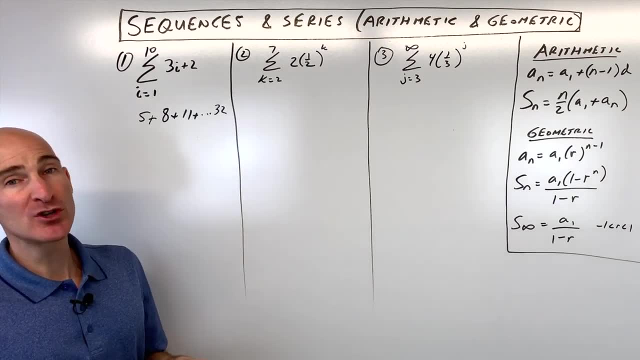 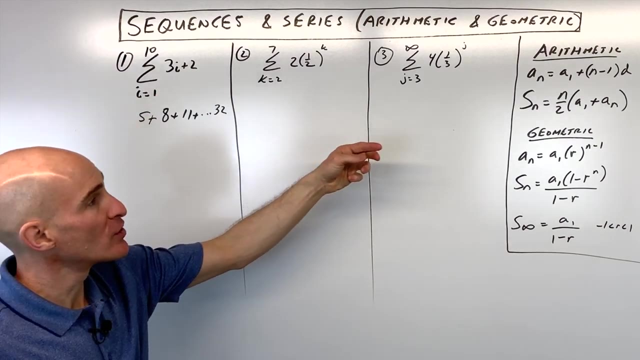 like that. So if we put 10 in, we get 30 plus 2, which is 32. And what the sigma represents, again, is a sum or a summation. It's a series, and we're adding up all these terms. But what you can notice here is that, see how we're adding 3, 3, 3? This is an arithmetic series. So to find this sum, we're going to go over here to our arithmetic series formula. We're going to take n, which is 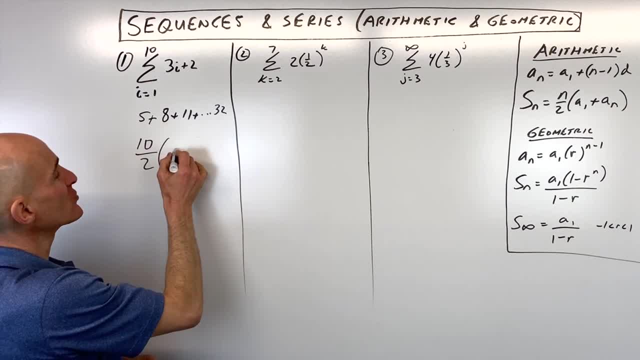 the number of terms, 10, divided by 2. The first term, a sub 1 is 5, plus the last term, which is 32, and we get 5 times 37, which is 150 plus 35 is 185. 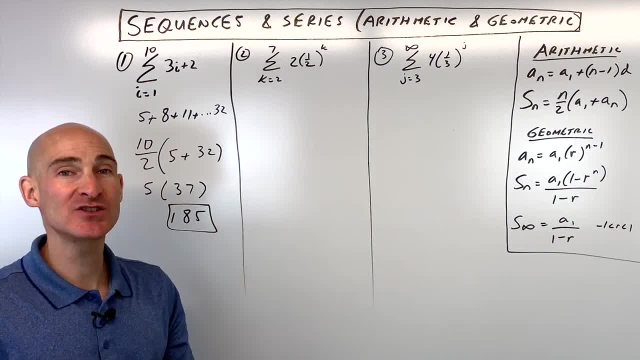 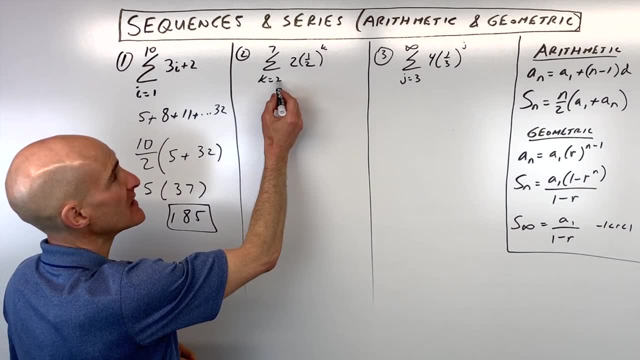 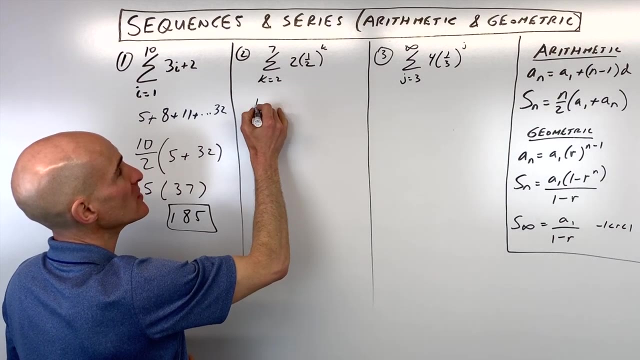 And you've got the sum. So this is kind of like a compact, condensed way of writing a series. Let's look at number 2. So same idea here. You're going to start at the bottom index, your k in this case, and you're going to put 2 in for k. 1 half to the second power is 1 fourth times 2 is 1 half. 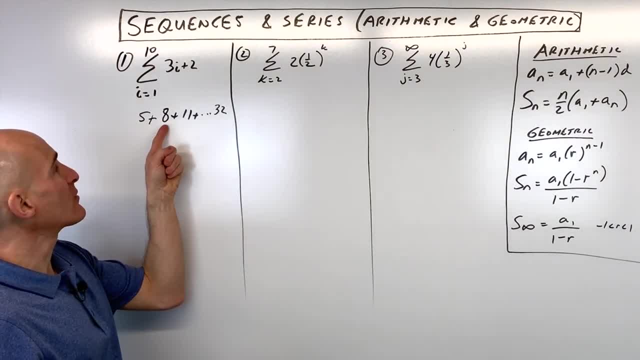 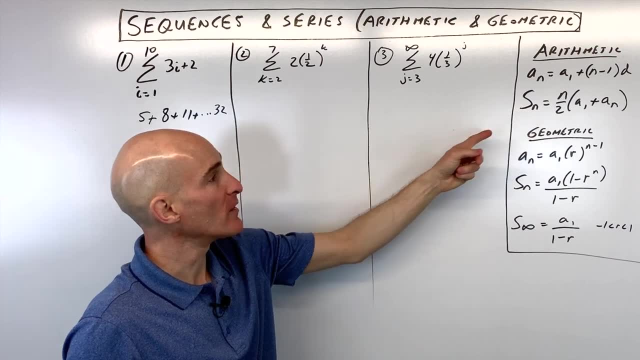 up all these terms. But what you can notice here is that see how we're adding 3,, 3,, 3? This is an arithmetic series. so to find this sum, we're going to go over here to our arithmetic series formula. we're going to take n, which is the number of terms, 10, divided by 2,. 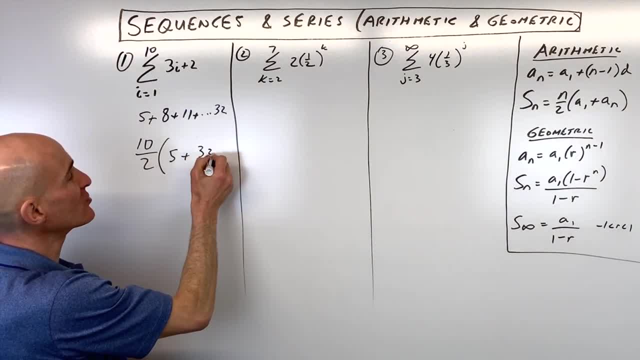 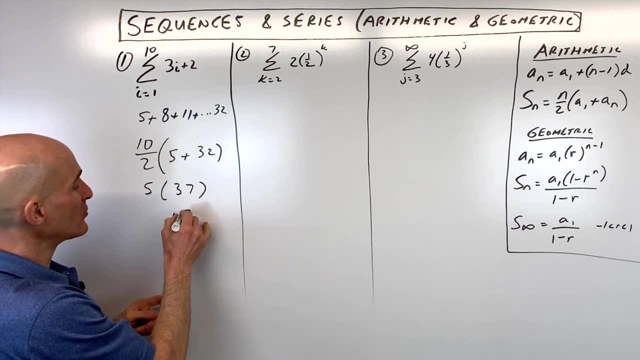 the first term, a sub 1, is 5,, plus the last term, which is 32,, and we get 5 times 37,, which is 150 plus 32.. 35 is 185, and you've got the sum. 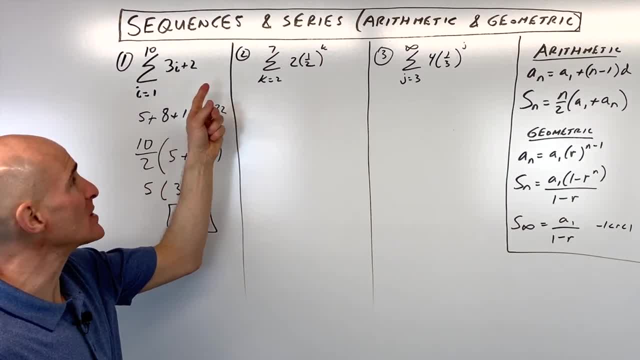 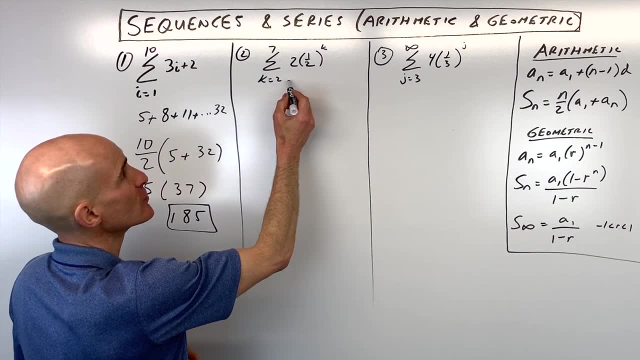 So this is kind of like a compact, condensed way of writing a series. Let's look at number 2.. So same idea here. you're going to start at the bottom index here- k in this case- and you're going to put 2 in for k. 1 half to the second power is 1. fourth times 2 is 1. 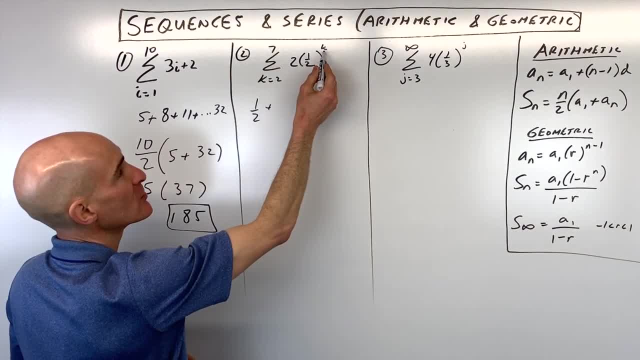 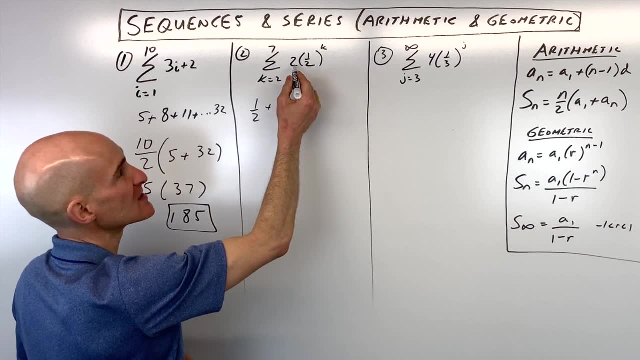 half. Say, for example: we put the next one in 3, we get 1 half cubed, which is 1 eighth times 2, which is 1. fourth Say, we put in 4.. We get 1 half to the fourth. power is 1. sixteenth times 2 is 1. eighth dot, dot dot, right until. 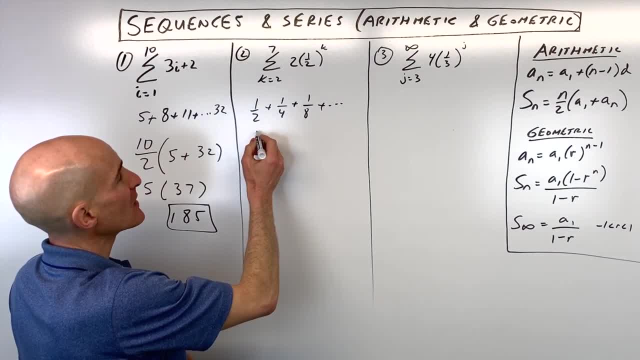 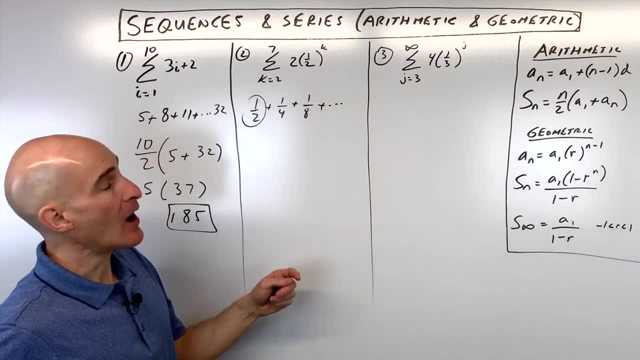 you get to the seventh term. So here, what you can see is that we're multiplying by a half each time, and we can see that the first term is 1 half, and now all we have to do is figure out how many terms are there. 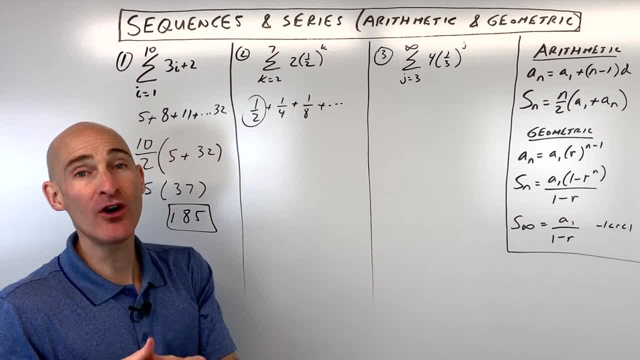 from 2 to 7.. Now a lot of people mistakenly will look at this top number and say, oh, Mario, it's 7.. That's not quite right, because we didn't start at 1,, we started at 2, and another mistake. 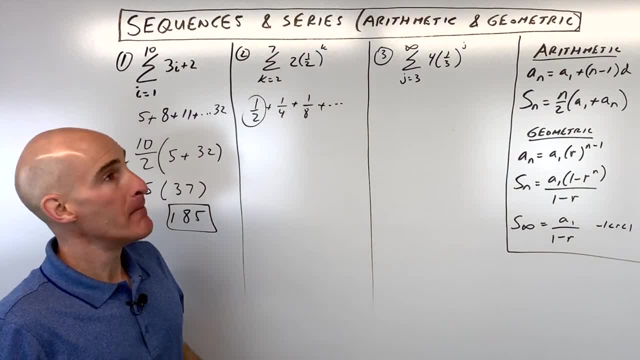 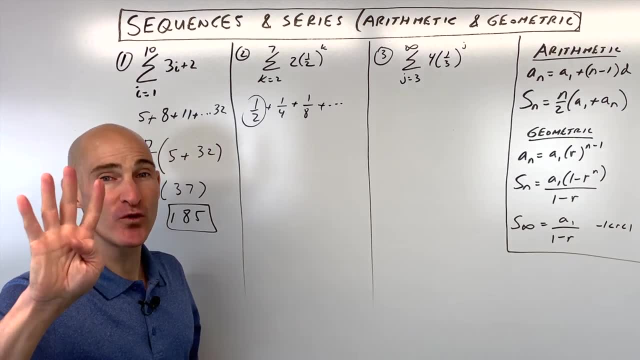 students make is they say: well, oh, Mario, it's 7.. Oh, 7 minus 2 is 5, but there's actually 6 terms here, because think about it, if somebody says how many numbers are there, from 1 to 5,, 5 minus 1 is 4, but really you can see. 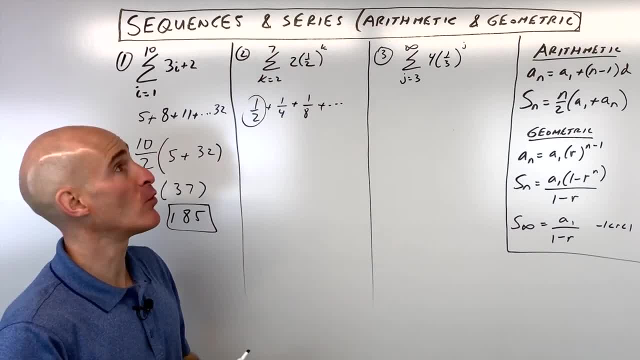 there's 5 terms. So when you're counting the first and the last, when you subtract you have to add one more. So 7 minus 2 is 5, plus 1 more is 6.. We have 6 terms. 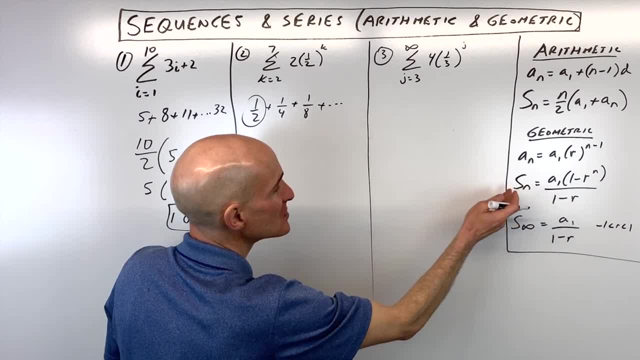 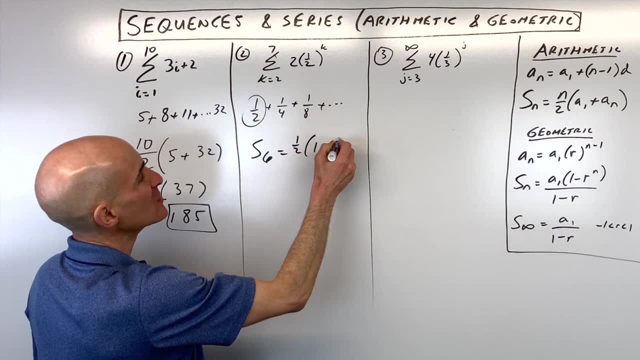 We know it's geometric because we're multiplying by a half, so we're going to use this formula right here. So the sum of these 6 terms- The first term we said- was 1 half, The ratio, which was 1 half, there was 6 terms all divided by 1 minus 1 half. 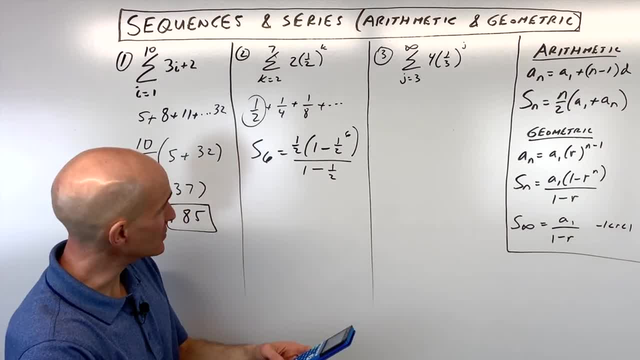 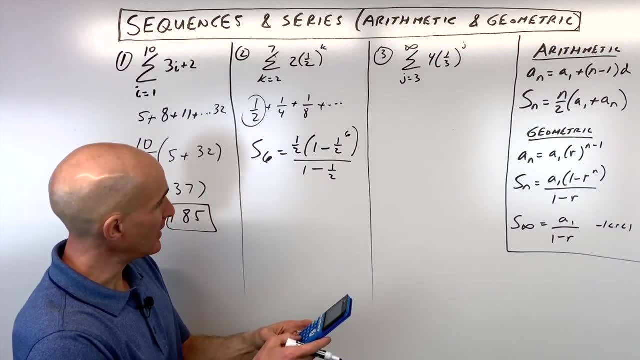 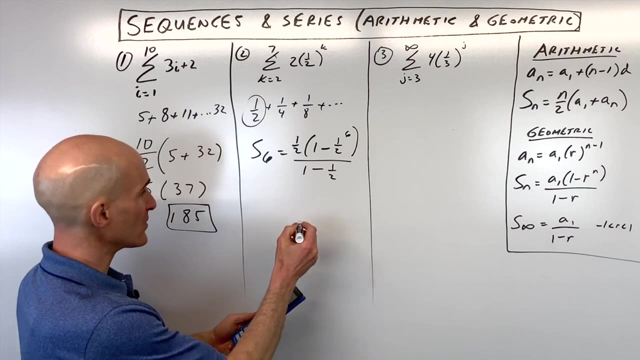 So let's go to the calculator on this one and let's see what we get. So we have 1 minus OK, all divided by, and I'm getting. let's see if I can convert that to a fraction here: for us it's 63 64ths. 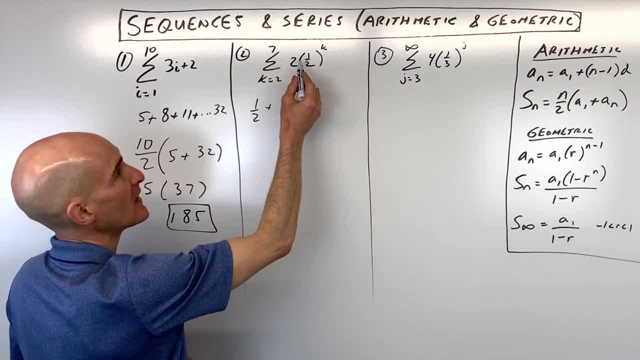 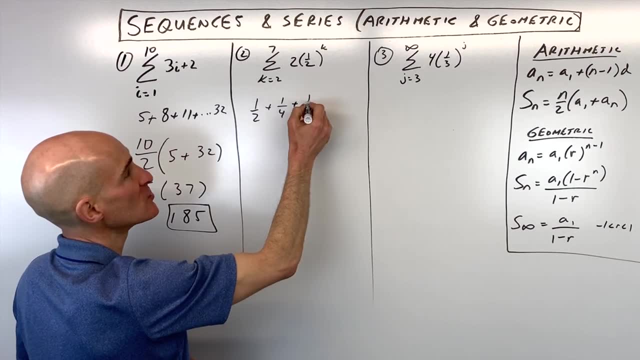 Say, for example, we put the next one in 3. We get 1 half cubed, which is 1 eighth, times 2, which is 1 fourth. Say we put in 4. We get 1 half to the fourth power is 1 sixteenth times 2, which is 1 eighth, dot, dot, dot, right, until you get to the seventh term, okay? So here, what you can see is 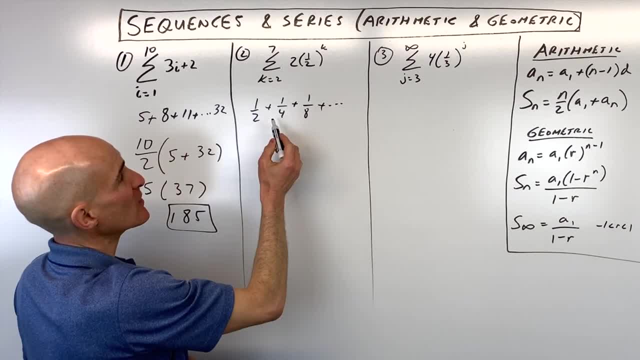 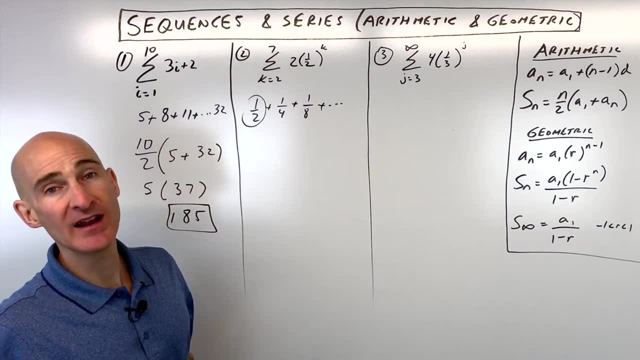 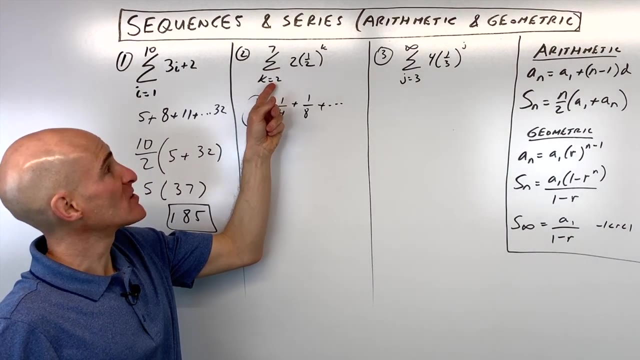 that we're multiplying by a half each time, and we can see that the first term is 1 half, and now all we have to do is figure out how many terms are there from 2 to 7. Now, a lot of people mistakenly will look at this top number and say, oh, you know, Mario, it's 7. That's not quite right, because we didn't start at 1. We started at 2. Another mistake students make is they say, well, oh, 7 minus 2 is 5. But, 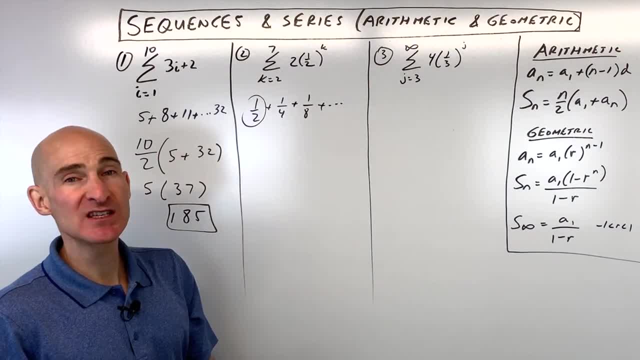 there's actually 6 terms here, because think about it. If somebody says, how many numbers are there from 1 to 5? 5 minus 1 is 4, but really, you can see there's 5 terms. So when you're counting the first and the last, when you 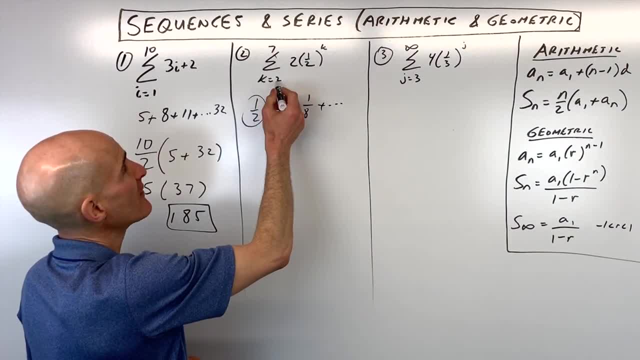 subtract, you have to add 1 more. So 7 minus 2 is 5, plus 1 more is 6. We have 6 terms. 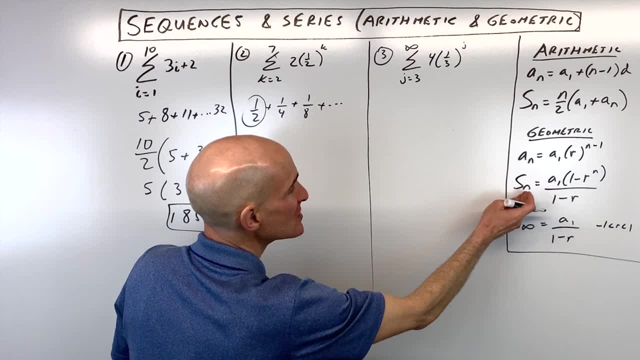 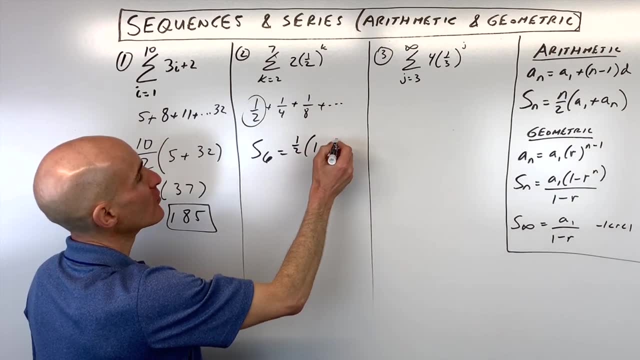 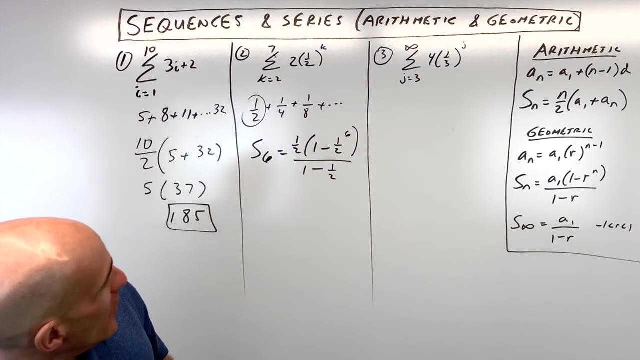 We know it's geometric, because we're multiplying by a half, so we're going to use this formula right here. So the sum of these 6 terms, the first term we said was 1 half, the ratio, which was 1 half, there was 6 terms, all divided by 1 minus 1 half. So let's go to the calculator on this one, 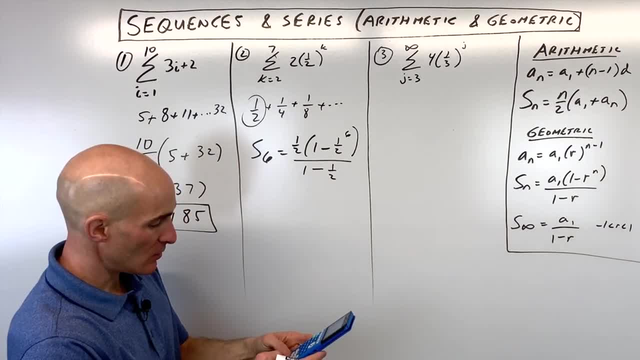 and let's see what we get. So we have 1 minus, okay, all divided by, and I'm getting, 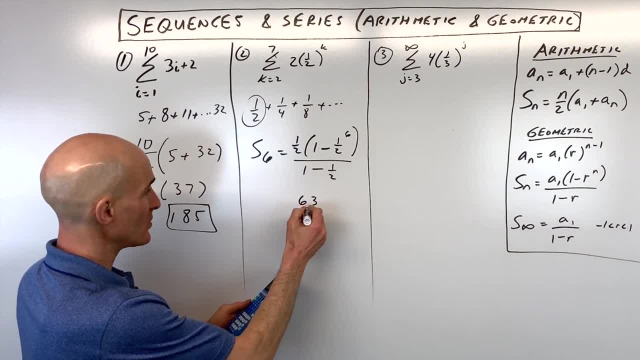 let's see if I can convert that to a fraction here for us. It's 63 64ths. 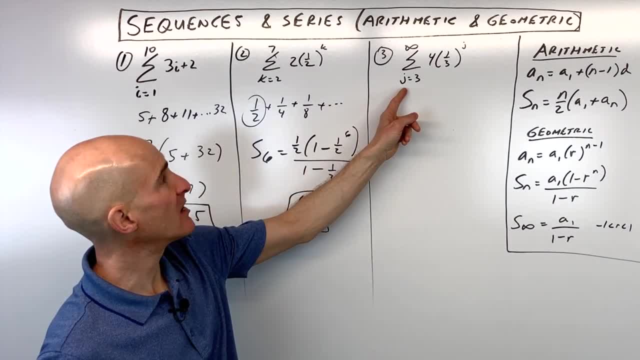 Okay, let's look at number 3 now. This one, you can see that it's an infinite number.